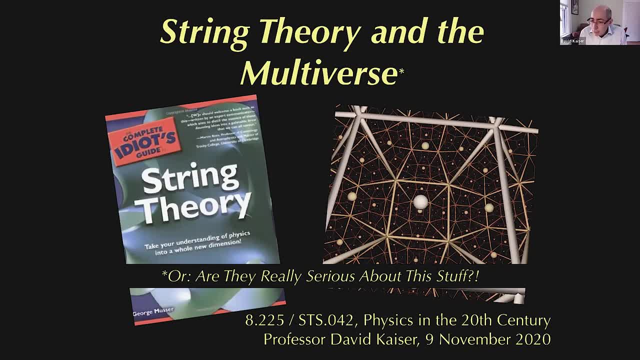 described in popular culture. There are ideas that are still clearly speculative. These are not proven by any possible measure, but they are, at least to some members of the community, well-motivated. There's reasons why lots of people think about these things and take 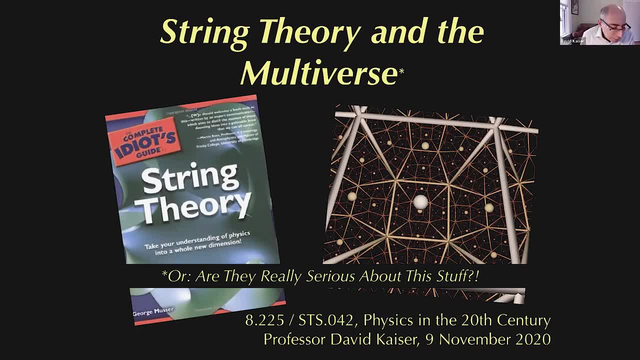 them seriously, even though we, the community, certainly don't have any kind of consensus yet, let alone a lot of kind of reliable empirical or observational information to help us sift through competing ideas. So we're in this kind of awkward state where lots of folks are pursuing interesting and sometimes very strange-sounding questions. 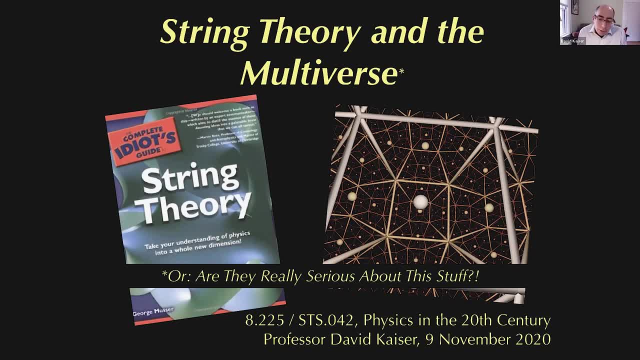 and suddenly they get actually stranger and stranger-sounding, I think, And so I wanted to kind of end our semester this term with this kind of taste of some small set of the open questions that members of the community are still really wrestling with and grappling. 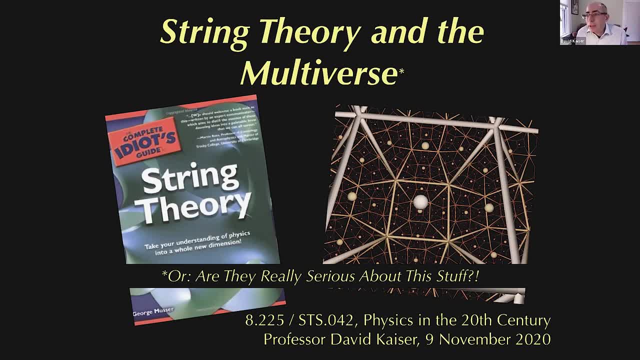 with today. So I'll focus on ideas about string theory, some ideas about string theory and the multiverse, And there's lots and lots and lots written about this, often for a non-technical audience, And part of also what I wanted to do with this class was just give you some pointers. 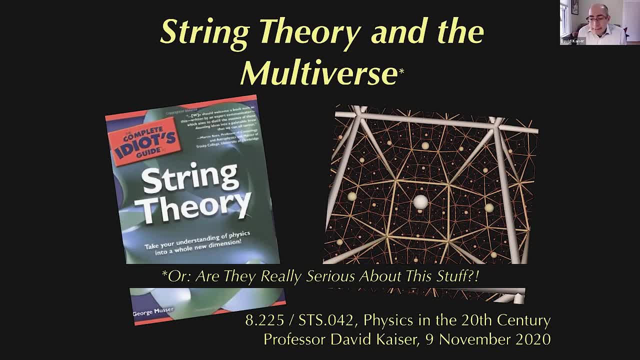 for some books that I really like, some accessible, really very well-written popular books by physicists with a range of opinions about this stuff, And so some of them are written by kind of arch rivals conceptually and they together, I think, can help us get a reasonable. 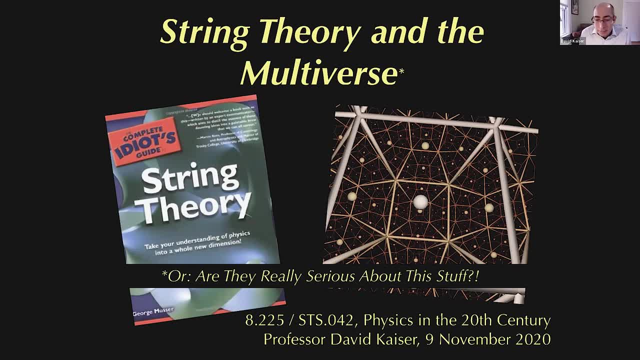 sense of at least what seems to be at stake. What are some of our colleagues so exercised about, and why do they have competing visions for kind of next-generation, next-generation, next-generation- big steps forward on this intellectual journey? we've been kind of marching along together this. 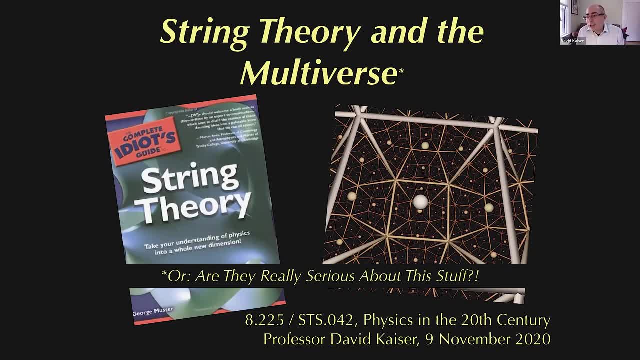 term. Not all of it is in the Complete Idiot's Guide, though I do actually like this book by my colleague George Musser. He's an award-winning science writer and a PhD in astrophysics. He actually is himself not an idiot, but he wrote this fun book for the Complete Idiot's Guide. 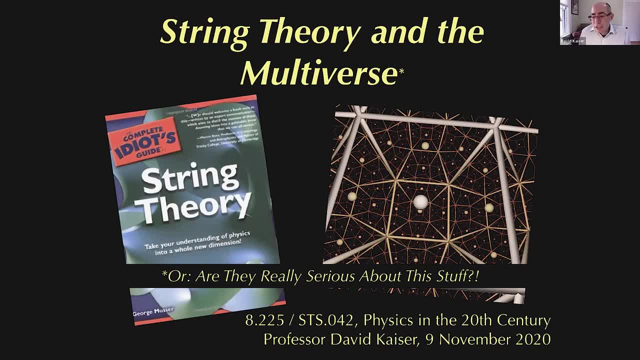 series on string theory and, of course, other books as well. So partly what I'll do with these slides is give little shout-outs with some book covers for some of these books that I enjoy. you might be interested in reading after the dust has settled on this crazy semester, if you're looking for some. 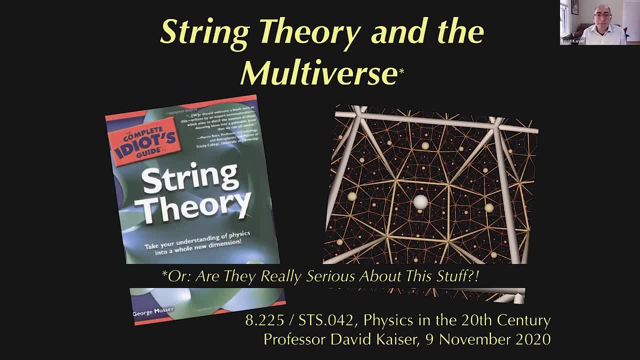 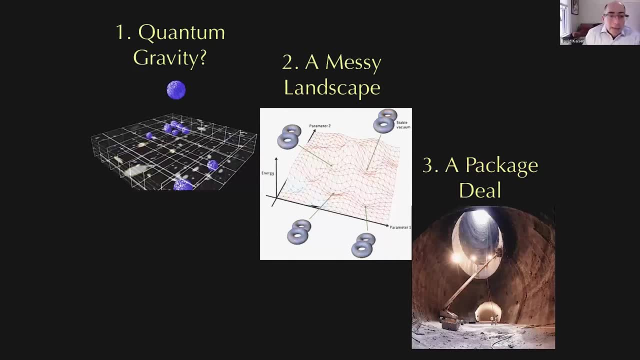 virtual beach reading for IAP. These might be of interest. So, as usual, of course, three main parts for the discussion today. I want to turn the clock back and look at this really hundred-year-long quest, a hundred-year-long challenge to try to find a quantum mechanical description of gravity. 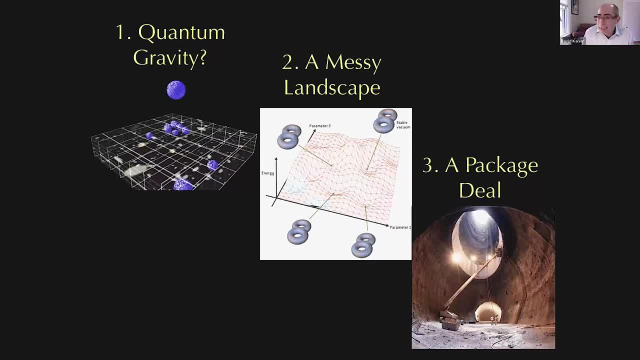 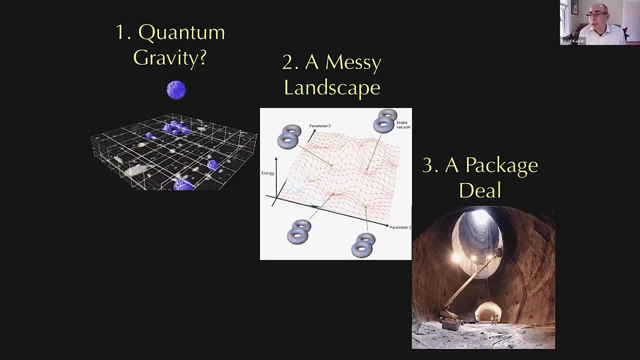 and why has this approach taken such a different turn compared to other efforts to describe fundamental forces of nature, quantum mechanically. So we'll look at, in some sense, where string theory comes from and why some people have been so excited about it compared to other approaches. 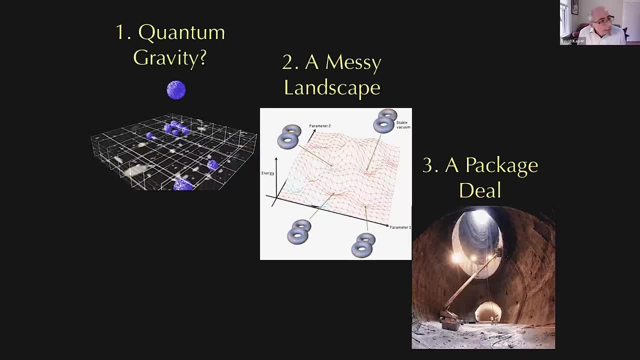 Then in the second part we'll look again just very briefly at some of the kind of collisions, some of the possible implications of thinking about these string theory ideas in the context of cosmology getting a little closer to work that I've been involved with or some of my colleagues have been more involved with. 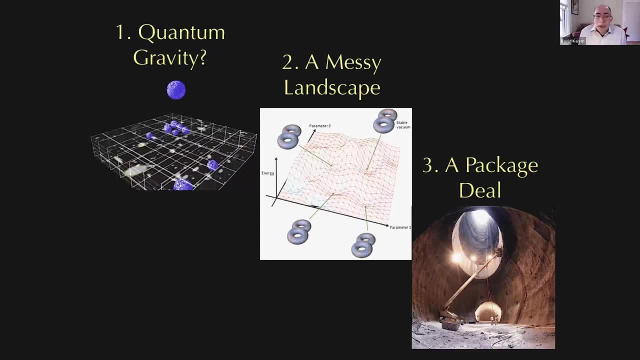 So when we take this kind of particle cosmology view and take on board or try to take seriously some of the ideas or possible implications of the high energy theory part, the string theory part, what does that lead us- at least lead some people- to wonder about in this more cosmological setting? 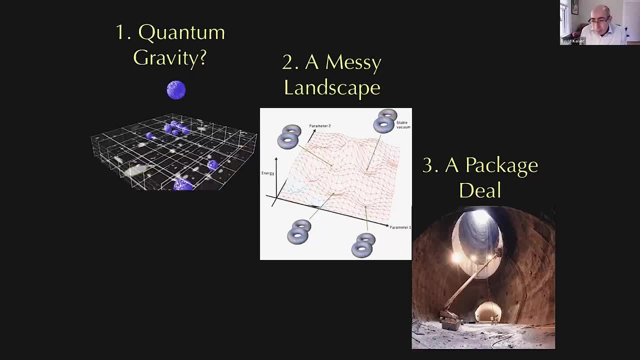 That's part two And then part three. just very briefly, we'll zoom out and again remind ourselves that, like all the work we've looked at together over this entire semester, none of these ideas are kind of unfolding in a vacuum that I think we can make sense of some of. 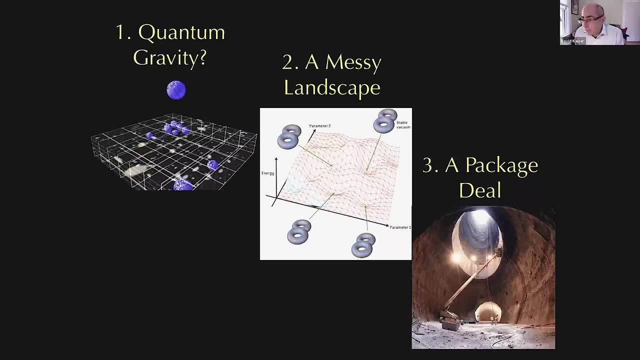 the rhythms of change, if not the particular ideas that come forward by asking about who's doing this work, in what settings and what's- some elements of a larger context that might help us make sense of the of the twists and turns. Okay, so, as I mentioned, this century-long challenge, 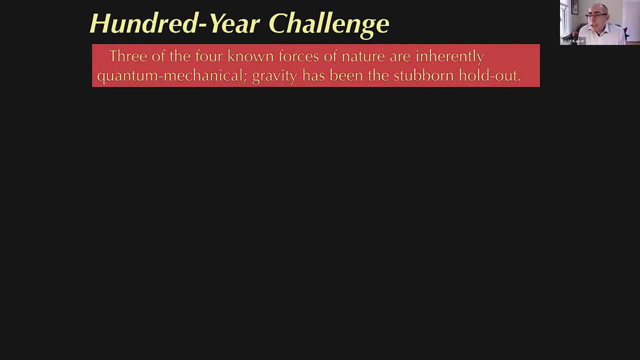 a kind of grand challenge for the field has been to find some internally self-consistent description of gravity in the kind of framework of quantum theory. We've seen, at least in some we looked at in some detail, others we had kind of hints at that- over the mostly second half of the 20th century especially. 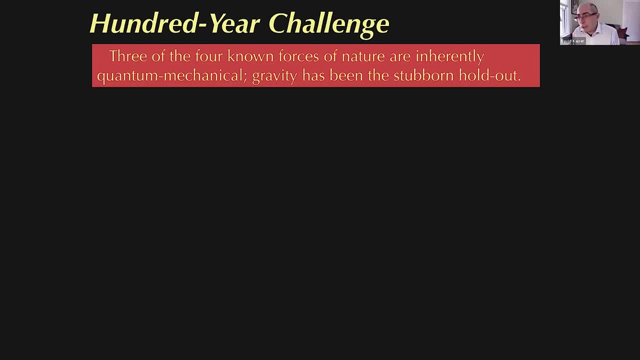 each of the other three main known physical forces of nature- electromagnetism, the strong nuclear force and the weak nuclear force- each of those has been given a quantitative treatment in terms of quantum theory, in terms in particular of quantum field theory. We looked a 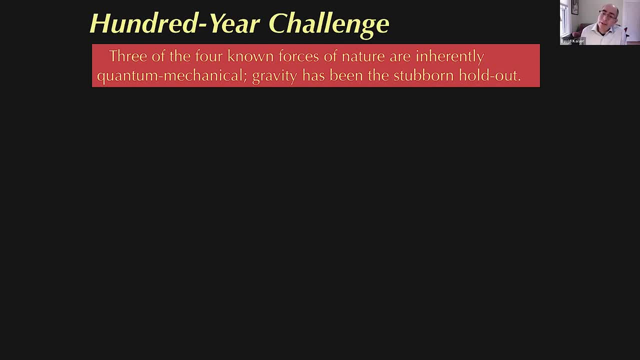 lot at quantum electrodynamics, the quantum mechanical version of electromagnetism, associated with people like Tomonaga and Julian Schwinger and Feynman and others. Likewise, we look briefly at quantum chromodynamics. There's been this sort of remarkable success. 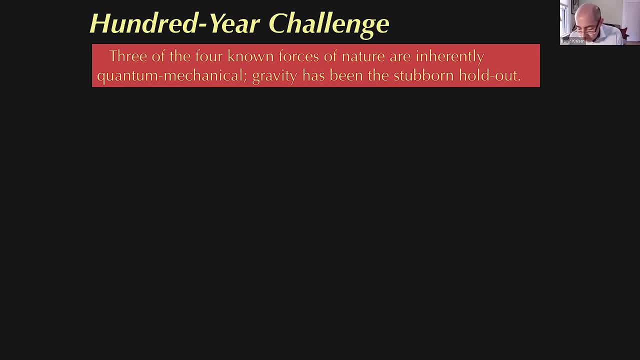 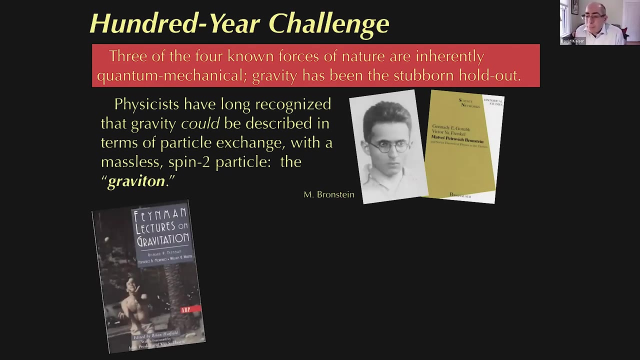 often in very close dialogue between experimental inputs and theoretical advances, And yet gravity, the fourth known force of nature, has been this stubborn holdout, Turns out. this has been going on for a long, long time. One of the earliest people to try to build a quantum theory of gravity is 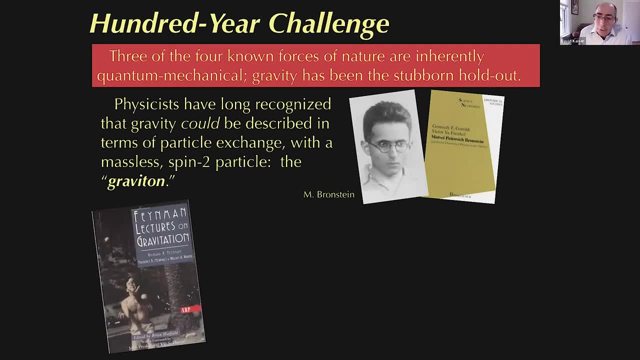 this young person shown here, Matvei Bronstein, who was working in the Soviet Union in the mid-1930s. He was quite young. as you can see in the photo. Bronstein was writing papers mostly in Russian in some of the Russian journals, a few of them in German, not very well known outside of his 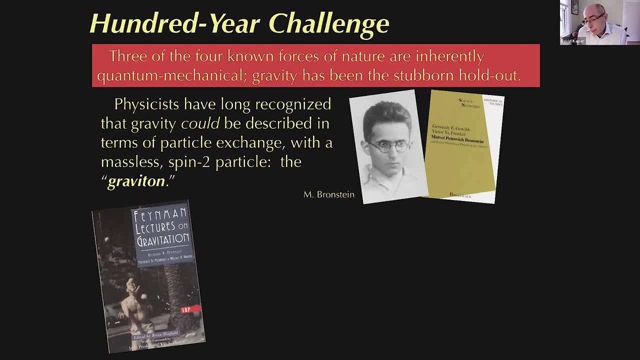 immediate circle at the time. But he was doing what in hindsight we see was really pretty advanced stuff and that has held up, I think, quite well over time, Where he recognized that if one tried to make a quantum mechanical treatment of Einstein's general theory of relativity, the reigning description of gravity, 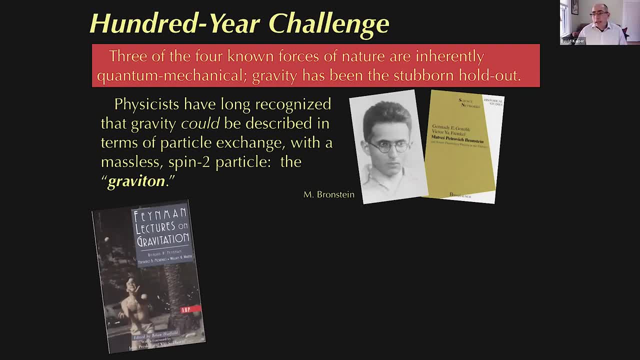 then you could try to formulate it on a model of exchange of virtual particles. The virtual particles in this case would have a little more complicated mathematical structure. That might not surprise us, given how much we saw even Einstein's own version of general. 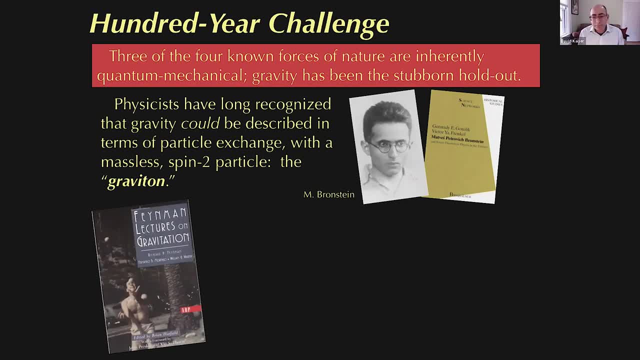 relativity was so mathematically involved with warping spacetime. Bronstein showed that you could actually reproduce the basic structure of general relativity as arising from the exchange of a certain kind of particle, a certain kind of force-carrying particle. 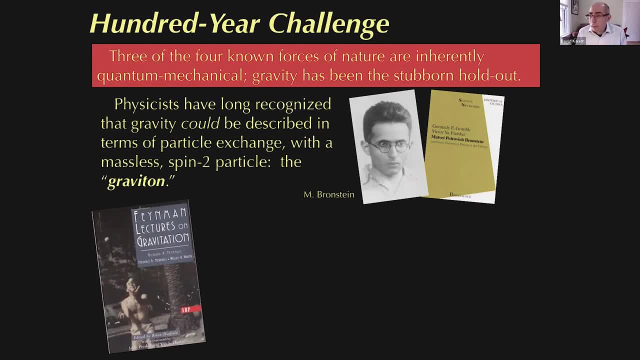 Instead of the photon being the force-carrying particle for a quantum mechanical version of electromagnetism, for quantum electrodynamics, there would be a hypothetical graviton, a particle force carrier for gravity, And it would be kind of analogous to the photon. It would be. 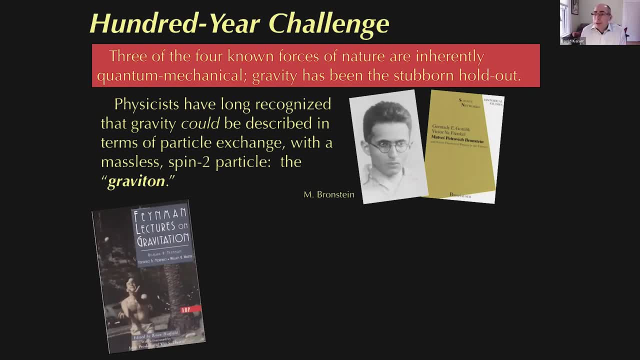 for example, a particle that would have zero mass, just as the photon has zero mass, but it would have two units of spin, whereas the photon has one unit of spin. and most ordinary matter has half integer unit of spin, like electrons and quarks, or even protons and neutrons. 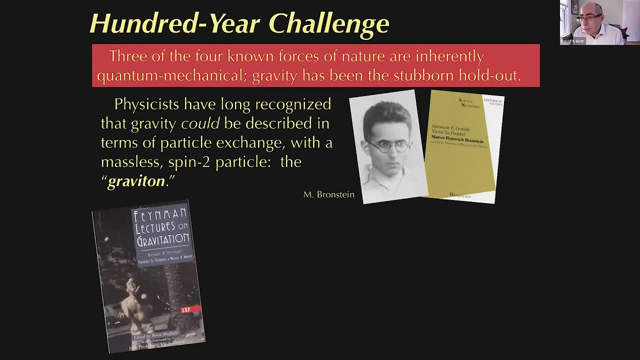 So one could try to reformulate Einstein's version of gravity as arising from the exchange of a particular kind of force-carrying particle, a massless spin-2 particle dubbed the graviton. That was done mostly in obscurity and quite tragically. Bronstein's theory of gravity, which 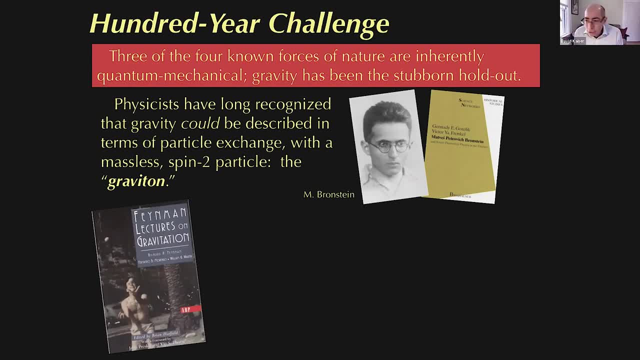 in fact is a very interesting one, is that when he was murdered about a year later, he never had a chance to explore this or, frankly, anything else. he fell afoul, as many, many people did, of Stalin's. 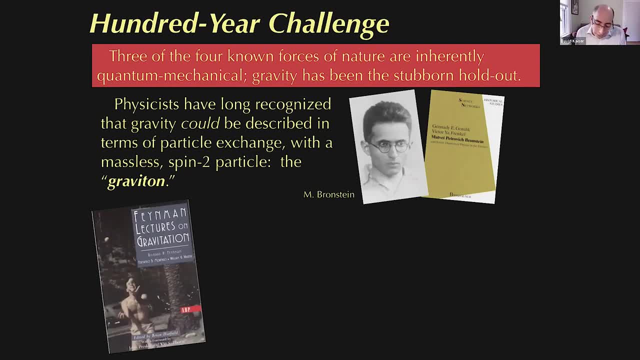 Joseph Stalin's purges in the Soviet Union. He had some political ideas that suddenly put him on the outs with the reigning authorities and he was rounded up, found guilty on a kind of so-called show trial and executed the very same day. There's no chance for an appeal. 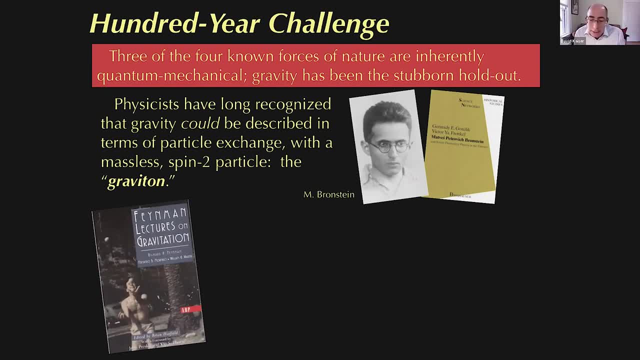 His quest in many ways ended tragically, tragically early. many, many years later Other colleagues, including many in Western Europe and North America, kind of rediscovered insights that Bronstein had put together way back in the 1930s, Much more famously. 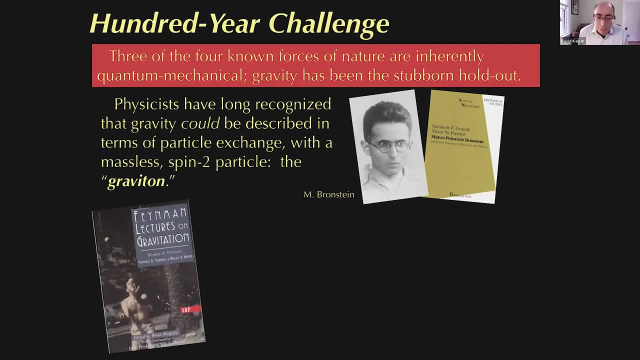 much, much better known, especially in the US and Europe. Richard Feynman, followed along very similar kind of thought paths in the early 1960s, when he himself got interested in gravity, not only particle physics, And Feynman also. in fact he gave these now-famous lectures that were 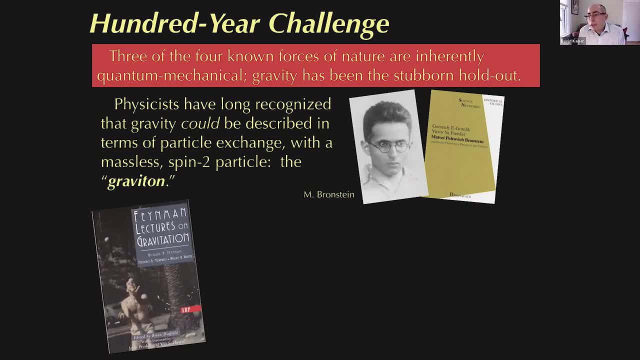 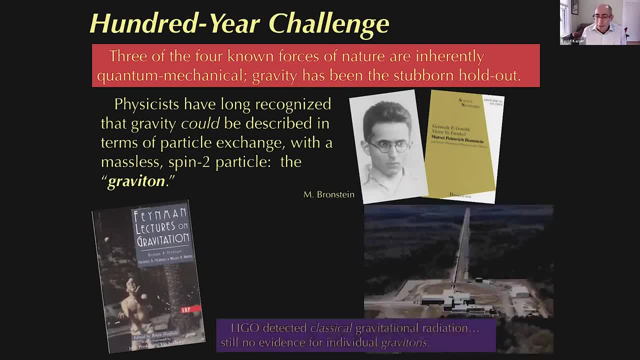 of these particular kinds of force-carrying particles, just classically. Now you might be saying: well, don't we already know that gravitons exist, After all? our very good friends at LIGO have found gravitational radiation. They certainly have using these. 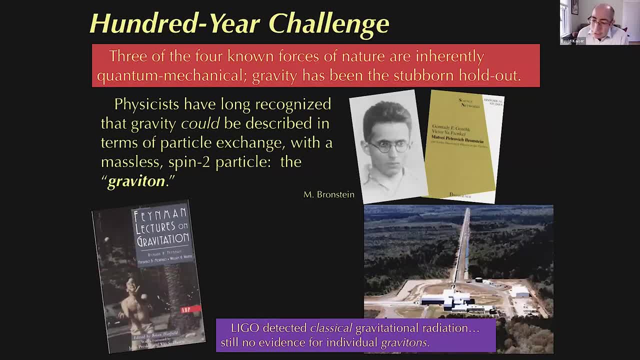 enormous detectors in Hanford, Washington, in Louisiana, now similar devices throughout Europe and others under construction elsewhere. But this is really finding classical gravitational radiations, not identifying individual gravitons. It's like the difference between finding classical Maxwell waves like radio waves, electromagnetic waves that are continuous and classical and extended. 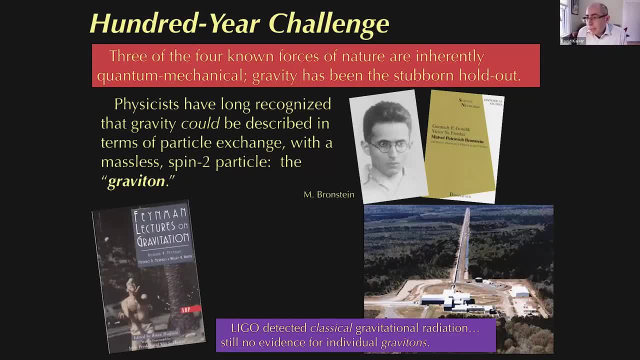 through space and time. It's the same, it's a similar gulf between that and finding evidence of individual photons, individual quantized force, carriers of a quantum mechanical force. So, whereas now we have, thank goodness, really quite compelling evidence about classical extended wave-like, 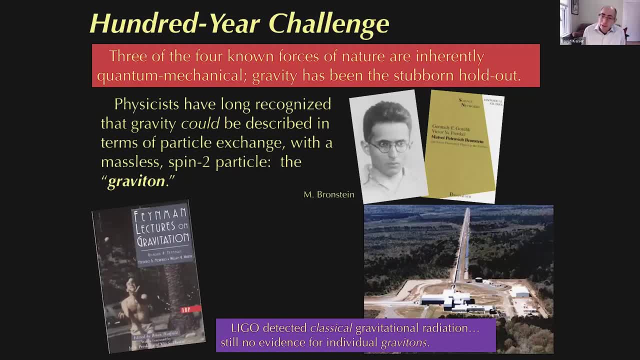 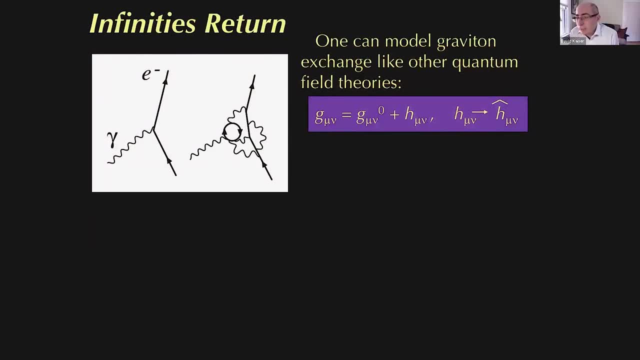 features from gravity. this still is not evidence of individual gravitons. The challenge on that score is still elusive Now. even though there's not compelling experimental inputs about the behavior of gravitons, one could still- and people have over the century- try to build a kind of 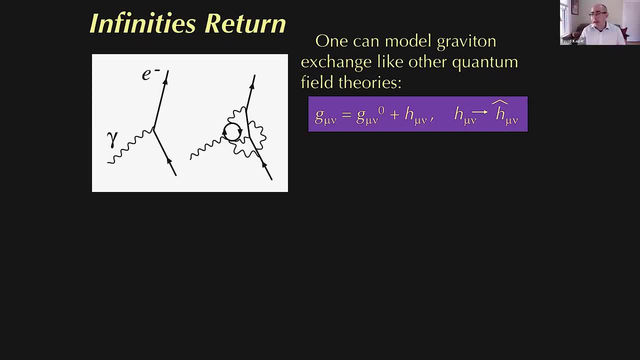 quantum mechanical treatment of these hypothetical force carriers as gravitons, massless spin-2 particles. and that's the kind of work that Bronstein began all the way back in the mid-1930s and people like Feynman and many of his students tried to do. 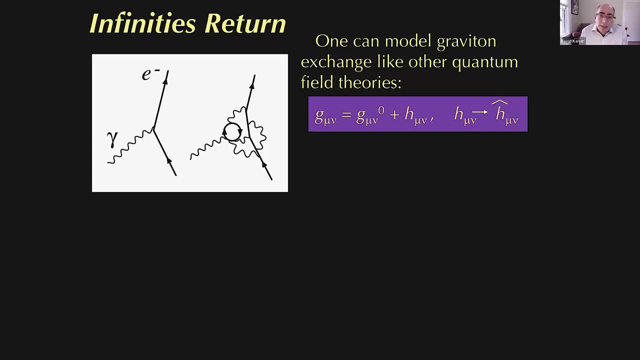 head-on throughout the 1960s and so on. So you can basically say there's a kind of gravitational field, a kind of warping space-time of the sort that Einstein had described. You can imagine the kind of little perturbations around some average value. You can try to treat that as some quantum. 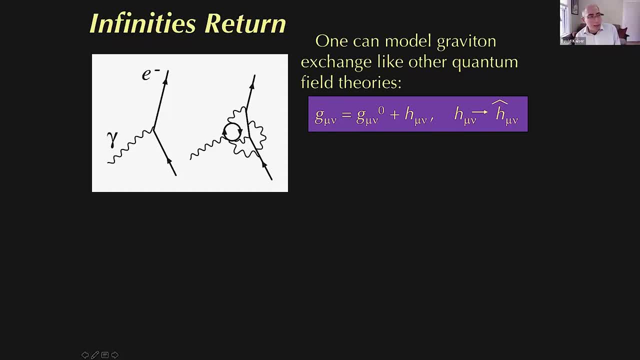 mechanical object, all in direct analogy to the treatment of, say, the Maxwell field as composed of photons. But unfortunately, as people like Bronstein were finding early on, this does not lead to a clear way forward. This approach leads to infinities when you try to account quantitatively. 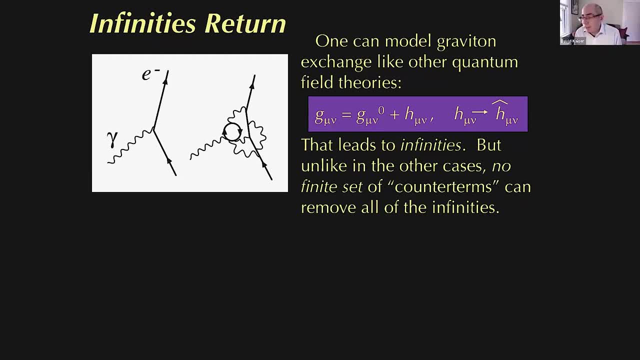 for the behavior of virtual gravitons, much as one would do, say, the exchange of virtual photons. But unlike the case of QED or, as people now know, even unlike the case of quantum chromodynamics and the others, there's no way to get rid of or to kind of self-consistently absorb these infinities. 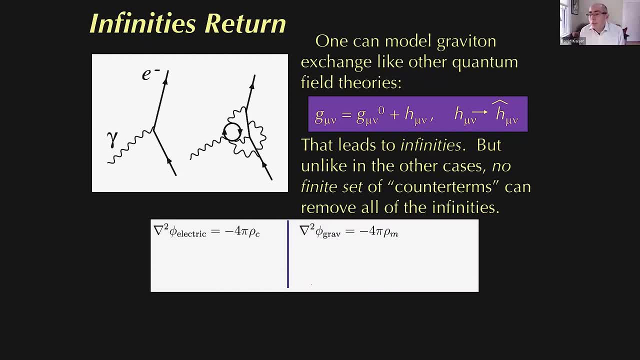 And we can get a sense for that by going all the way back to one of the very first lectures this term. Classically, we can get a sense at least for why there might be a disanalogy between, say, electromagnetism and gravity. when we try to treat them each quantum mechanically, We go back to things. 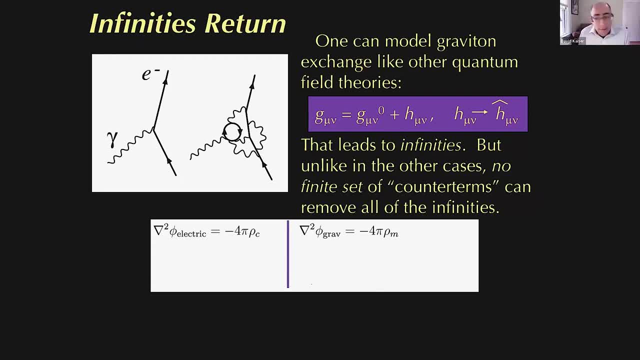 that some of our favorite wranglers- or my favorite wranglers- were super excited about back in the 1840s and 50s- people like William Thompson and James Clerk Maxwell. They were working out this electromagnetic or sorry, this mechanical worldview, where they found these mathematical analogies. 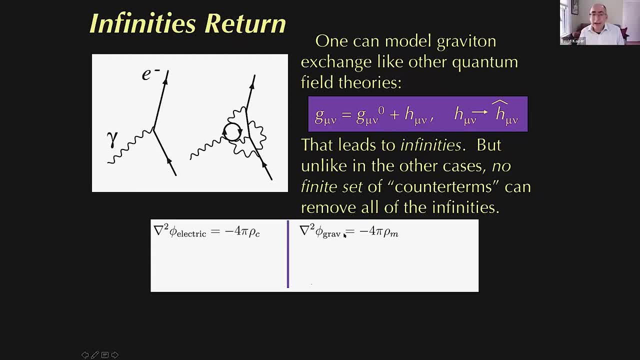 between, say, electrostatics and Newtonian gravity. They can each be written in terms of some potential, some function that extends throughout space and changes over time. In the electromagnetic case, the electromagnetic potential could be understood as responding to, as we'd say, sourced by where the electric charges are. 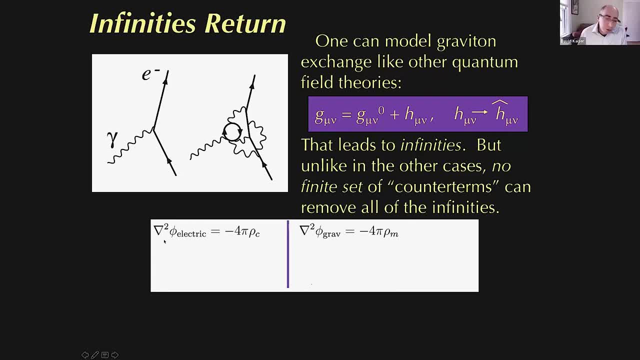 So we could look at the variation, the gradient squared, of the electric potential as arising from the charge density, the charge per volume. and if we just do some dimensional analysis, just some quick dimensions, without trying to really calculate things carefully, we can see that the charge density goes like the electric charge. 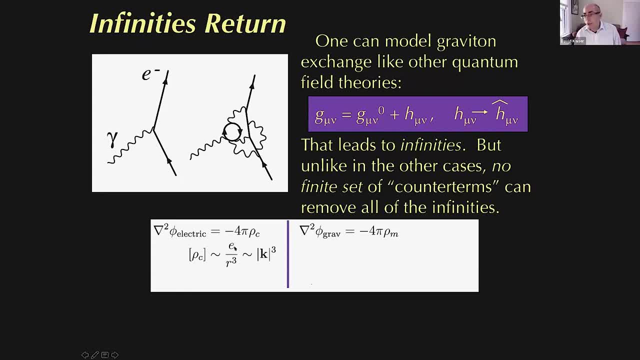 per volume. So it's like some charge, whether it's the charged electron or some larger collection of charges divided by some volume. Also remember, as the wranglers certainly well knew, that this all-important quantity, the wave number, goes inversely like some characteristic length, So wave. 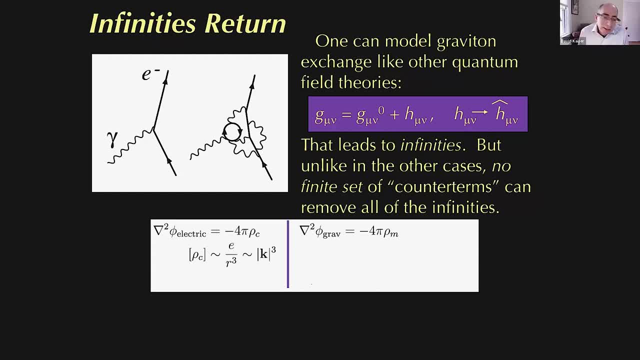 is inverse to wave length, And so the charge density in sort of appropriate units goes like the wave number cubed, As I mentioned, at least briefly some time some lectures ago, the electric charge, if we choose to measure it in so-called natural or appropriate units. 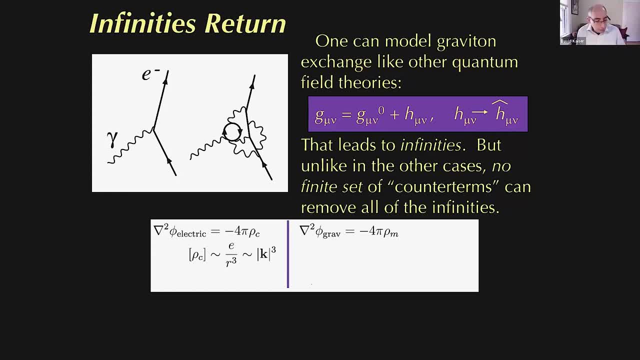 the electric charge is dimensionless. In fact the charge squared goes like 1 over 137.. It has a very particular, just a number. It's not a dimension for quantity. So dimensionfully, dimensionally, the charge density, to which the electrostatic potential is sensitive, scales dimensionally. 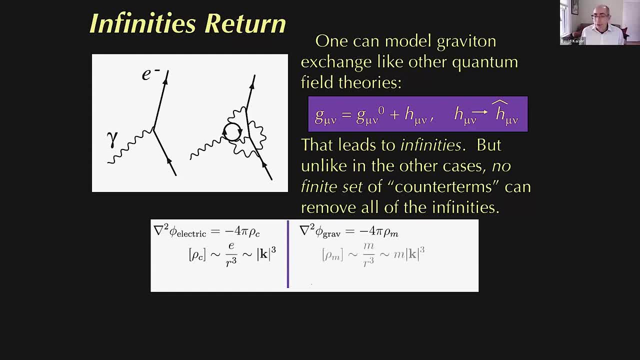 like the cube of the wave number. Now let's try to follow that analogy for the gravitational side. Even for Newtonian gravity, the very similar scaling holds even for Einstein's more complicated version. Remember that the gravitational potential is sourced not by the electric charges but by 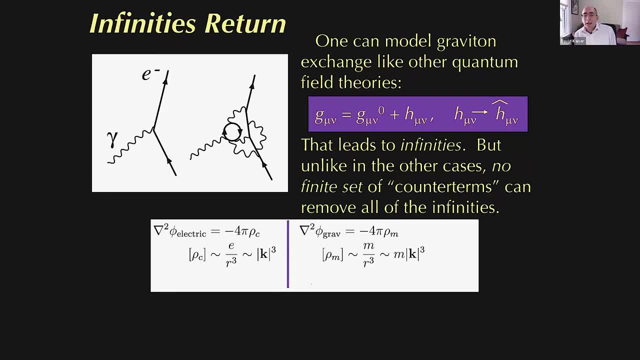 masses, or eventually, in Einstein's version, by mass energy. So we have to worry about the dimensions of this source over here, the mass density. So you can see that the gravitational density, well, that goes like by some characteristic mass divided by volume, it's a, it's a density. 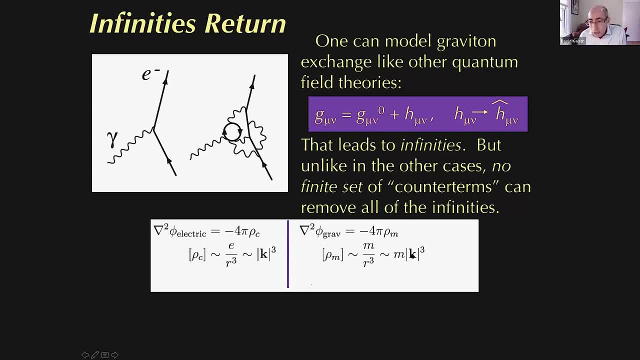 the volume factor, we just convinced ourselves scales like the cube of some wave number. but the mass, unlike the electric charge, the mass is also dimension full, and so something that was not known to either William Thompson or James Clerk Maxwell, but has become really clear to theorists over the course of the 20th century, is that that dimension for quantity mass, actually. 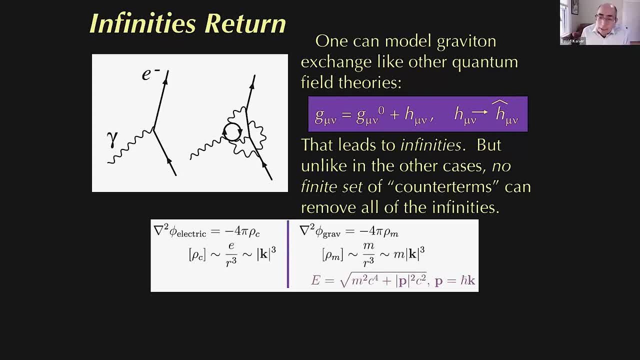 matters quite a lot. thinking just from relativity, we saw, thanks to Einstein, that energy, mass and momentum are all basically interchangeable. the famous expression e equals mc- squared- we saw briefly- is really more generally a relation between energy, mass and momentum and they're all interchangeable, with some kind of change of units given by the speed of light. but if we 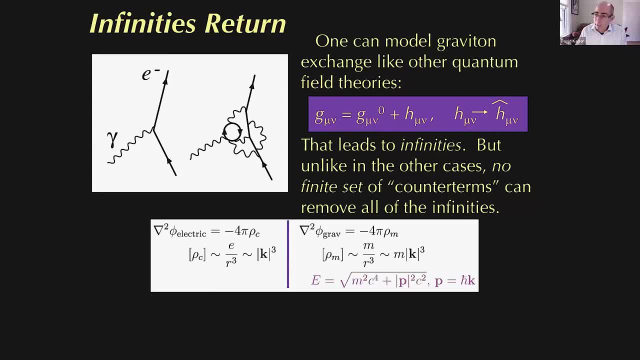 measure these quantities in kind of appropriate units. they're all dimension, full energy, mass and momentum, and in fact they're all really kind of interchangeable. there's not a sharp, a sharp conceptual divide anymore in relativity between mass, energy and momentum. then that's the relativity side. then from quantum theory we saw, thanks to 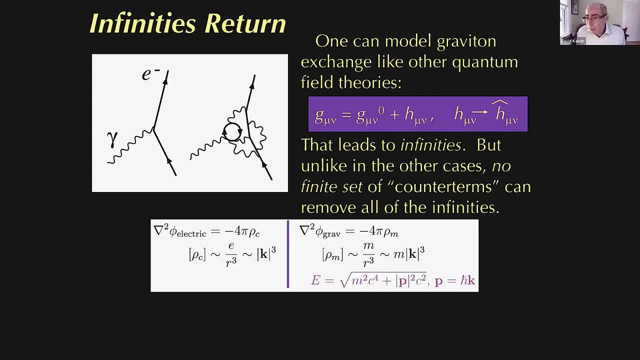 people like Louis de Broglie and built into the Schrodinger equation and much else, that momentum and wave number themselves are directly related. in fact there's. they're related by a different constant of nature, Planck's constant. so if we go back and find a scaling, even classically, for 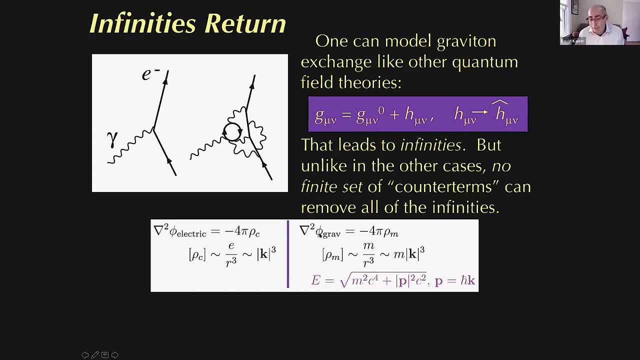 Newtonian gravity, that the source for these gravitational kind of disturbances, which we might choose to to quantize, if they're sourced by a mass density that actually has a different scaling, with wave number and therefore with momentum, than in the, than in the electrostatic case, there's a disanalogy between, say, quantum electrodynamics and a putative 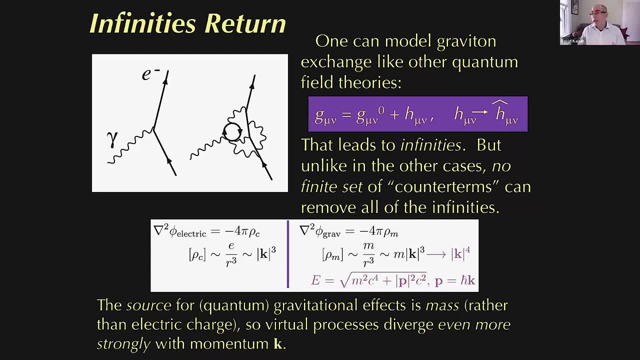 quantum theory of gravity, that has everything to do with insights from relativity and quantum theory. e equals mc squared and the de Broglie wavelength, and so what that means, when you try to just follow an analogy to these other ones, is that there's a difference between quantum 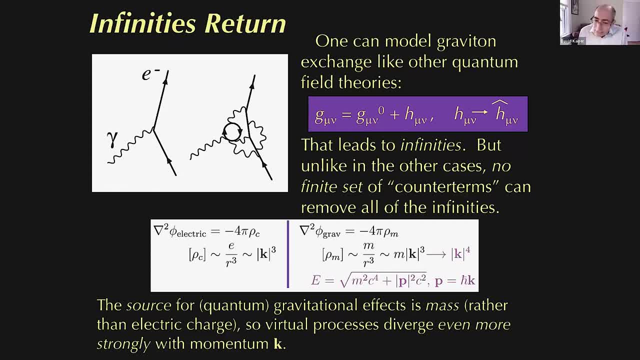 theory and quantum theory, the integral. when we try to count up the, the effects of virtual gravitons, the integrals diverge with momentum more violently than even the ones due in for the other forces. and it really comes to these very elementary notions from both relativity and quantum theory. The scaling is 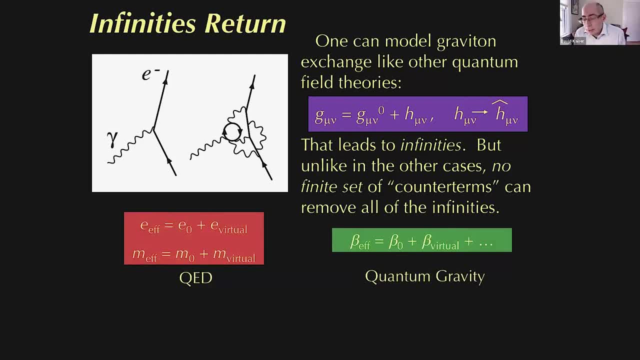 different. What does that mean? in slightly more practical terms? We saw again going back to these insights from Shinichiro Tomonaga during the war in Tokyo and then independently kind of rediscovered soon after the Second World War by people like Julian Schwinger and Richard Feynman. 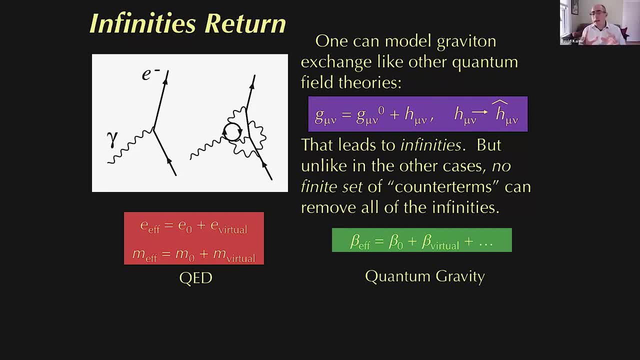 that for quantum electrodynamics, they could always arrange their equations so that they never had a bare infinity on its own. They could always organize things as these kind of input-output relations. This was the heart of what became known as renormalization And that you could always have. 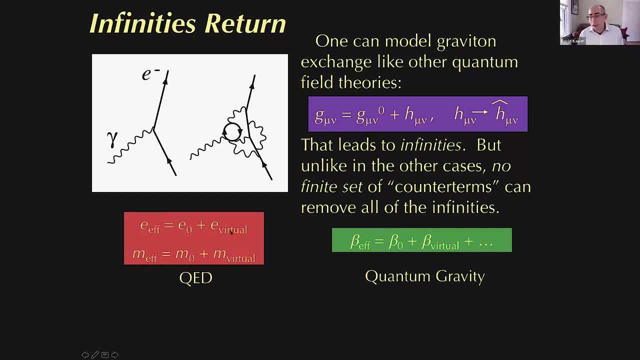 these combinations, which remained finite, even though each of these on their own would diverge, usually logarithmically, with momentum. So each of these, if you try to calculate them on their own, would be formally infinite, but their sum was well-defined and finite. And what people like? 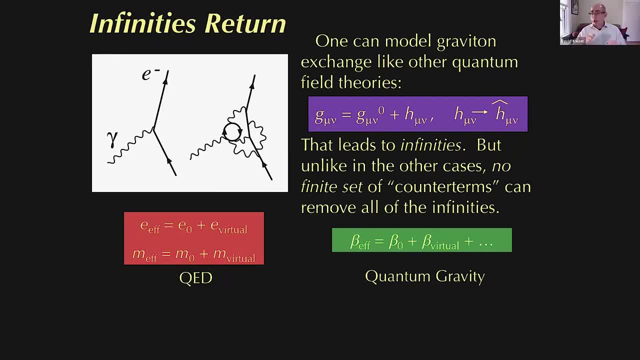 Freeman, Dyson and others showed is that that trick holds order, but it doesn't mean that you can do anything about it. You can't do anything about it. You can do it by order. in perturbation theory You can make arbitrarily precise calculations. 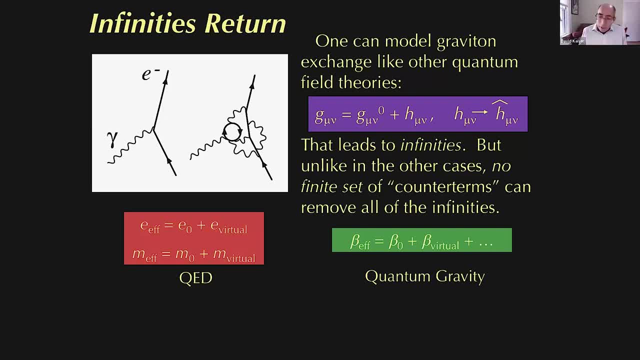 and these cancellations hold all the way through. What it means for quantum gravity to have these more violent divergences, the stronger growth with momentum for these virtual graviton processes, is that you need actually an infinite set of these kind of absorbing coefficients. 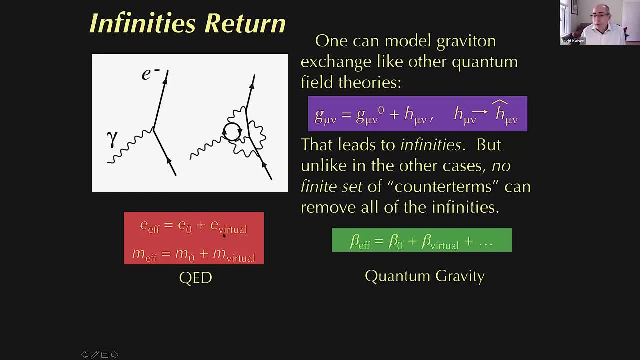 that you can't arrange things just in the input-output way. You never have a finite number of these kind of absorbing infinities, So you can never absorb or cancel the infinite divergences, at least from this first kind of approach to quantum gravity. 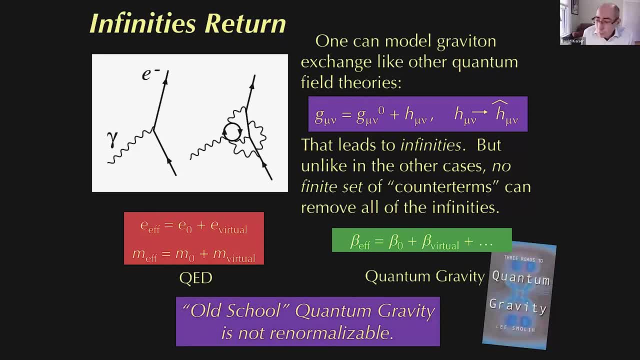 So this leads to a hard problem, And one of the first books that I'll recommend today is this really lovely book that came out 20 years ago by physicist Lee Smolin. It's, I think, a very accessible, very nice book. He is a leading theoretical physicist. He's also a very gifted. 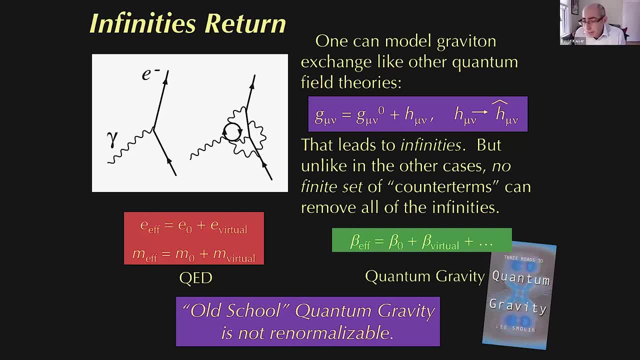 author. This book is called The Three Roads to Quantum Gravity, and he really goes through some of these early arguments as to why the analogies failed time and time again over decades, for generations, when people tried to apply insights from something like quantum electrodynamics. 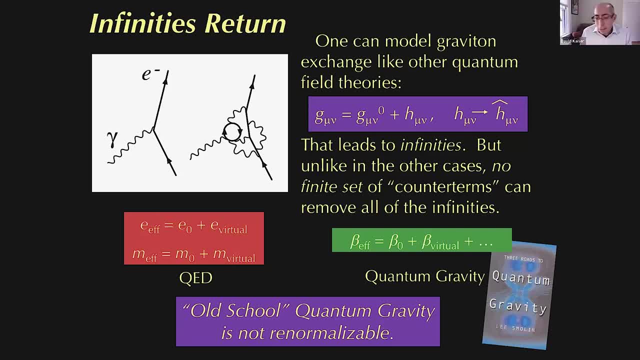 to try to kind of just do the same thing for quantum gravity. So what now? we can call somewhat tongue in cheek old school quantum gravity is not subject to renormalization. You can't get any sensible, finite answers from trying to deal with the zigzagging of 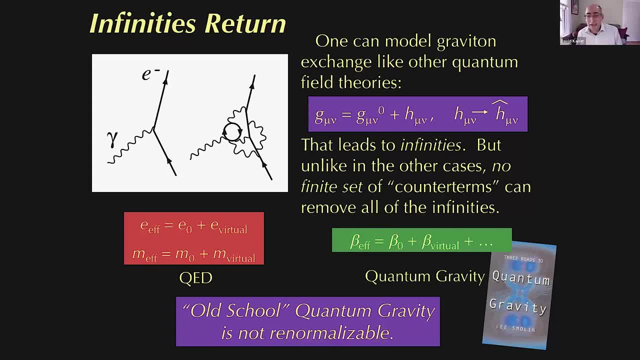 virtual gravitons, because there's stronger dependence of gravity on things like mass and momentum. Okay, So read Lee's book. He'll explain it better than I do, but I think that's in brief some of what's going on over really decades in this first wave. 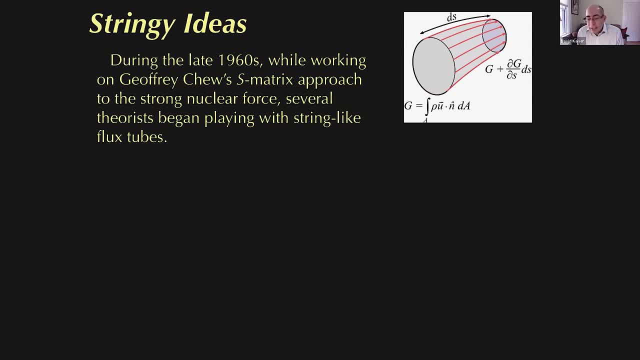 of effort to combine gravitation and quantum theory. While all that was unfolding and becoming kind of clarified, the dead end was becoming clarified in a quite different branch of physics. Now going back to ideas about the strong nuclear force, high energy, nuclear physics and 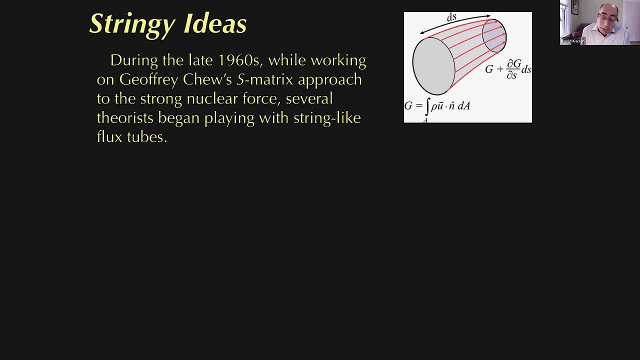 particle physics In the late 1960s, a number of theorists, some of them actually at the time based at MIT, were trying to make sense of this. one of these main approaches we looked at from the middle decades of the 20th century for the strong force, Jeffrey Chu's so-called 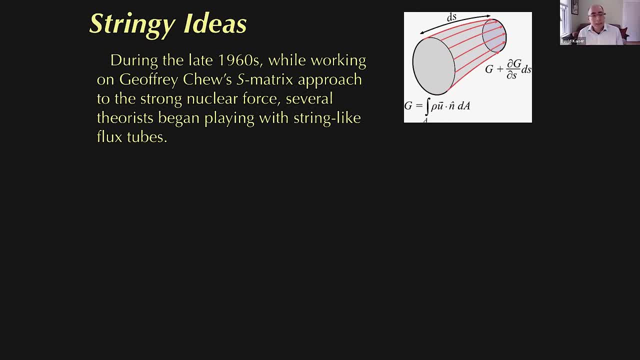 S-matrix force. He was sort of flipping these Feynman diagrams around, finding these self-consistent dynamical solutions where basically nuclear particles could make the force-carrying particles. that would bring the particles together to make those force-carrying particles. You find one self-consistent set of relationships among the particle zoo. 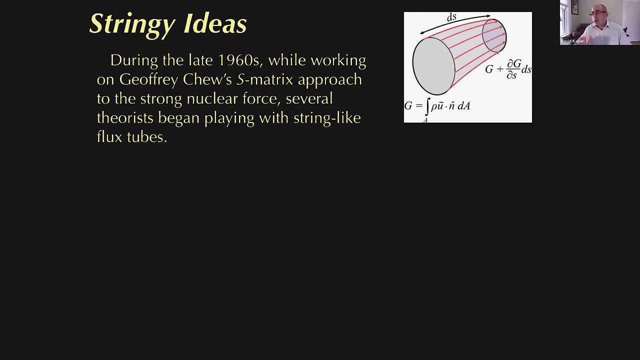 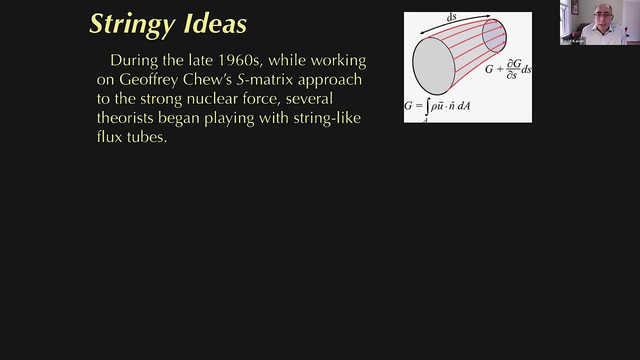 That kind of thing was a cylinder or tube, a kind of a string-like flux tube, And that really was, as far as I'm concerned, what might explain the nuclear force that keeps things like protons and neutrons bound with an atomic nuclei. 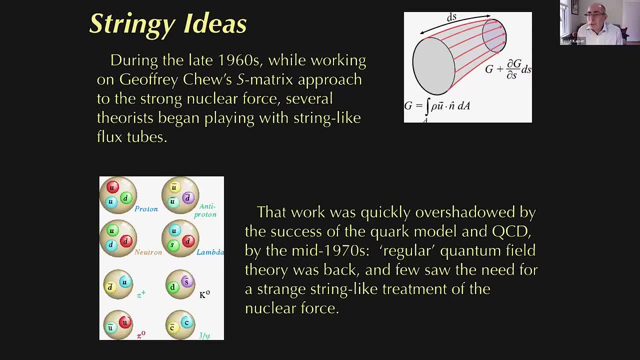 That was being published, starting in 1967-68, by a small little circle of kind of specialists. It was curious, it was interesting and it was very quickly overshadowed for the reasons that I think we can make sense of, given what we saw together. 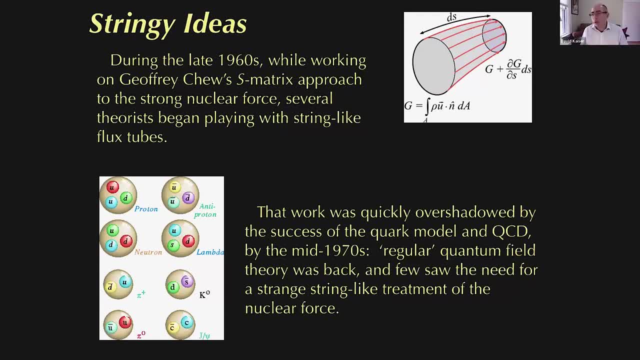 the kind of gathering force, the kind of choppy road toward the quark model and ultimately quantum chromodynamics. so we saw, although the idea of quarks had been introduced as early as 1964, it took really a solid decade into the mid-1970s. 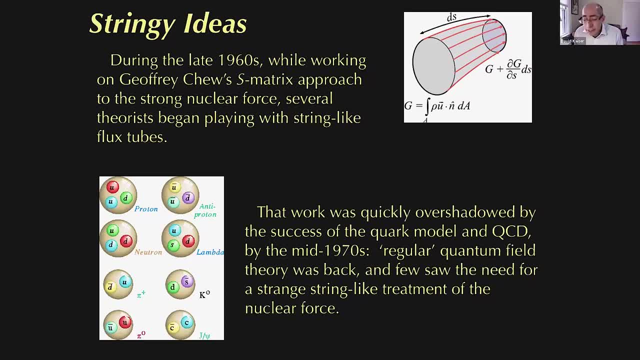 before. even the quark model proponents themselves, like murray gelman, were saying that this is, these are physical entities in the world. and it was really only after the successes of this very specific quantum mechanical field theory, quantum chromodynamics or qcd, where the various pieces 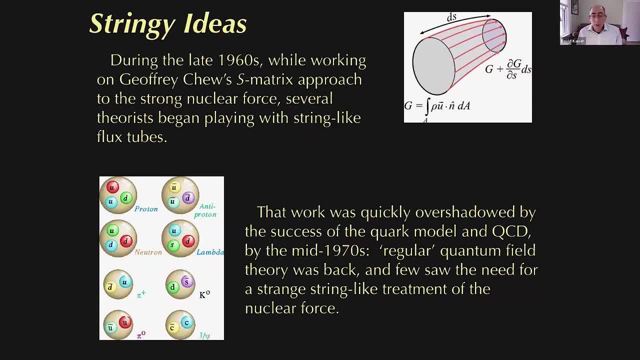 came together and also got some helpful kind of uh, bolstered by some new experimental inputs. so by the mid-1970s it looked like people had this strong nuclear force well in hand and all these kind of weird funky geometrical flux tube things from the kind of jeffrey chu inspired work. 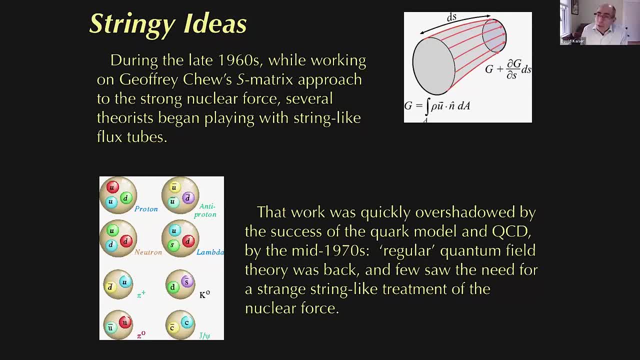 that kind of faded away. it wasn't proven to be wrong, it just seemed like it was no longer the best road forward. the quark model finally seemed to be scoring success after success, and that was built as a model of quantum quantum mechanics and it was built as a model of quantum quantum. 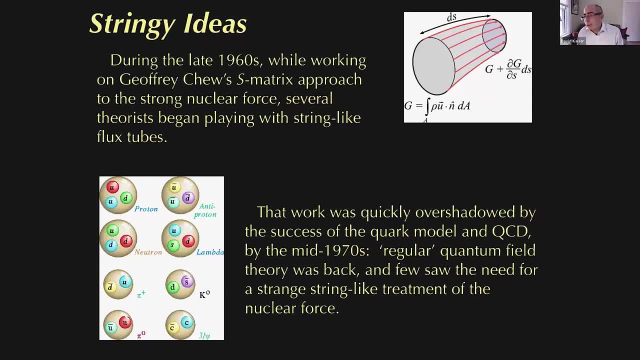 electronics. so you imagine elementary point particles with certain kinds of charges, in this case quarks and gluons, and you trace the virtual particles, uh, among them, and all that in a, in a framework much more like quantum electronics. so the early string ideas really kind of fell away. 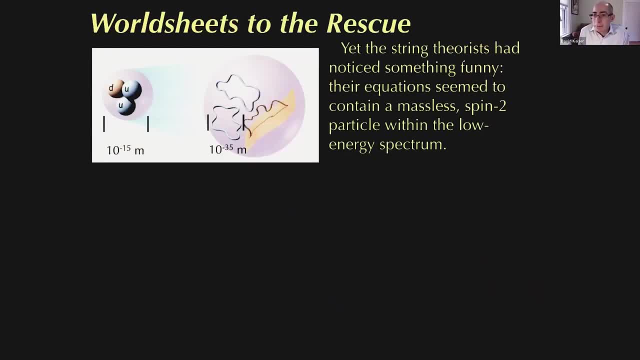 not because they were just proven, but because they seemed, um like, uh, maybe not the best way forward to understand the strong force. before people stopped paying attention, though, a few of the small string ideas were really kind of fell away and they were kind of like the strong force. 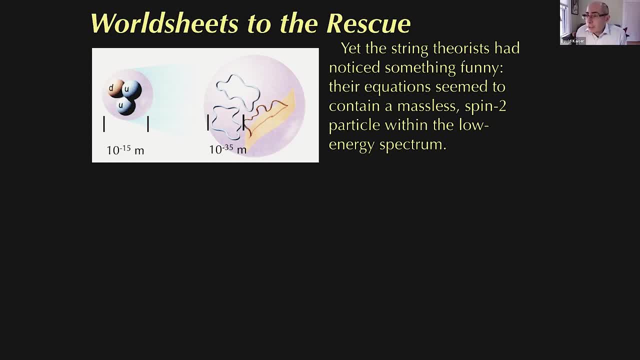 in the circle recognized something curious in their equations for the jeffrey chu, like for the string approach, stringy approach to the nuclear force. if you look at the low energy limit of these complicated, self-consistent, highly non-linear equations, it looks like in low energies. 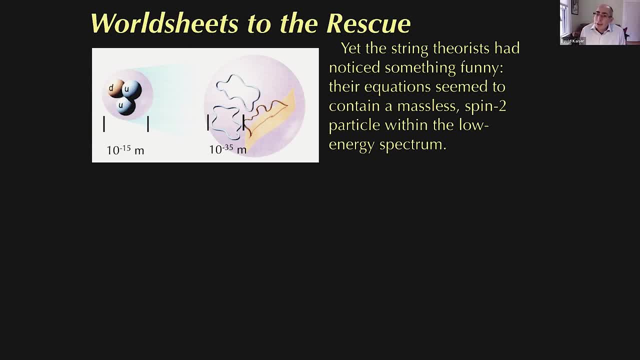 this seemingly nuclear type interaction includes a the exchange of a massless spin two particle, and some people said: wait a minute. i remember hearing something about that. a massless spin two particle is a massless spin two particle and it's a massless spin two particle and it's a. 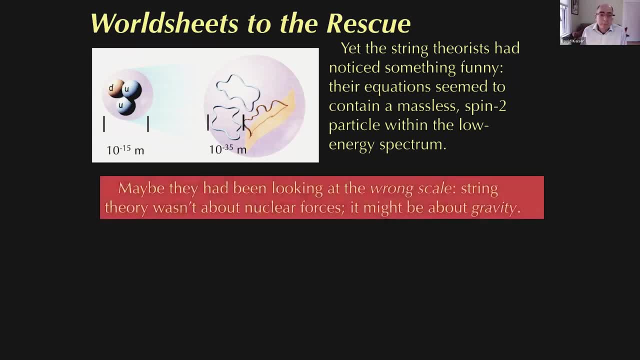 maybe comes up in other contexts, like in gravity, and so a few groups who who knew about the, the kind of strong force, stringy work, said maybe this, these insights about strings, extended 1d structures, maybe it has nothing particularly to do with the strong force, but maybe that was a theory about. 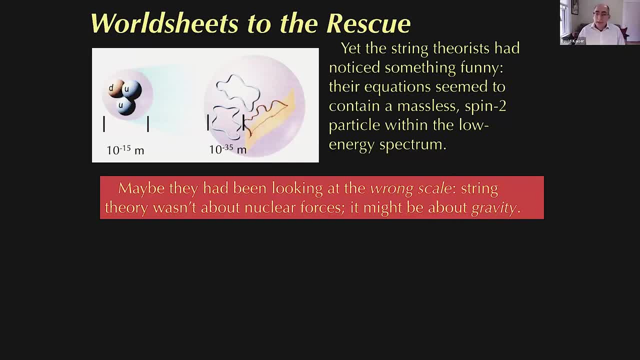 gravity and not about nuclear particles. if so, then the kind of typical length scale for these things would not be the size of a single nuclear particle like a proton, it wouldn't be femtometers 10 to the minus 15th of a meter. it might be the Planck length. 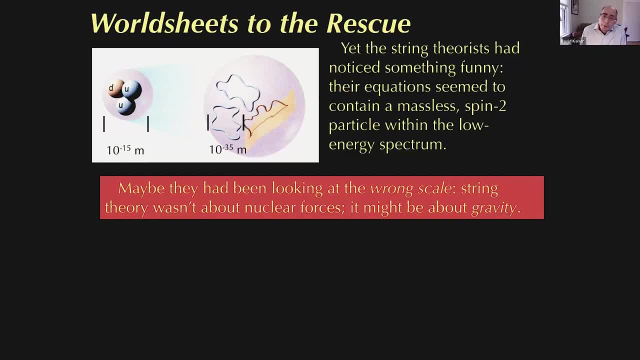 the smallest possible length, uh, longer than which one should be able to ignore quantum gravitational corrections. maybe the actual fabric of of einstein's warping space-time consists of these unimaginably tiny scales of a play, of these extended one-dimensional objects. maybe the strings are what give rise to the effects of gravity, not to that bound. 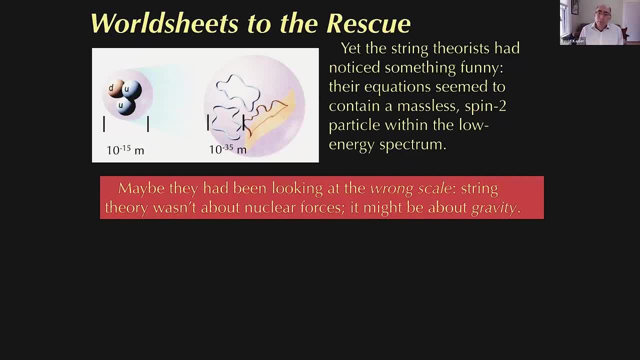 uh, quarks within a proton, for example. so because the low energy behavior of these stringy structures gave rise to just the kind of particle needed to make sense of gravity, uh at a in terms of particle exchange, the ideas about string theory became very interesting to a small circle as a. 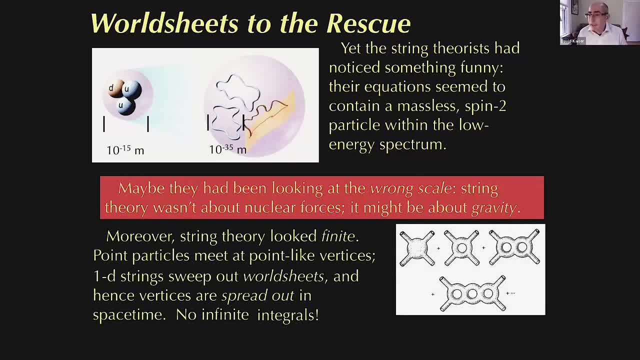 possible road toward quantum gravity, quite different from the kind of particle scattering qed type model. in fact, it looked even more promising again as many of these folks began to put together a model of the kind of particle scattering qed type model and they were able to put it together by the early and mid-1980s- roughly 10 years later. then it looked like calculating. 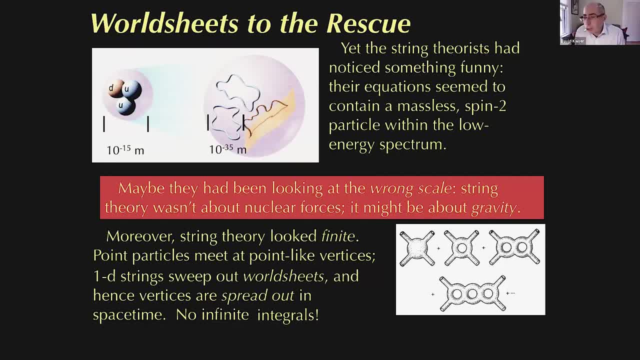 effects, quantum virtual effects of in this string theory of gravity might actually avoid all these messy infinities altogether. why was that? the infinities keep arising in these quantum field theories? because people integrate up to an infinite virtual particle momentum. that's like saying, that's like imagining that we could model the exchange as the scale of gravity. 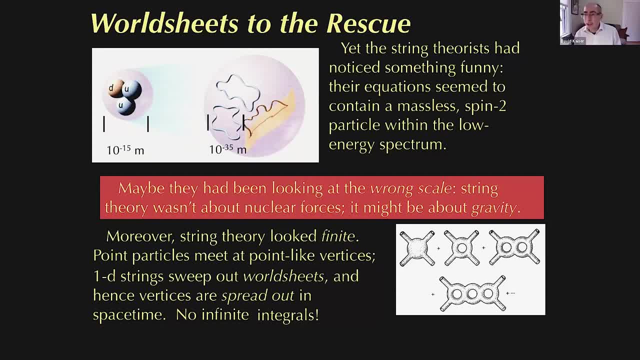 and that's like a virtual force carrying photon and electron that they meet at, literally, at a mathematical point. they meet in a region of infinitesimally tiny region of space, the the that suggests that they could be scattering off each other with a borrowed momentum up to up to 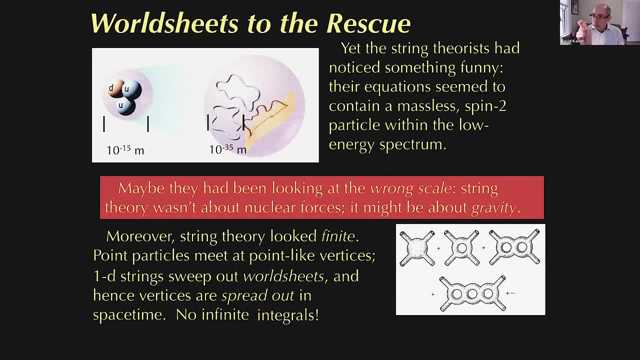 infinity. up to one over zero, the delta r could shrink to zero. that means that the momentum exchange could in fact become infinite, which is why you have to integrate those integrals up to infinity. well, these string objects are actually the same as the string objects, but they're 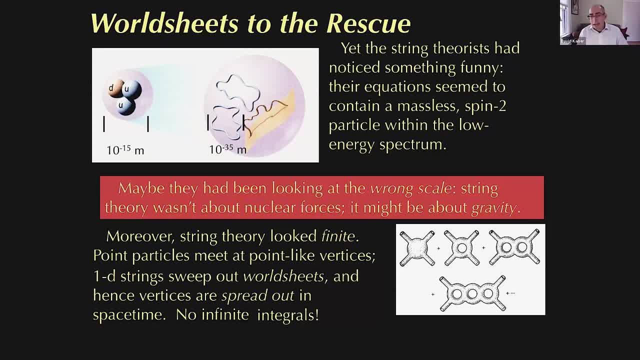 actually sweeping out not world lines through space and time but actually world sheets. they're extended objects, so the the analog feiman diagrams never pinch down to a single mathematical point. in fact you have these kind of pants, legs, structures where you have a kind of one kind of 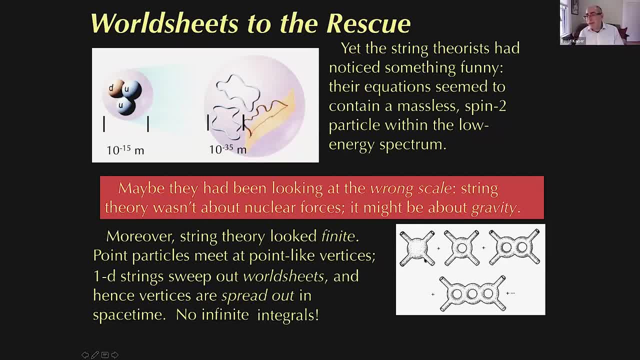 extended structure might blend into others, but they never pinch down into a mathematical point. so if you never have these point-like vertices in the kind of scattering among these putative strings, you can't do anything about it. you can't do anything about it. you can't do anything. 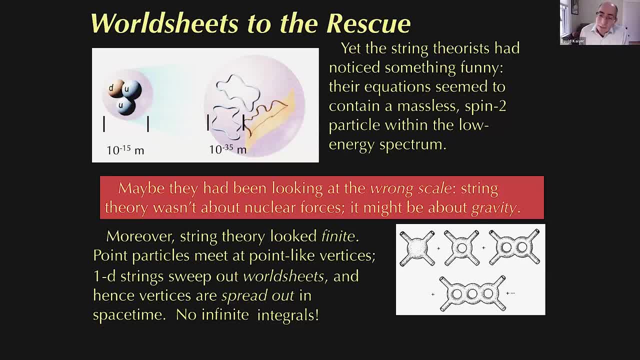 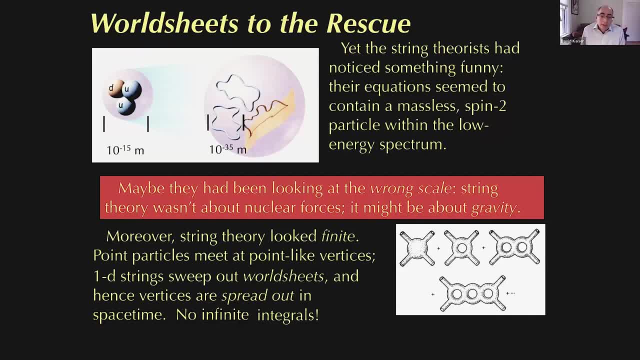 of old-school or classic approach to quantum gravity. so maybe you could have a finite theory of gravity that has the right kind of particle exchange in the appropriate limit and avoids infinities. so why weren't we done in 1984? well, because the same scholars found a pretty interesting 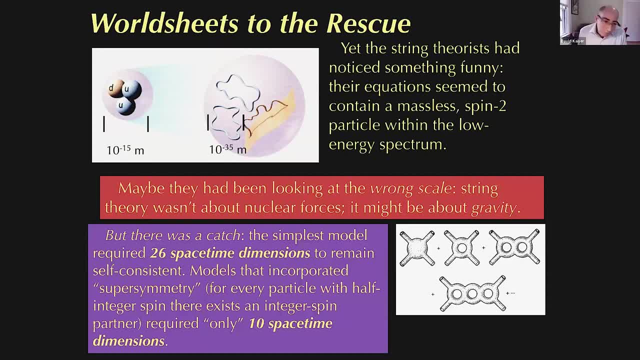 way to do this, and so they came up with the first model that was called the, the simplest model that could be written down, that could be applied to, to a gravitational model where these strings could be dancing around at the Planck length and giving rise to the to inappropriate. 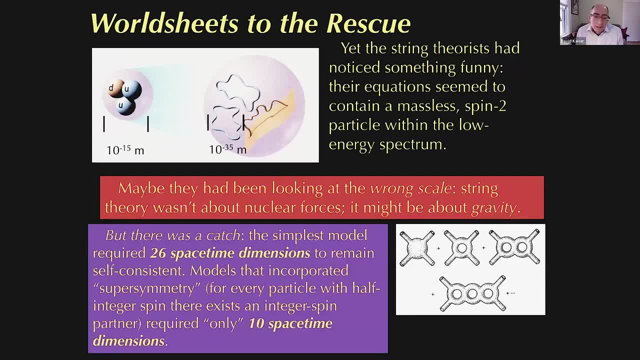 limit to Einstein's general theory of relativity. they only could live mathematically in 26 space time dimensions. I put that in bold and italics, so we'll linger on that for a second. the earliest self-consistent model, when applied to gravity to get the right limit at low energies to make it look like Einstein's. 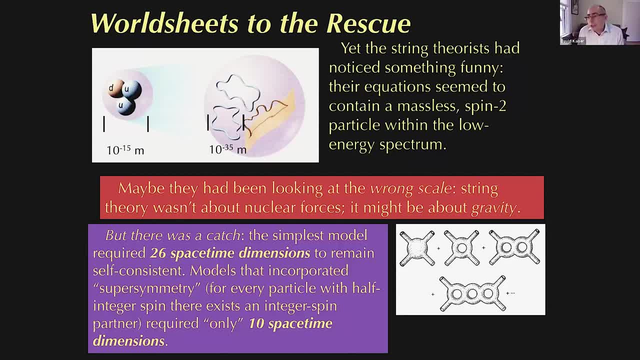 theory, at low energies these strings weren't dancing around in three dimensions of space at one of time. you know x, y, z plus t. They could only dance around in a mathematically self-consistent way if they were living in a 26-dimensional space-time. It seems pretty clear. 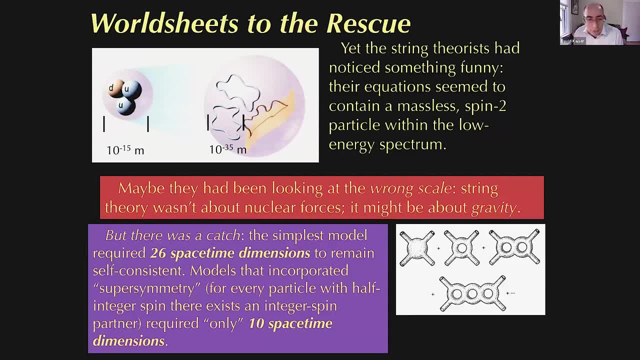 that we live in a four-dimensional space-time. So what's going on? A little while later, some of these physicists found that they could actually make these mathematically self-consistent string models of gravity if they incorporated a particular symmetry- strictly hypothetical symmetry. 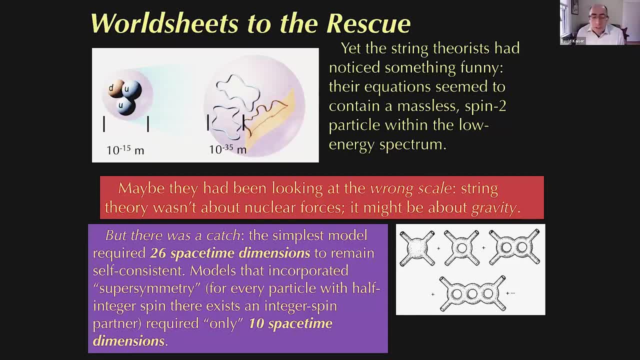 for which, even to this day, there's no empirical evidence at all, A symmetry called supersymmetry, which suggests that for every known particle, every quark, every electron, every neutrino and all the rest, there is a partner, a super partner: particle with the same mass and 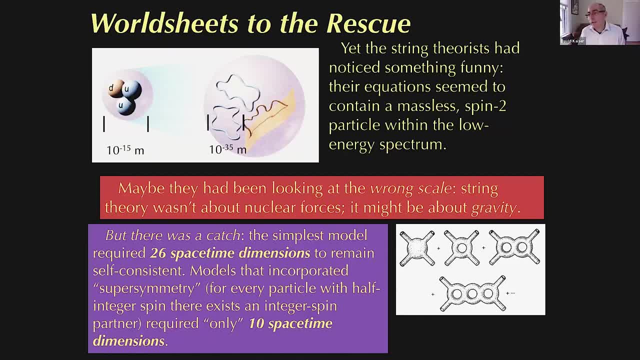 same charge but one half unit more of spin. So for every spin one half particle, like quarks and electrons and neutrinos, there would be integer spin super partners and vice versa. So for every integer spin photon there'll be a half integer or three halves integer super partner, like a. 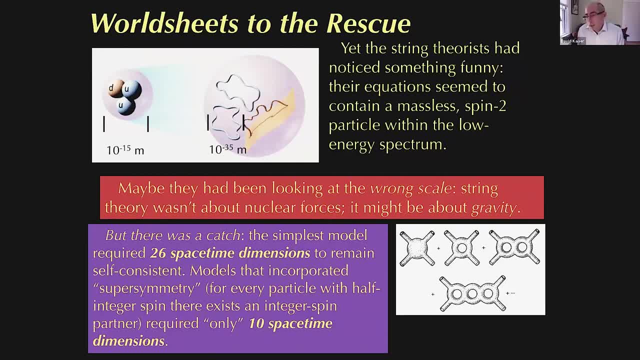 fotino. For every quark there will be a squark, And so, at the cost of doubling every single known form of matter, these superstring theories could be formulated in only 10 dimensions of space-time instead of 26. That's getting more than halfway. 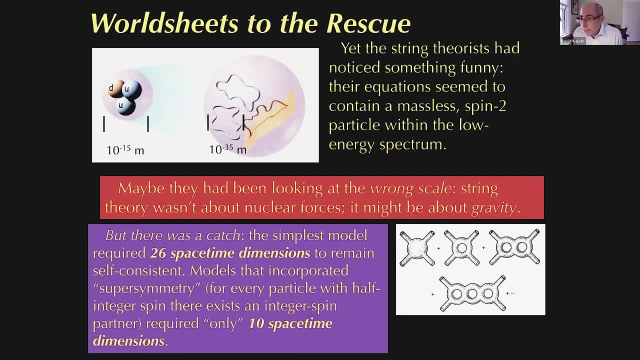 there. but it still means a lot more structure than what we seem to measure or just observe in our daily lives. So these early superstring theories for gravity had some unbelievable promise. These people weren't, you know, kind of deluding themselves that these could be of. interest, but there wasn't some sort of guarantee that these could be of interest. but there wasn't some sort of guarantee that these could be of interest. but there wasn't some sort of guarantee that these could be of interest, but there wasn't such a straightforward deal. 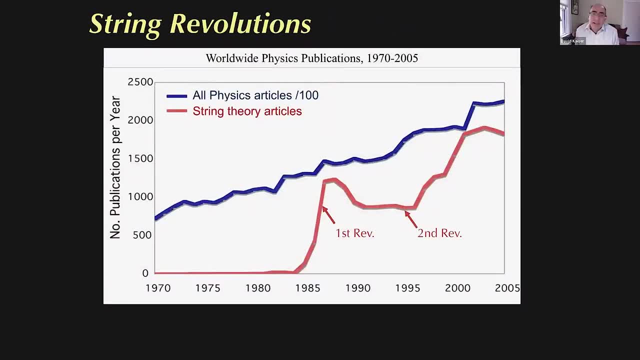 So we can then go to some of the kinds of plots that I love to make. Let's start counting stuff. So the blue curve shows all physics articles as covered by something called physics abstracts, a kind of worldwide consortium of physics-trained librarians in many parts of the world. 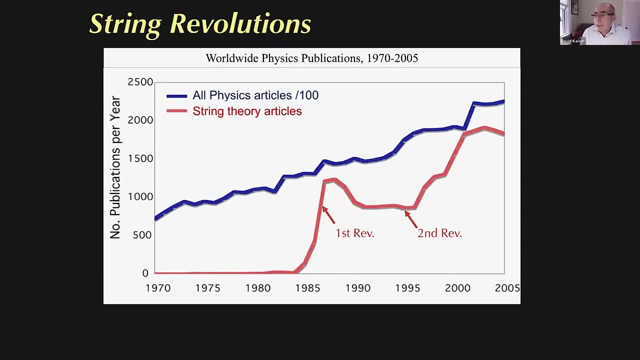 trying to literally count up and categorize by subtopic all the articles by professional physicists in the peer-reviewed journals in as many languages as they could master. So that's the blue curve and you can see it's growing fairly steadily over this period In the red curve- and I've renormalized it myself- 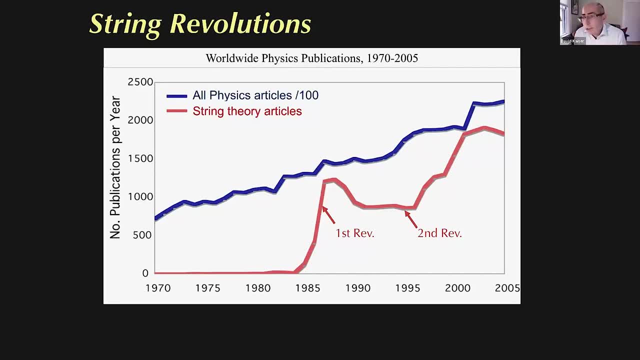 the red curve is then all the articles on string theory, including superstring theory, over the same time period. To fit them on one curve, I've actually divided the blue one by a factor of 100. So by the end of this period the red curves are about 1% of all the publications. 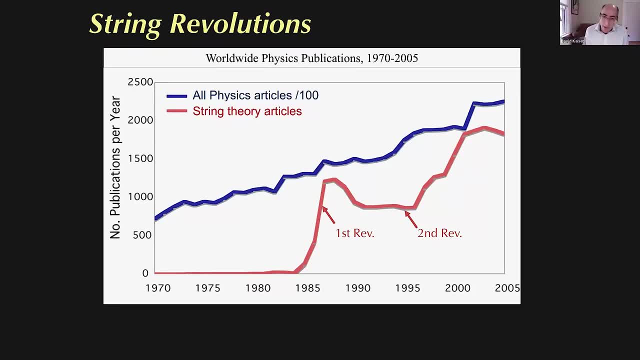 in all of physics They say they're almost equal, but I've cheated by making the blue curve change its amplitude by a factor of 100. So you see these very distinct structures in the effort expended on superstring theory compared to kind of global efforts on every branch of 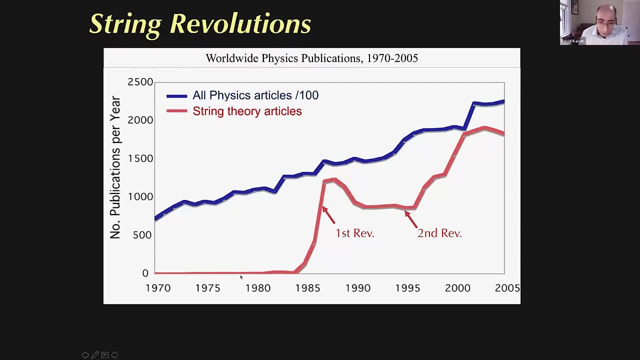 physics altogether. You see virtually no attention at all to string theory. it really is a very curious little specialty area. until the mid-1980s, What proponents of this work later called the first string revolution, which you have to know they only named after a second string revolution. no one. 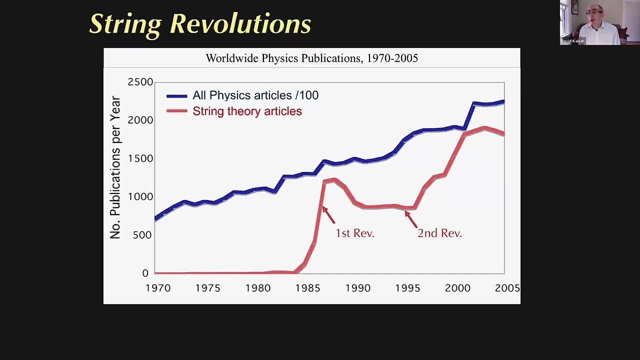 one world war one until world war two, so what later became called the first string revolution in hindsight was identified with this work. it was really published by a few independent small groups around 1984, where they began showing that the the stringy stuff could actually be, could include the: 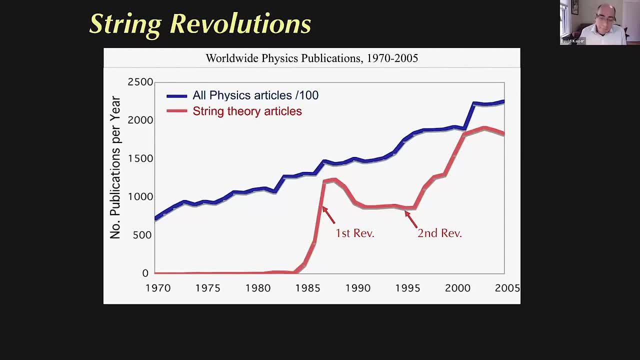 structure of gravity. uh, if you imagine that string-like filament to be describing, uh um, gravitational interactions at the Planck length, as opposed to nuclear physics? uh, and indeed there were several different self-consistent supersymmetric models published, all in 1984-85, and that led to an enormous burst, an exponential rise of interest in string theories, coming very. 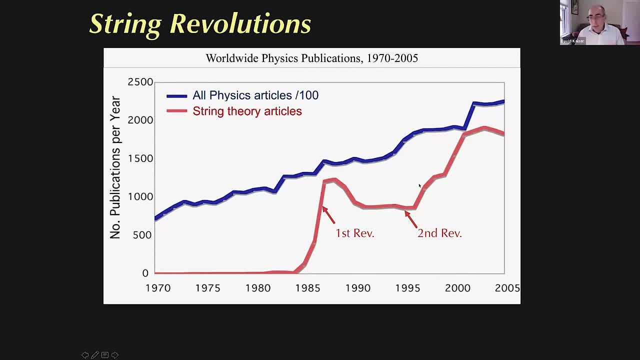 soon after that so-called first revolution. then there's a kind of plateau for about a decade and then there was what the proponents came to call the second string revolution, almost on right on schedule. 10 years later, what happened with the second string revolution? in brief, was that a few? 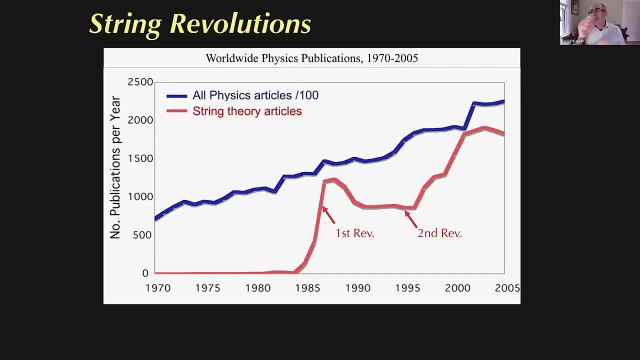 of these specialists found that what looked like five totally separate, distinct but self-consistent superstring models. they look different from each other. they all were mathematically self-consistent even though they they looked like they were different. candidates in the second wave of people like Edward Witten and other colleagues found kind. 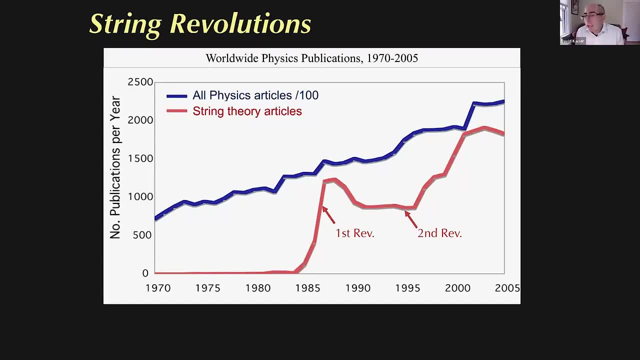 of one-to-one mapping. so in fact, these five different models might all be ways of expressing a single shared model. these might be almost, almost like coordinate transformations of a single structure. so if one performed what became known as a second revolution, so if one performed what became known as dualities, it really is analogous to kind of coordinate transformations you could. 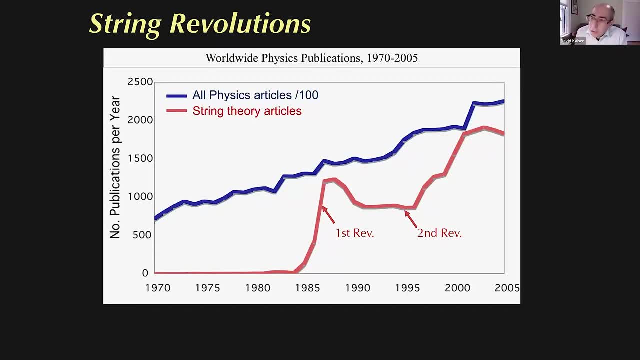 actually map feature by feature those seemingly five distinct models into a single structure. that got people excited again. you see another exponential takeoff of interest, so that by the early 2000s efforts on string theory, which had once been vanishingly tiny, occupy nearly one percent. 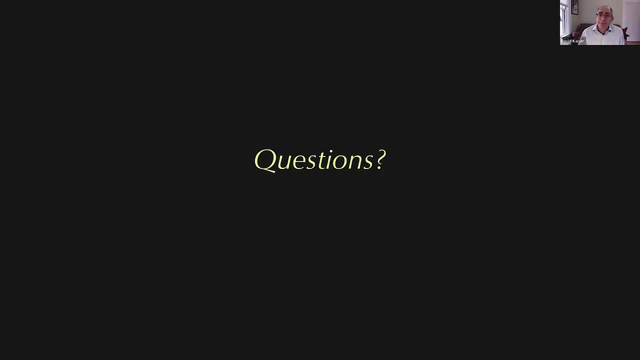 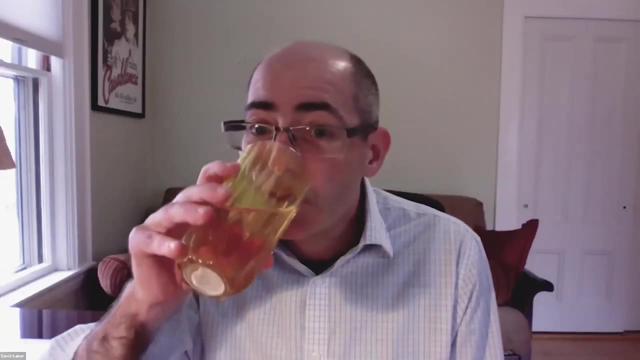 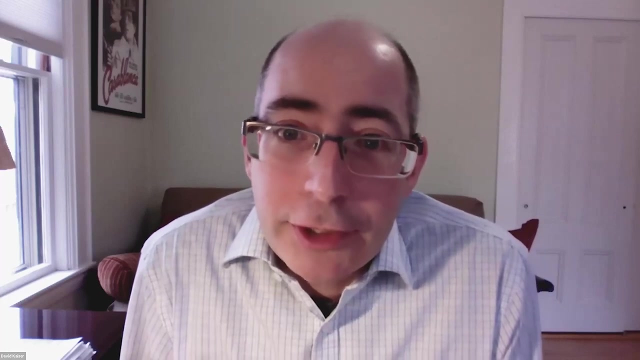 of all the physics output of all the physicists on the planet. so let me pause there, see if there's any questions on that kind of um alternate approach to an effort to try to quantize gravity. any questions on that? it's so straightforward, you're all convinced, you're. 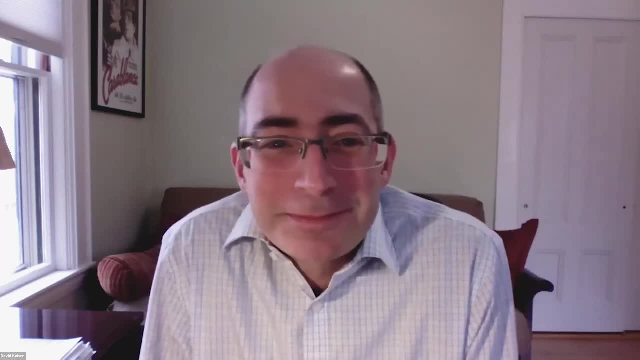 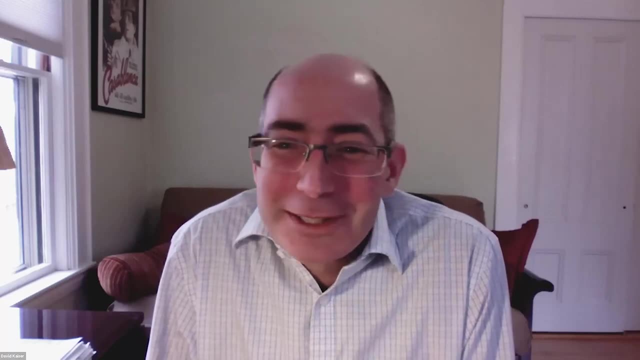 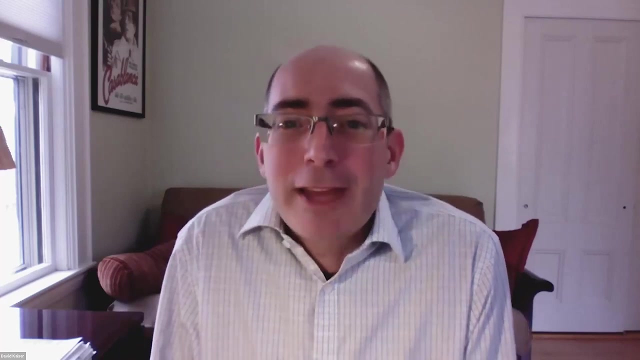 all now card-carrying string theorists. no, no lingering questions. julie is in. thank you, julian. i'll tell andy stromager he'll be glad. any other questions? if not, that's okay, of course, but i, um, i'll press on, uh, because, as if that weren't strange enough, boy, have i got news? 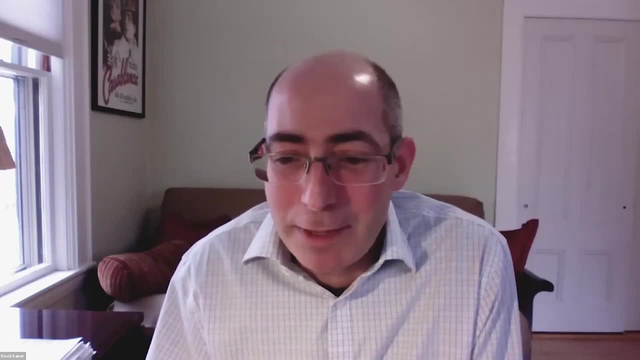 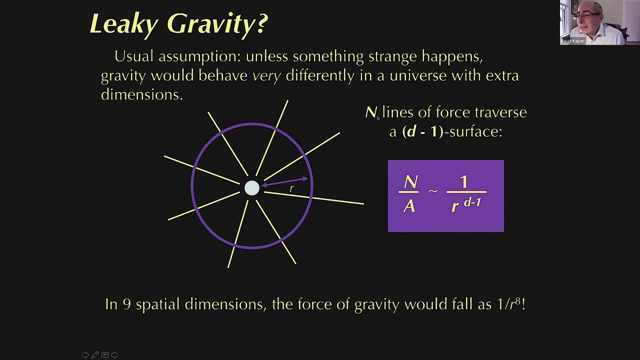 for you. you think that's strange. we live in 10 dimensions. let's, let's see where people take this, since they're now paying attention. okay, now i very blithely told you- and none of you seem to object- so clearly: it's the end of the term that these super string theories can only be formulated. 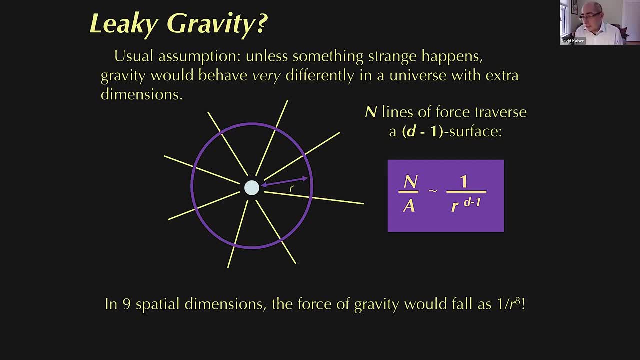 in a minimum of 10 space-time dimensions. they still only involve one time-like dimension. that means nine dimensions of space: height, width, breadth and six others all at right angles to them. i mean, i look at the- you know where the walls meet in my house and i can't find where the other six right angles would come from. so it's 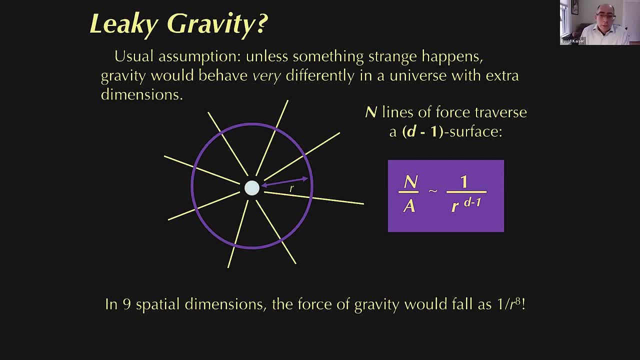 not just a failure of my own imagination, which fails all the time. this leads to some pretty strange sounding um possible implications. let's take a very simple one, going back again right to the very first um classes from this class sessions from this semester. think about, say, faraday's uh. 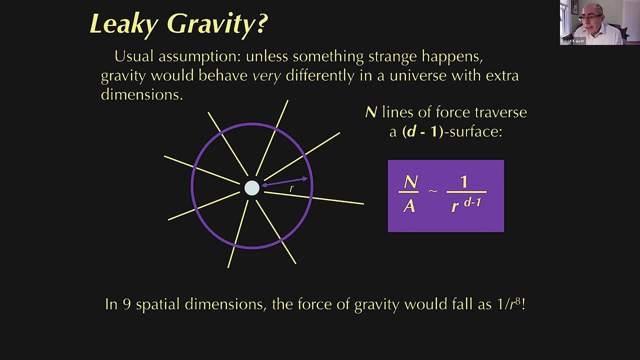 theory of lines of force, unless something very strange is happening. we really can't live in a tangent 10-dimensional world. if you imagine a single mass, some source of gravitation, some ball with some mass, a spherically symmetric one, to keep things simple, set it down at the origin of our 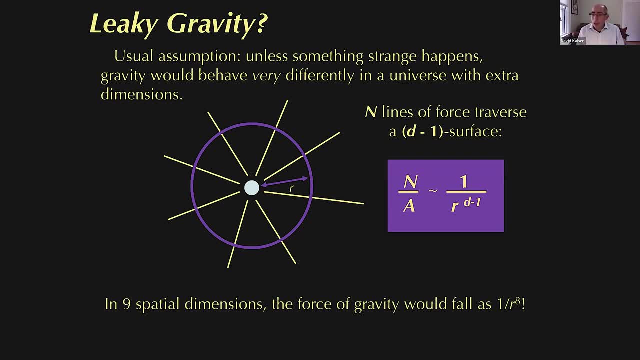 coordinate system. then, just like a single electric charge that got um michael faraday so excited in the 18, 20s and 30s, we can try to imagine how lines of force would emanate in this case: very simply, very spherically, symmetrically, lines of gravitational force emanating from that source. 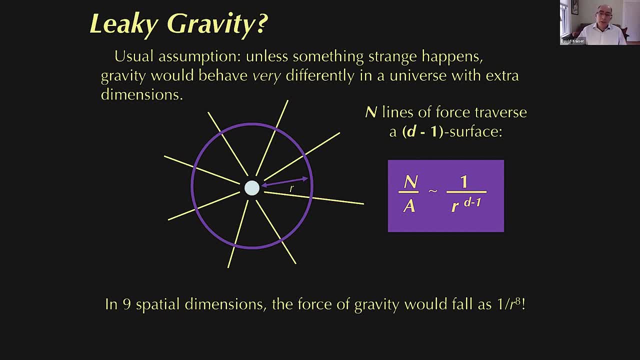 that mass m at the center. well, we can then try to do like faraday did and envelop, kind of surround our source with an imagined sphere. we can change the, the radius of the spheres. we can imagine how the strength of that force should fall off with distance. 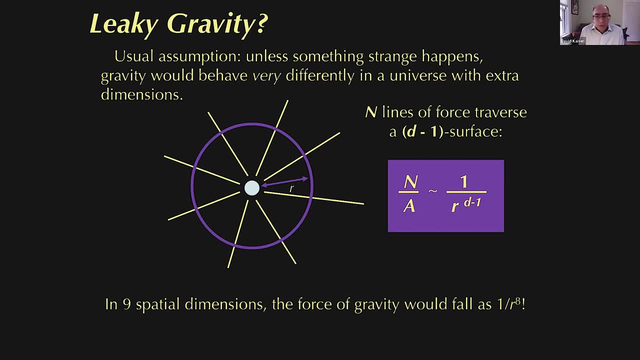 now again, as you, as you know, the surface area of some sphere will scale as one power less of the radius of the sphere, and the radius of the sphere will scale as one power less of the radius of the sphere, and the radius of the sphere will scale as one power less of the radius of the sphere. 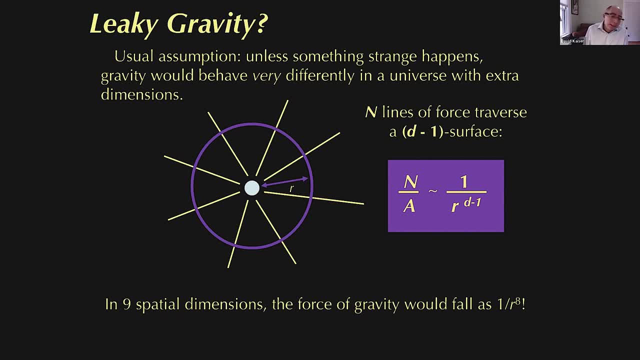 that holds in three dimensions, the surface area of a sphere goes like r squared, even though the volume goes like r cubed. that same geometrical relation holds for any dimensions of space, any hypersphere in particular, one that's in, say, nine dimensions of space, the surface area, we can very 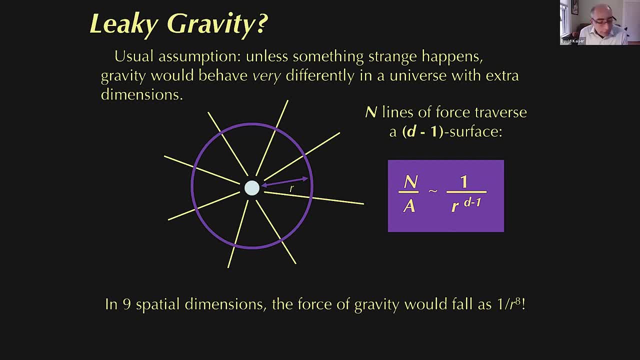 self-consistently, project um an appropriate sub-manifold and be all super fancy geometrical about it. we can calculate the surface area of a nine sphere and the area will grow like the radius to the eighth power to d minus one. so if we just redo michael faraday's- really, 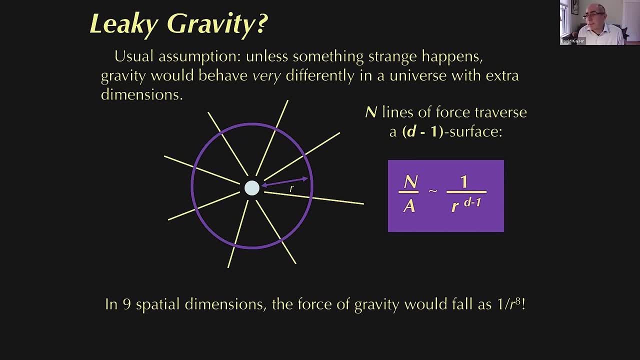 lovely, um ingenious, in fact, geometrical scaling. then if we really think gravity lives in nine dimensions of space, then we would expect newton's law to go like one over r to the eighth, instead of one over r, squared. why are we not? why are we finding inverse square laws, even in the context? 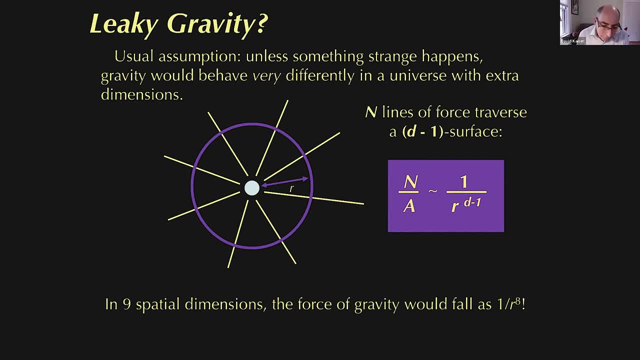 of einstein's general theory of relativity very high accuracy, whereas if we just have gravity kind of spilling out into across nine co-equal dimensions of space, we would expect a completely different behavior for the force of gravity. so what's going on when you say that this theory of gravity is 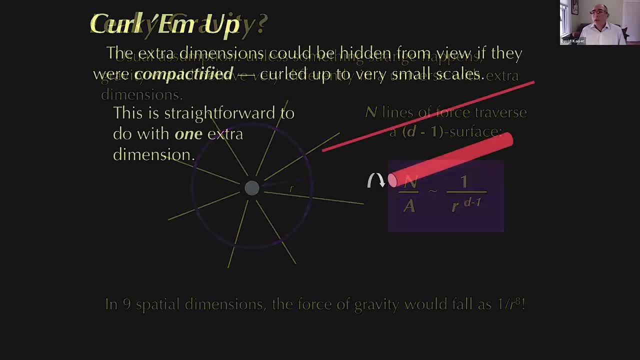 formulated in nine dimensions of space. one of the earliest efforts to address that is called compactification, which really just means make the extra dimensions super tiny. so the idea is that, for as yet unexplained or unknown reasons, the idea is that these extra dimensions of space are not arbitrarily extended. they're not macroscopic. i can't take a walk in dimensions. 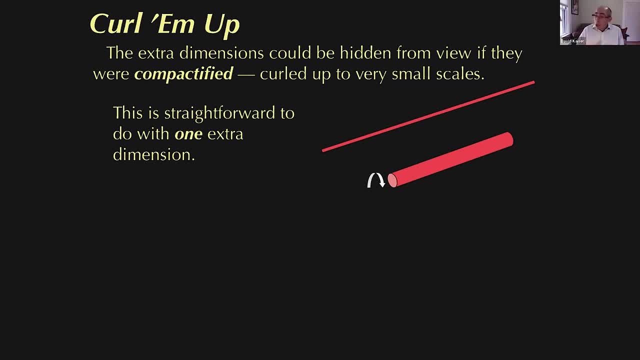 number um, numbers four through nine, because, at least hypothetically, they've been curled up onto each other and the way this the analogy is always made, and you might have heard before, we think about a kind of soda straw or a garden hose. now, if you're very close to that straw or hose, you can. 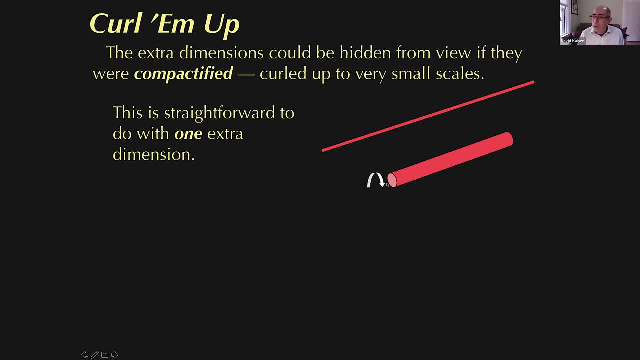 see, it's an extended object. it has both a length and a width to it. but if you look at that object very far away, it looks indistinguishable from a dimensionless line, an arbitrarily thin line extended only in one dimension. so the idea was: what if these extra dimensions of space are not? 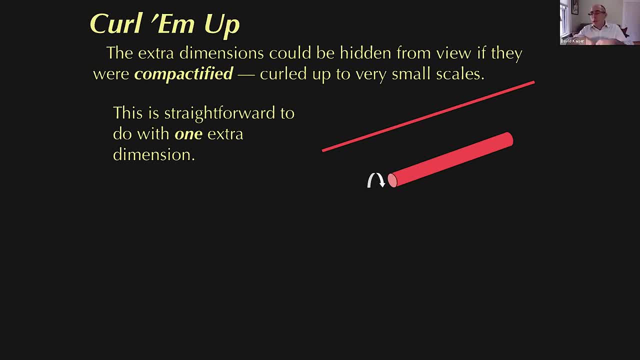 macroscopically large but in fact are curled up on each other. they have a kind of internal radius that never becomes large. it's controlled by some as yet hypothetical kinds of dynamics, so that from our clumsy human size scales what is actually a garden hose at an impossible 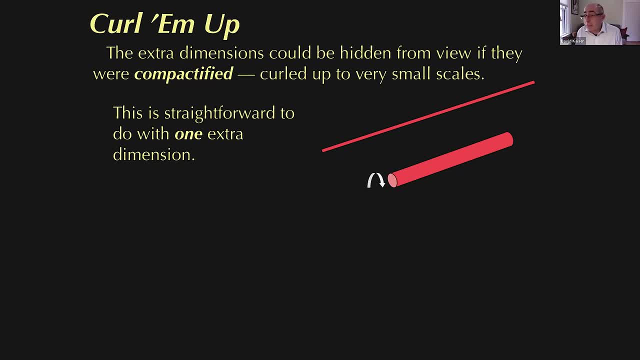 tiny radius looks to us indistinguishable from me, being merely a line of zero width. that's the kind of hand-waving version of how you could compactify, in this case one extra dimension, so we might live in a universe with x, y and z- macroscopic height, width and breadth, and then w. 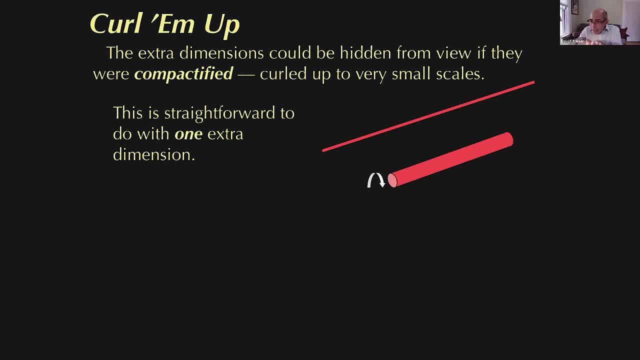 let's say some fourth dimension of space, but that one is a tiny little circle that if, uh, that we don't probe at, at low energies and so we never see anything kind of we never see this structure, because we're never able to see the structure of the universe, we're never able to see the structure. 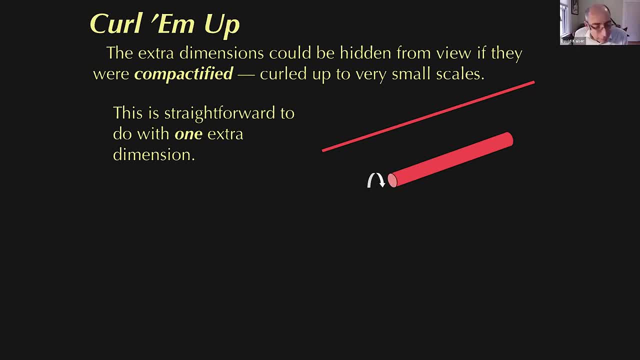 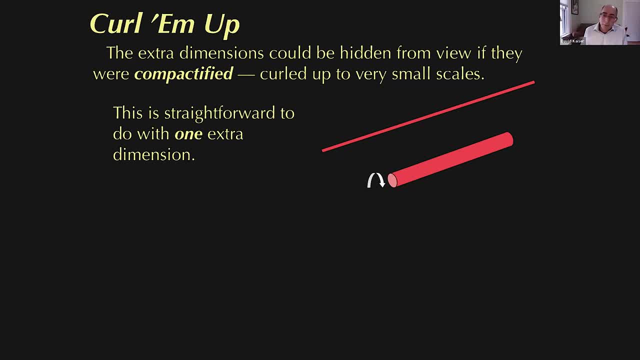 no way to know it directly because we can't kind of measure anything with such high um spatial resolution. so that's the idea: to compactify these extra dimensions. that works pretty straightforwardly if you only have one extra dimension space to kind of get rid of. but remember these superstring. 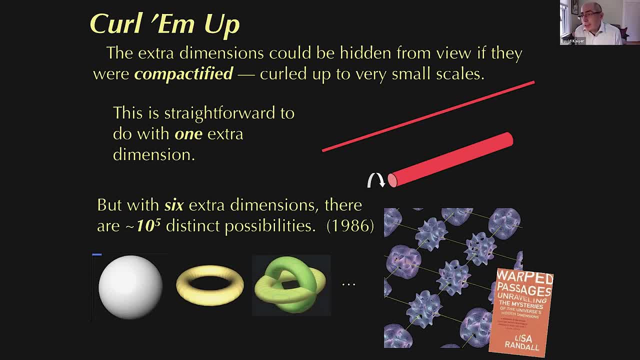 theories require at least six extra dimensions, nine dimensions of space plus one of time. so we we have three macroscopic ones that we can self-evidently move around in. so you have to compactify six extra dimensions, not just one. it turns out again as people began finding. 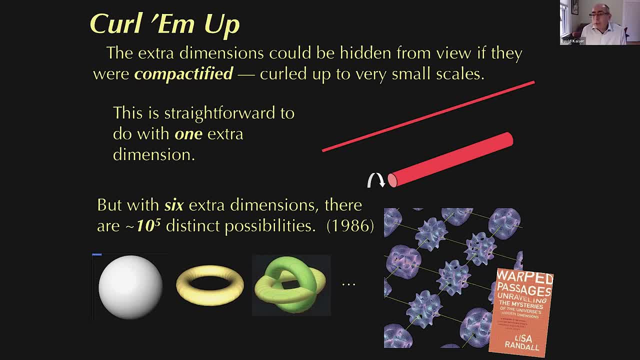 as early as the mid-1980s that that becomes an unbelievably complicated problem in topology that there are estimated to be about a hundred thousand topologically distinct ways to kind of curl up or fold up these six extra dimensions. so at every point in x, y, z, 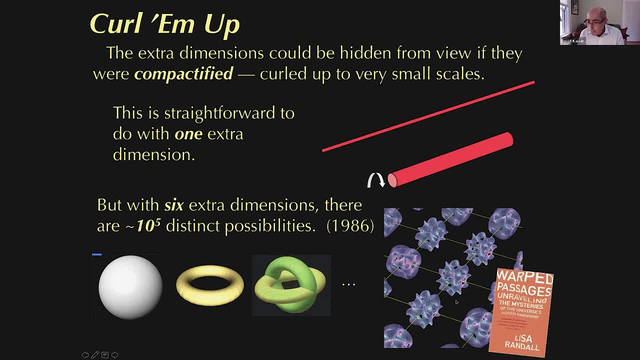 that we could kind of walk along. there will be curled up, maybe in some different pattern, six extra dimensions of space with a characteristic scale of order, the planck scale 10 to the minus 35th of a meter, and yet the actual curling up, the shape of it, really the topology could be different. 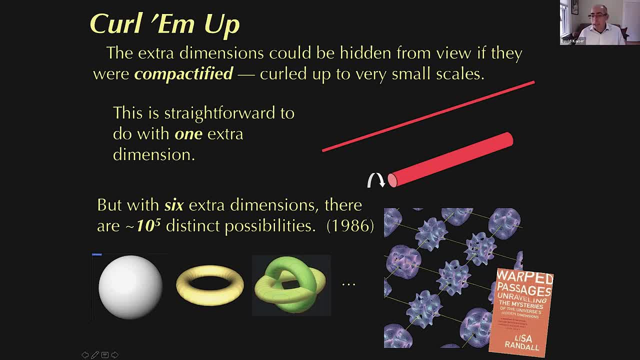 from one location to the next. so people start talking about these so-called kalabayau manifolds, a topic of great interest to pure mathematicians, and some of the string theorists wondered: would that kind of topology accounting work well, and would it be useful for making sense of these shrunken down, compactified dimensions? 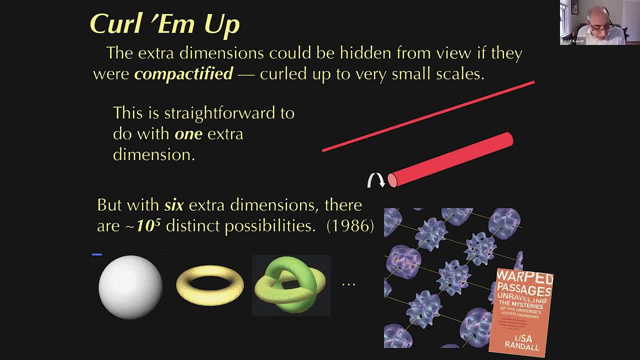 my next uh book club suggestion is a lovely book by a colleague, lisa randall, who's uh teaches at harvard- she used to teach at mit uh, but harvard um convinced her to move all the way across campus- and a really lovely book called warped passages which lisa walks through. some of the kind of 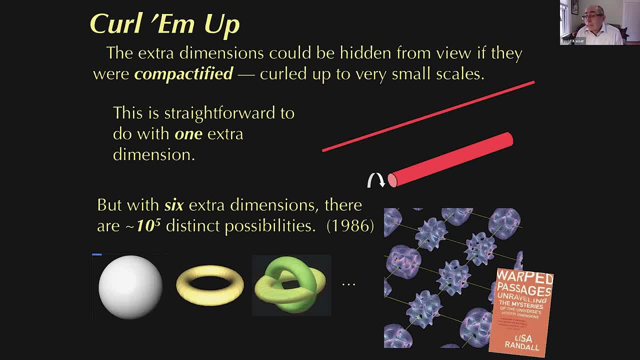 reasoning behind these extra dimensions of space, what are different ways to try to make them go away from our everyday experience? so she, she plays that, i think, really very nicely, and i think it's really interesting to see that the first main conceptual approach to these extra dimensions is curl them up, even though it turns out that's pretty complicated to do. 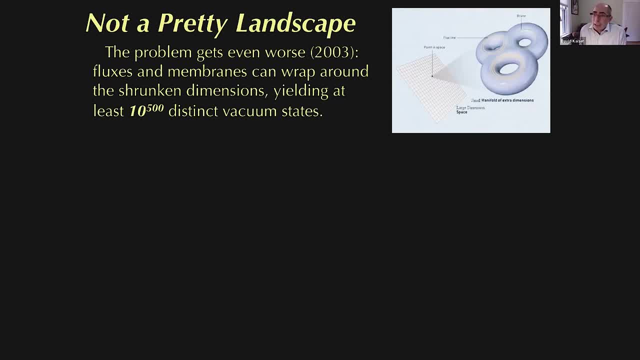 it got even worse. uh, i would call it worse. it got more complicated in the early 2000s and we're getting kind of close to where we are today. people begin. other string theorists began to realize you don't not only have to worry about the actual kind of dimensions of space which can be topologically. 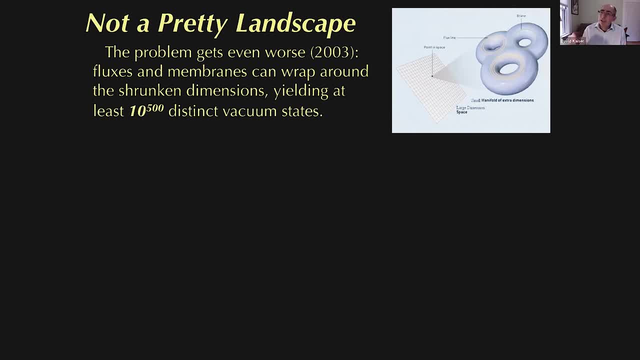 complicated in those so-called kalabaya manifolds, but you actually have to worry about self-consistent configurations of states and how it's going to play out. you actually have to worry about not just these strings but also, say, these strings within and among those dimensions, so you don't 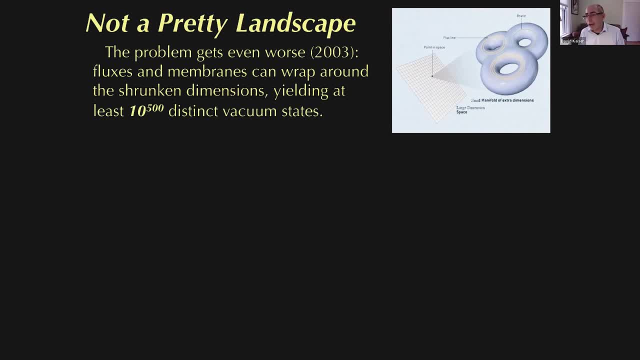 only have topologically distinct configurations of geometry. you actually have some physical degrees of freedom kind of dancing around them and, as you can imagine, you get quite a different um solution if your string is wrapped around a sphere versus if it's wrapped around a taurus versus if it's 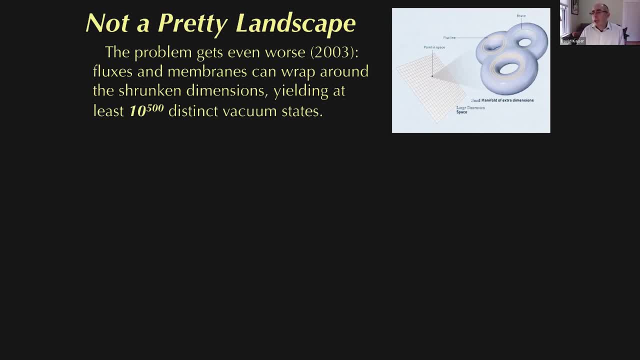 wrapped around a kind of three tours or whatever else. so when they began counting up, the actual theory states, we worry not only about the geometry of the dimensions of space-time, but actually how these physical degrees of freedom, these string-like states, could be distributed within and among them. 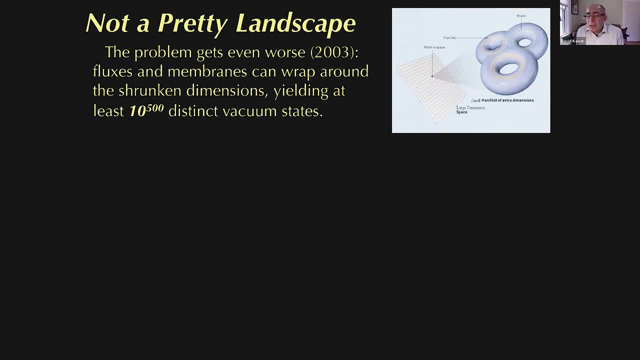 they came up not with 10 to the 5 100 000, they came up with 10 to the 500, which is more than a rounding error. so they began to be concerned that there seemed to be 10 to the 500 distinct low energy string states: 10 to the 500. i won't ask for a show of hands, but it's pretty hard. 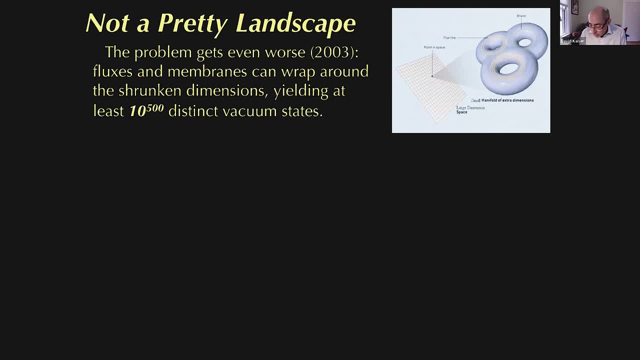 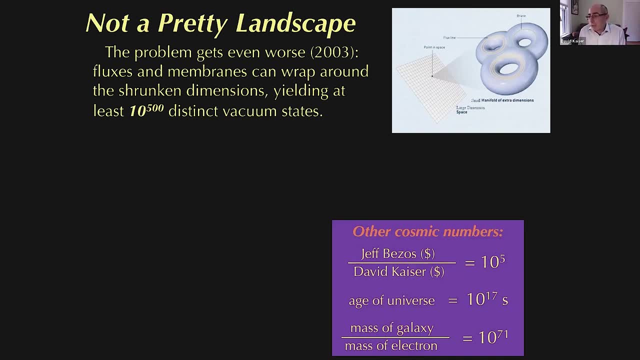 to come up with numbers like 10 to the 500. i've tried. let me give you some of my mundane examples. if internet accounts are to be believed, then jeff bezos has 10 to the five dollars for every buck that i can lay claim to, and that means leveraging everything. sell the house the kids never go to. 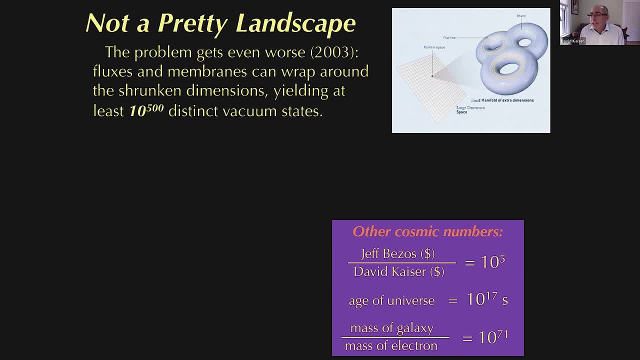 college, forget the car. every single cent i could rub together. bezos has more than a hundred thousand for every dollar i could scrape together. so like that's either impressive or depressing. it's mostly depressing, but 10 to the 5 is nowhere near 10 to the 500, right okay. so now let's go cosmo, let's take the whole universe, let's put 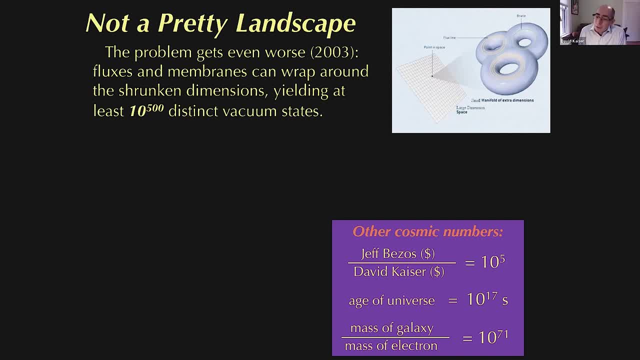 the universe to work for us. if we try to measure the age of our universe in seconds, we get a measly 10 to the 17. if we're a little fancier and say let's enter the age, let's measure the age of the universe with the shortest measurable unit of time that that has been measured so far in quantum. 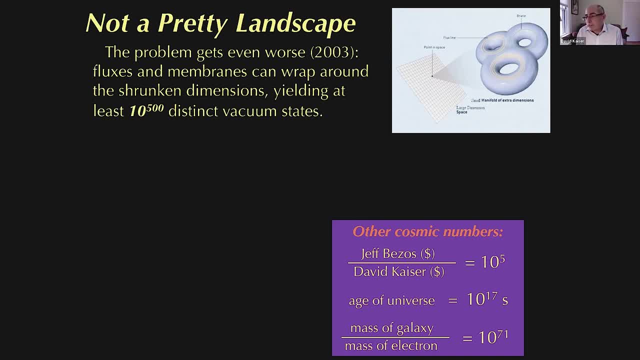 optics, that's about a femtosecond. it's the end of the minus 15th of a second. that only gets us to something like 10 to the 32 we're still scraping. that's nowhere near 10 to the 500. now let's compare, say, the mass of the. 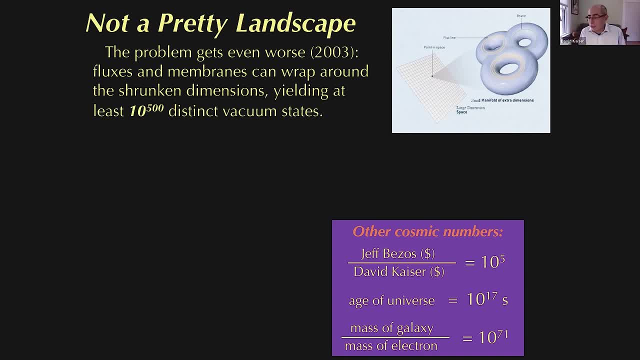 entire milky way galaxy to the mass of a single electron. it's really big. it's a big galaxy. electrons are tiny. that ratio is 10 to the 71. you get the idea right. 10 to the 71 is basically equal to zero when we're comparing it to a number like 10 to the 500. so what became? either interesting or 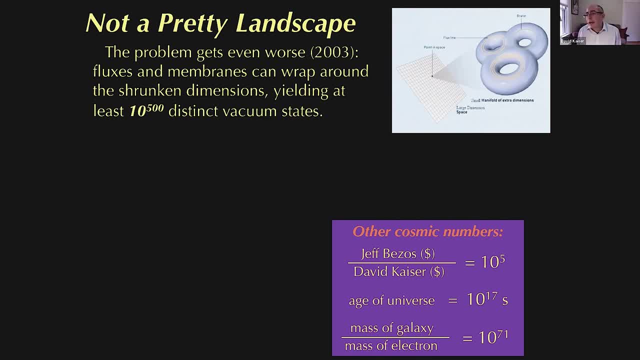 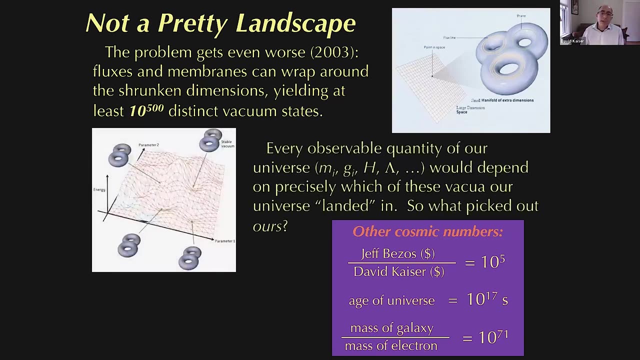 horrifying to me. i think horrifying in the early 2000s was in a number of these string theorists realized that there were unfathomably large numbers of what looked to be self-consistent low energy string states within, uh, these strength super string theory models. now, why should we care? 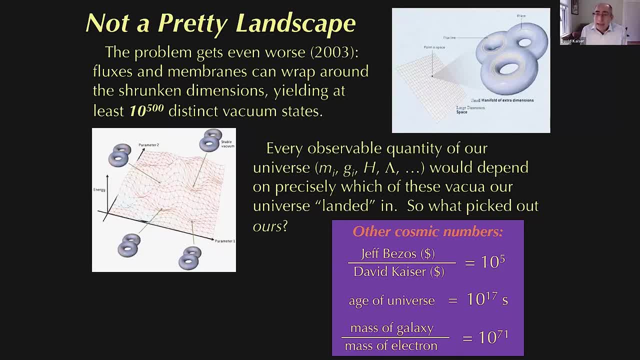 because at least, within this super string theory framework, every single quantity that we with which we might try to characterize our universe, the masses and charges of every kind of particle, every electron quark, glue on everything, uh, would depend in principle on the particular one out of those 10 to the 500 string states in which our universe happens to um to land. so even for 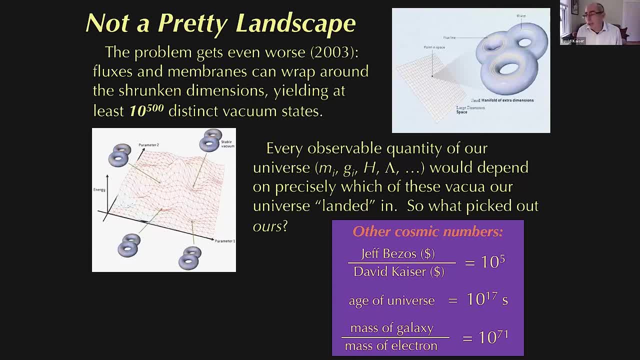 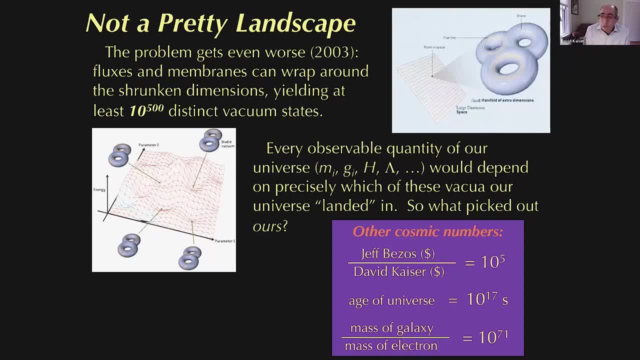 rate at which galaxies recede from each other, or things like the value of so-called dark energy, or the cosmological constant, even the bulk properties with which we try to characterize our universe at large. each of those numbers, the actual quantitative value would, in principle, depend on which one of 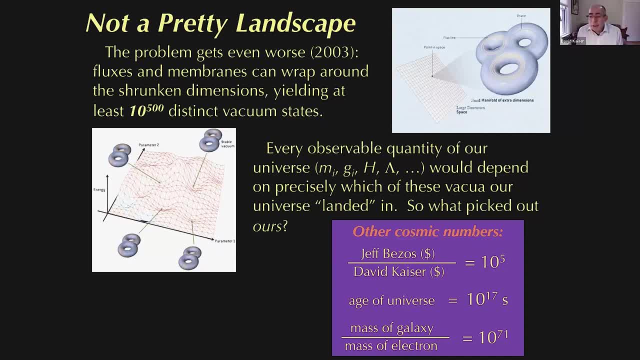 the out of these 10 to the 500 distinct string vacuum states. so how do we make any predictions, or how to make any sense at all, empirically or quantitatively, out of the universe we live in, either from data like the large hadron collider? 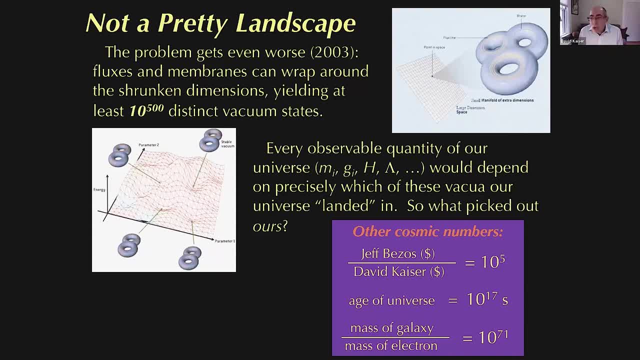 or from all our astrophysics, cosmology, if suddenly we have no way, or at least no practical way, it seems to, to relate this kind of seemingly fundamental description of nature at these very tiny string scales to things we can actually probe, measure and wonder about. that became. 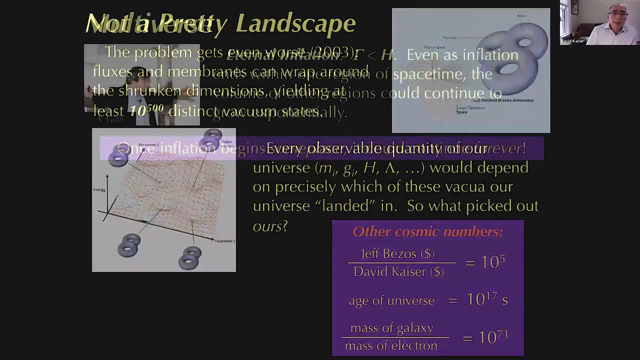 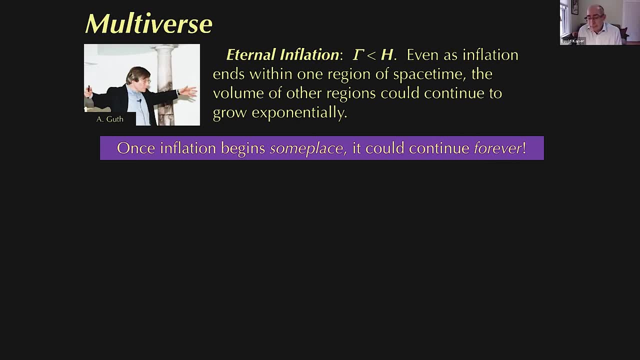 this new twist in the string theory saga in the early 2000s. so here once again is alan alan guth. that idea about the string, so-called string landscape, these 10 to the 500 equally self-consistent low energy states of string theory, that set of ideas kind of collided with some some. 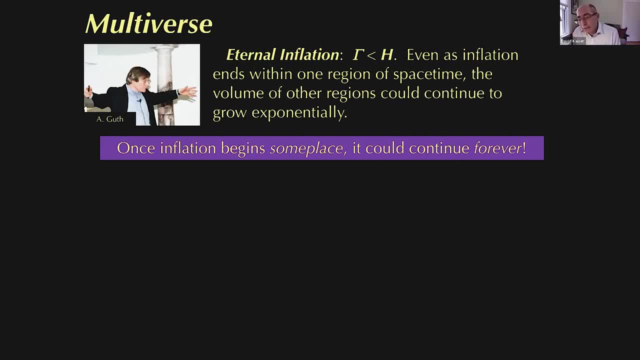 cosmological ideas which had first been developed quite independently. so we talked in the most recent class session about cosmic inflation, a set of ideas that i dearly love. it turns out early on in thinking about inflation, people including alan and paul steinhardt, and actually a number of folks- 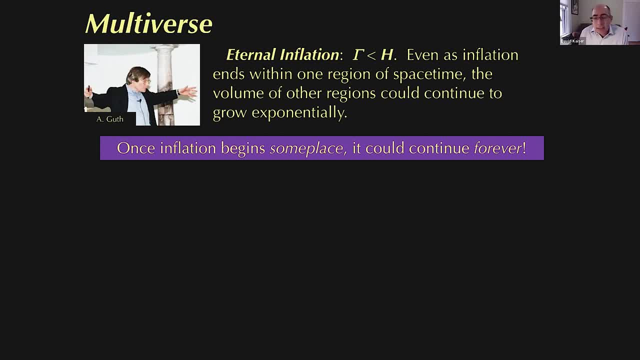 we mentioned briefly last time, audrey lindick began to recognize something curious about these inflationary models. basically, each inflationary patch, each inflationary phase, let's say, has some kind of natural lifetime. it's almost like a radioactive decay that the configuration of those higgs-like fields, that 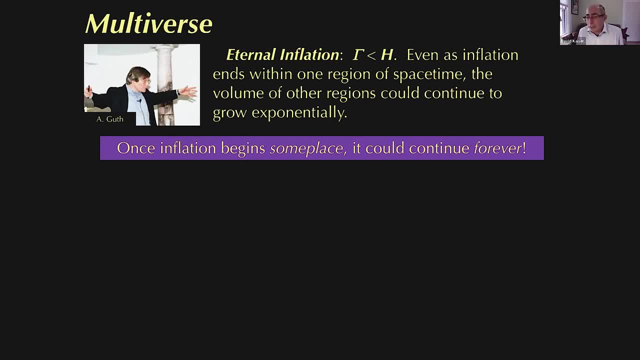 temporarily drive this very rapid, accelerating expansion of space and time. they have a kind of natural decay or natural lifetime. it's not infinite. in fact we know it was a very short-lived period of inflation and in fact we can kind of estimate for a given model what the kind of almost like a 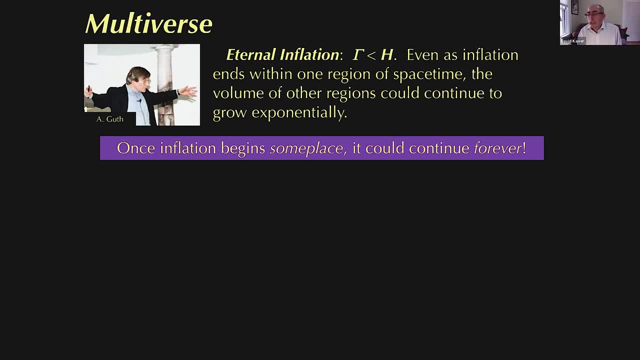 half-life would be, for how long that phase is expected to last. it's probabilistic, it's a quantum mechanical process, but it's very similar to calculating a kind of radioactive half-life. and what became clear is that for many, many, many of these models that otherwise seem to match predictions on our 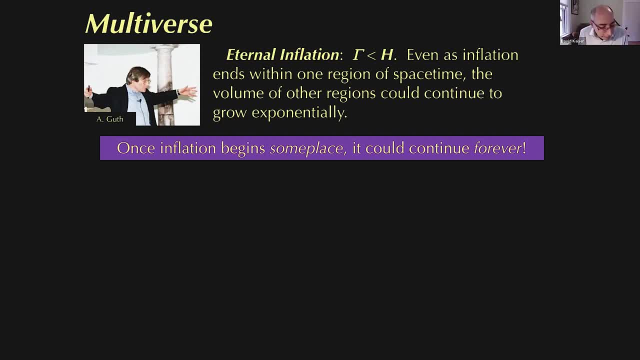 sky beautifully they're. they're models that seem to have many nice features, that the the kind of half-life, the decay rate, so to speak, is actually smaller than the expansion rate, that in regions that have not yet decayed out of that phase, space should be stretching exponentially quickly, more quickly than the rate at which 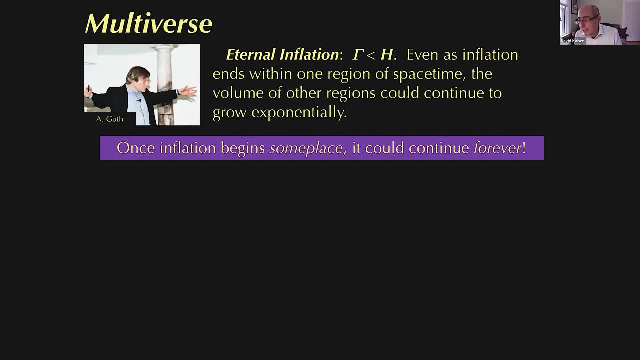 neighboring patches of space will fall out of that inflating phase. this became called eternal inflation, and the idea is that at least at least seems self-consistent to suppose, based on what we otherwise know, that if inflation begins anywhere in the universe, it never stops. it will. 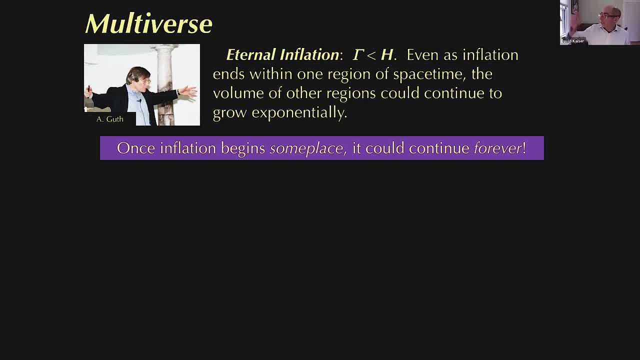 stop at that location. it's not inflating for us right now. it'll stop at that location, but there'll be some other regions of space that would 자신—always will continue to inflate andantesett�– tradicional windtimes More øu卓 course that would position itselferved at the Halloacci shear conditions. 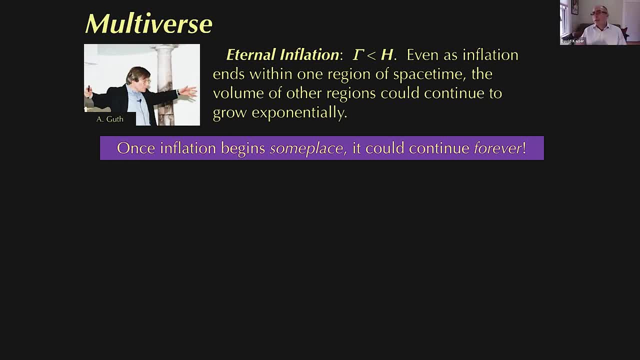 time that are still growing exponentially quickly, And that's because there's this sort of competition between the kind of rates for any given location in space to fall out of inflation. that's the kind of capital gap, the kind of lifetime of inflating phase and the rate at which the volume of some 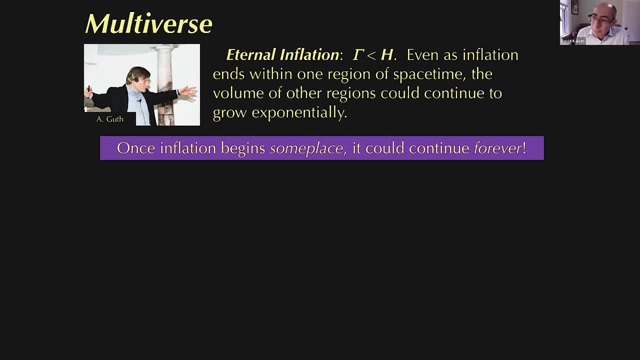 neighboring region continues to grow. So, even though it's perfectly self-consistent for our universe that we see around us, our observable universe, not to be in that inflating phase right now or to have fallen out of the primordial one for all we know, it looks more likely than not. 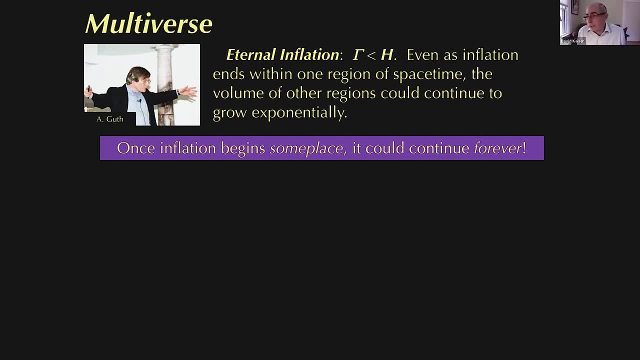 at least in this scheme, that some regions so far away from us we haven't received even a single light beam yet. they could still be in an inflating phase. And that could happen forever, because when that neighboring point falls out of inflation, some other volume of space will grow quicker still. 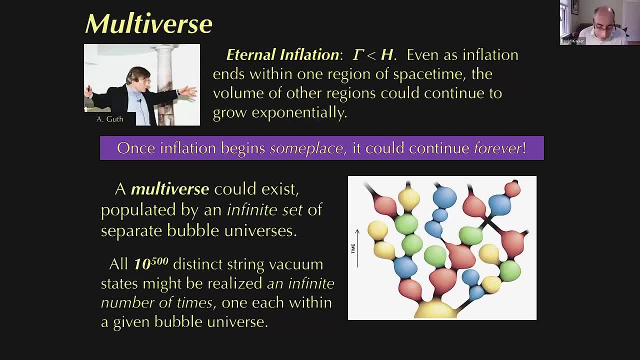 So that led to this idea that Andre Linde in particular really championed, and Alex Vilenkin and many scholars who were interested in cosmology began wondering about a so-called multiverse. Could it be that our observable universe, everything we've seen? 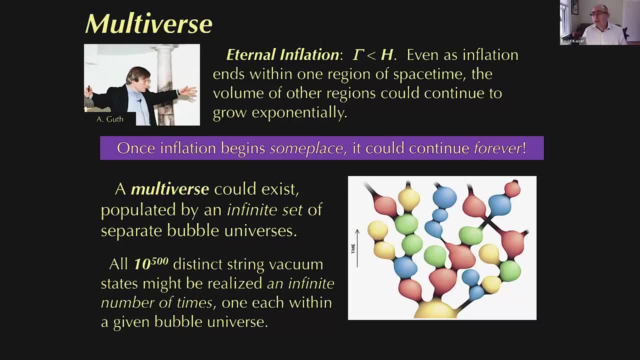 everything we could measure, the CMB and all the rest. is that actually just one kind of self-contained region of space and time within an arbitrarily larger region in the midst of which other patches are still inflating exponentially and others have fallen out as well? Could you have an infinite? 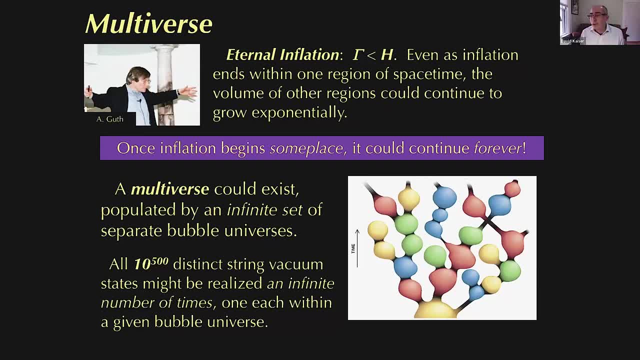 multiverse If inflation never ends, if it really could happen towards T, would you be able to build a multiverse? if we had an infinite volume of space? If we could do that, if we had a world where T equals infinity, then in principle we would have an infinite volume of space. 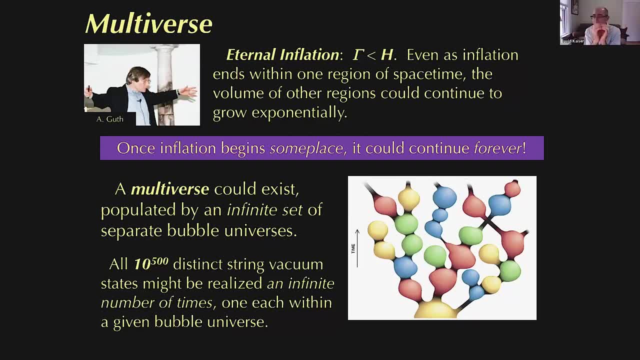 We occupy, we can observe around us a very tiny, self-contained bubble within an infinite bathtub. We're like a soap bubble within a bathtub that actually is infinitely large in volume. So that was the idea of eternal inflation, suggesting not proving, but suggesting there could exist a multiverse. 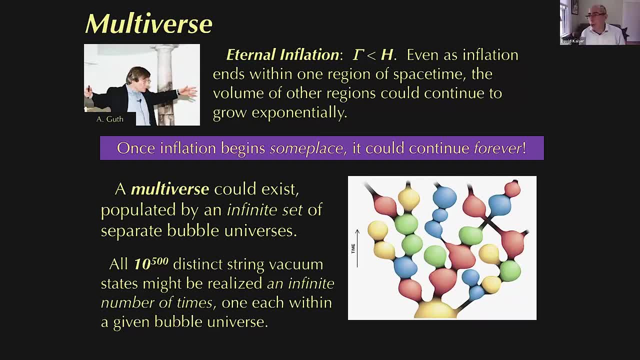 a huge collection of pocket universes well beyond our own and gather information, And that idea then kind of collided with or was merged with this series of ideas from string theory in the early 2000s, and particularly the so-called string landscape. If there are 10 to the 500 distinct self-consistent. 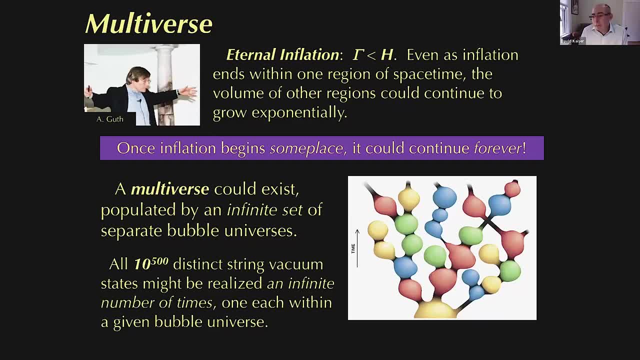 low energy string states and you have an infinite number of chances for them to be realized, because you have an infinite multiverse within which you can have these self-consistent pocket universes constantly inflating and then falling out of inflation while neighboring regions inflate. 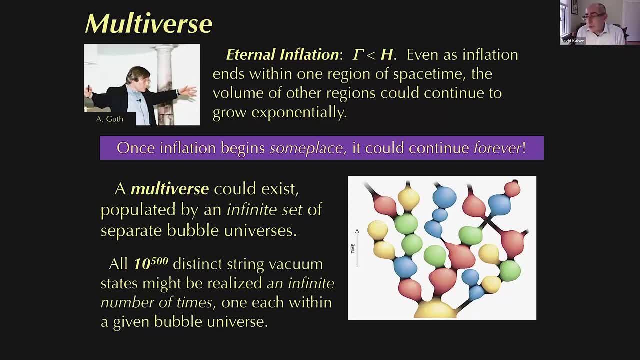 could it be that every single string state is actually realized an infinite number of times? So 10 to the 500 is big. it's infinitely smaller than infinity. right, You can see where. I hope it's clear that I'm not endorsing these ideas. 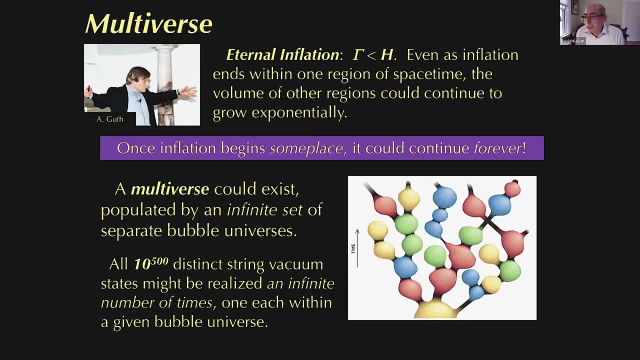 I find these ideas pretty unusual is the nicest way I can put it, But I can at least appreciate why so many of my colleagues have been led to wonder about them. You can see the kind of thought train that leads to this as the next question. 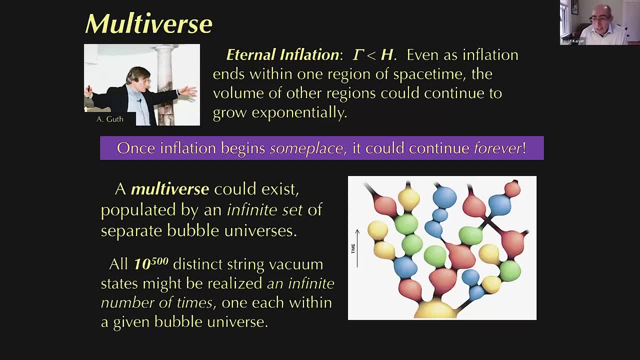 or tentative conclusion. You can also see how it's getting harder and harder to get the kind of reinforcement of the input or the kind of dialogue with empirical data, unlike, say, the early days of quark physics. So I hope I can at least convey to you. 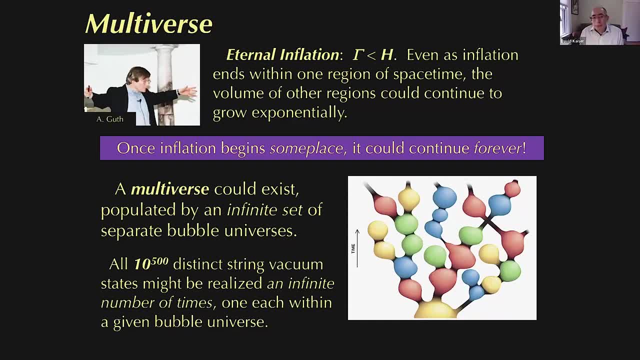 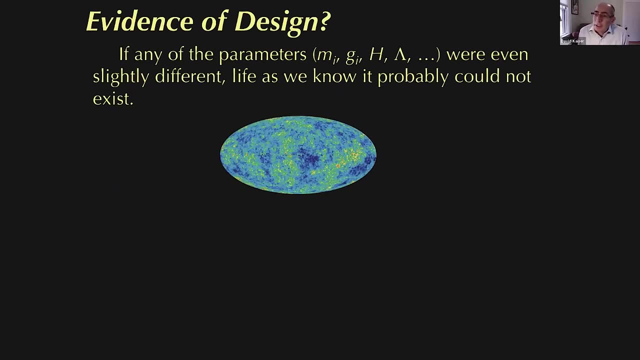 as a collegial neighboring, skeptic why people ask these kinds of questions, right, This kind of merger of ideas from string theory and from things like inflation. Okay, so if every one of the parameters that we measure empirically the masses and charges of elementary particles 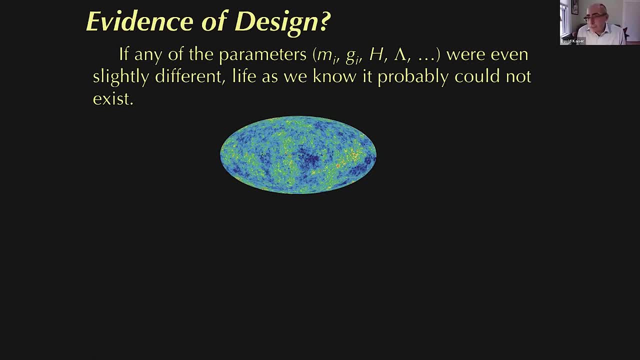 larger properties, like the Hubble expansion rate. if they were slightly different, people began to wonder: would the universe as we know, would our observable universe, have shown anything like the pattern of evolution that we have actually empirically measured? Could there have been galaxies that actually formed stably? 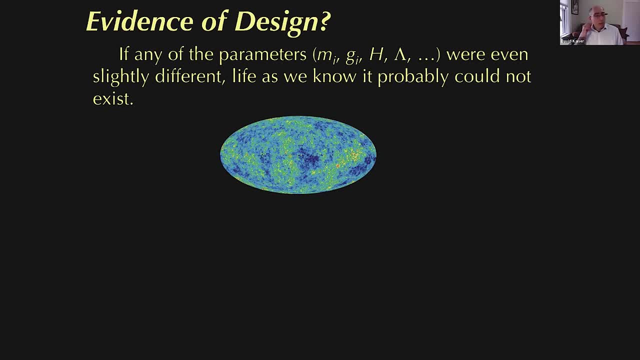 if the expansion rate were slightly larger. The idea was, if the expansion rate were actually a little bit larger in early times, could galaxies? galaxies never have overcome the kind of expansive pull of gravity where they've never coalesced to be gravitationally self-bound? 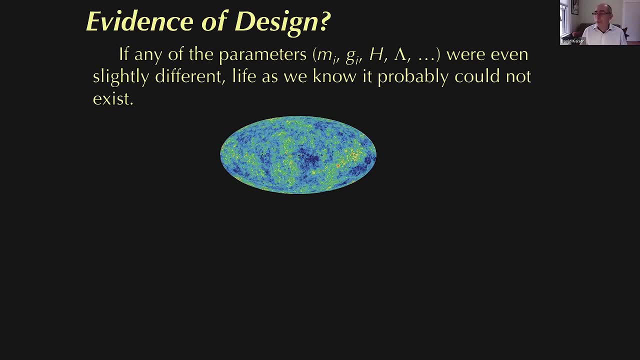 If the expansion rate were slightly larger than it happened to have been in our observable universe, maybe there would never have been galaxies. If there's never galaxies, could there be things like stable solar systems or planets? You can play this game all the way down. 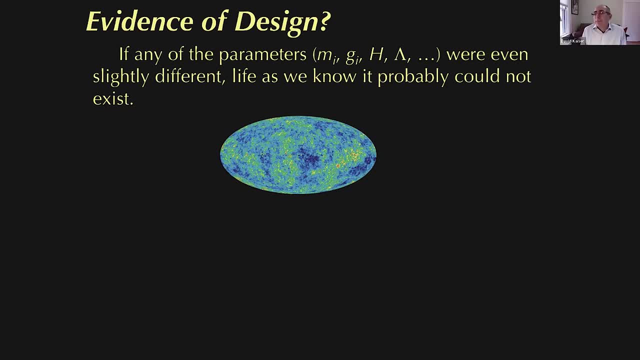 Could there be life as we know it If any of these seemingly fundamental parameters have been slightly different from the values that we happen to measure? Now it turns out historians can remind us that's a very old argument If that sounds familiar, especially to our historians. 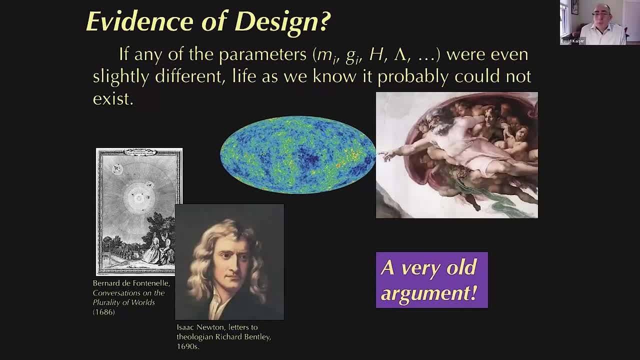 of science in the group. you're right, That idea that if any parameters of our environment had been slightly different then we wouldn't be here, that goes back, at least in a kind of European tradition, at least to the late 17th century. 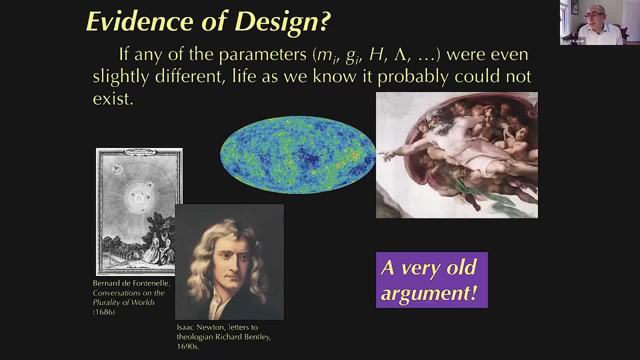 I'm sure we could find clever anticipations even earlier, But some of the most famous articulations of that come from this very charming book by Bernard de Fontenelle, a French natural philosopher, translated as Conversations on the Plurality of World. 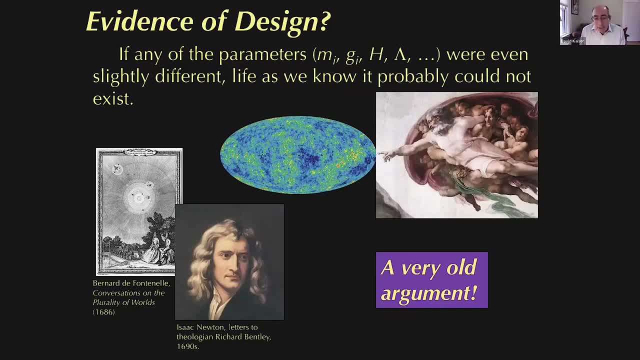 It's still in print. you can buy a cheap paperback. Very soon after that, Isaac Newton was writing letters privately to a theologian friend of his. They were published soon after Newton's death, his friend Richard Bentley, where he was musing on this as well. 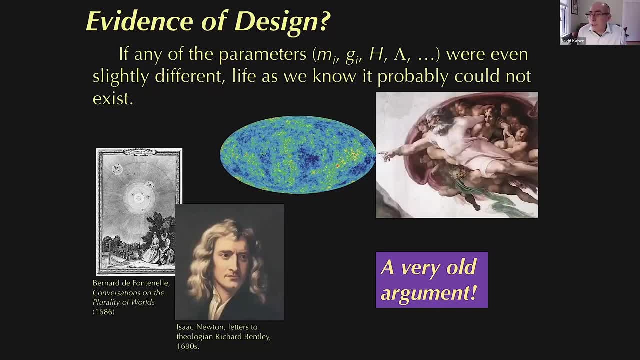 To these folks, this kind of fine tuning argument was, to them, absolute, incontrovertible proof that God exists and to them that was a kind of- you know, fairly recognizable Christian God of the Bible. in their reckoning, The idea was that God must have made the world just for us. 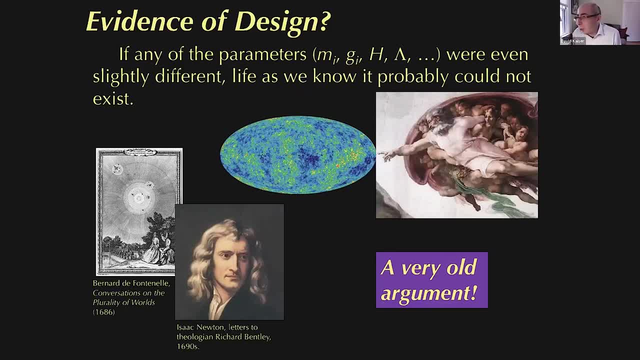 If the earth were slightly further from the sun, it would be too cold for us to have flourished. If the earth were slightly closer to the sun than it is, it would be too hot. These kinds of fine tuning arguments have a very 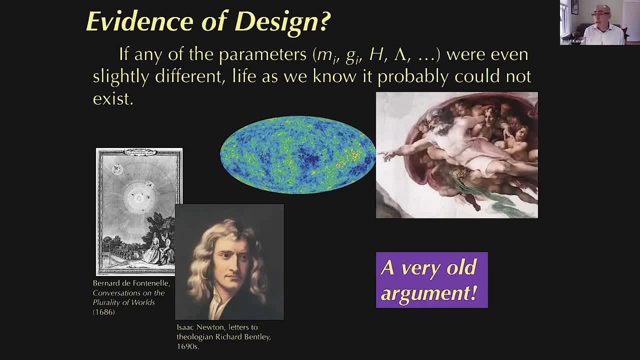 very long history in astronomy and astrophysics, And for a lot of the early advocates this was taken as literally proof of a kind of biblical story of Genesis that God made the universe literally for us. So is that how these later string theorists formulated? 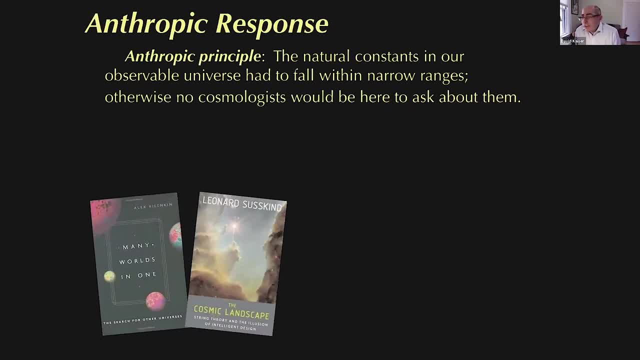 Not really like, not at all. So two-thirds of that fine tuning argument sounds just like what Isaac Newton or de Fontenelle had been saying 300 years earlier. But some of these later, more recent advocates give it an interesting twist. They appeal not to a religious or a kind of supernatural. 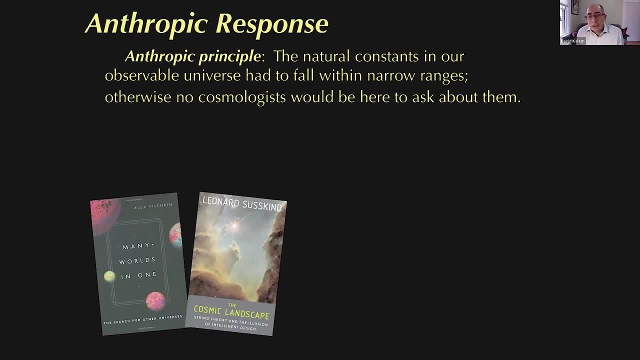 force. they appeal back to us in something called the anthropic principle which, again, you might've read about. The idea is, I think, is that you know the idea, as I've mentioned before, as even Fontenelle and Newton had recognized. 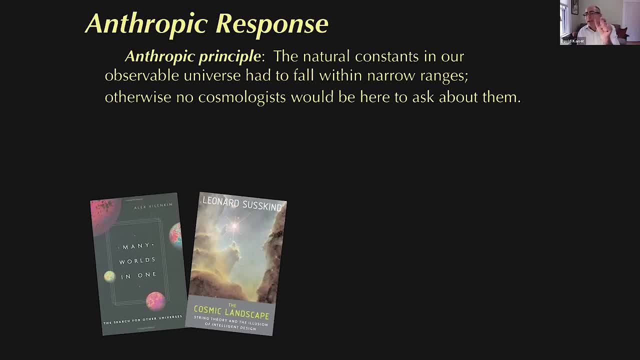 is that the natural constants have to be within, seem to have to be within, very specific and actually narrow, fine-tuned ranges for anything like life as we know it to have survived, to have evolved and survived. So if those parameters were not within those 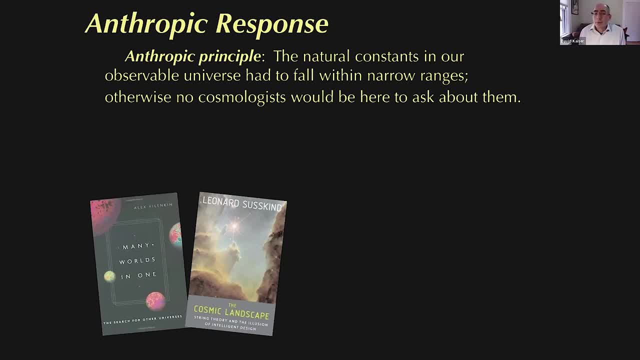 finely tuned ranges, then we wouldn't be here to ask these questions. So it comes back to what's the precondition for cosmologists, or any humans at all, to be asking questions about? you know the universe. And so again, here's some other very nice popular books. 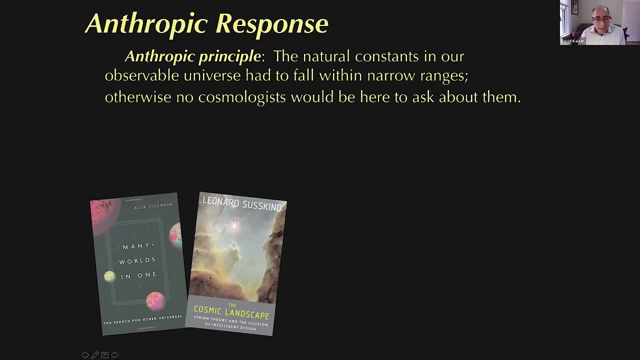 that came out around 15 years ago or so, One by Alex Vilenkin, who teaches at Tufts- he's very nearby, a real pioneer in this work. Another book by Leonard Susskind, who teaches at Stanford, And they're both discussing these more recent developments. 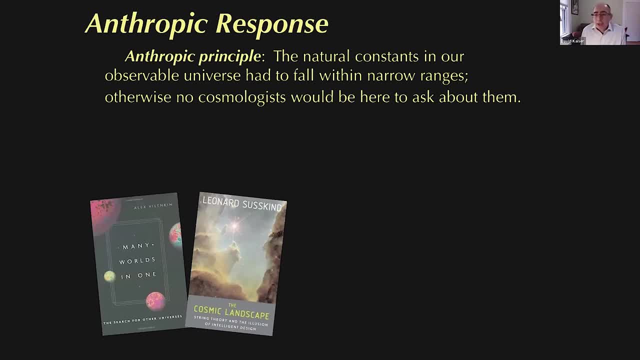 when the string landscape meets the multiverse. And you can see each of their answers are very clearly not appealing to a kind of religious explanation. In fact, they say the basic structure of the argument is if there are 10 to the 500 distinct string states. 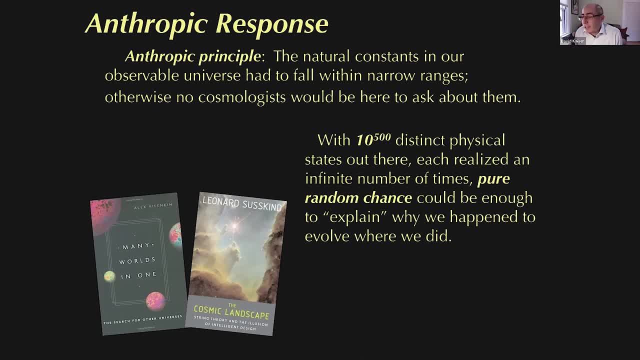 each of which has an infinite number of chances, because this eternal inflation argument, each of which is realized in an actual physical volume of space an infinite number of times, then it just takes pure random chance. It's almost kind of Darwinian that we 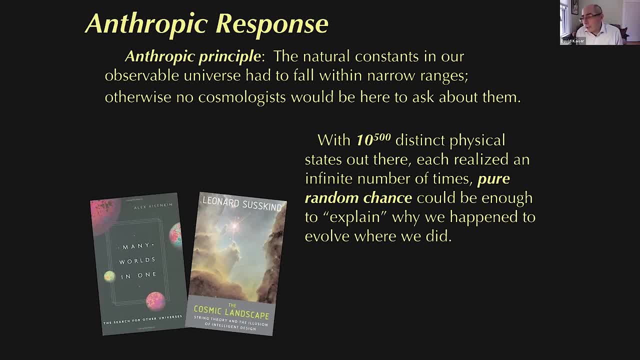 would evolve where we are to measure the constants we do, because we had no choice, That is to say, any difference in those constants which might really be happening arbitrarily far away, people like us wouldn't have evolved there to ask those Questions. So the explanation why: 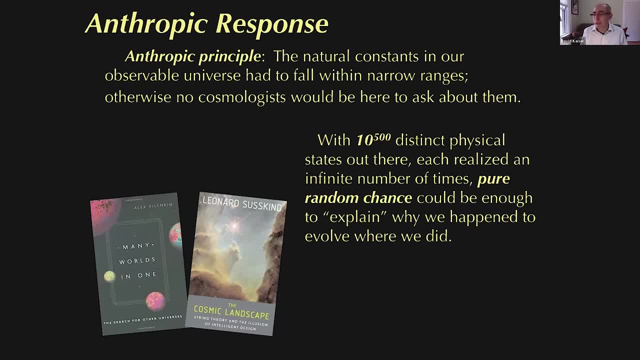 do we measure this value for the expansion rate or that value for the mass of electron? is not, they argue, because we have to know why one special value out of those 10 to the 500 gets picked out, But simply to say they're all out there. 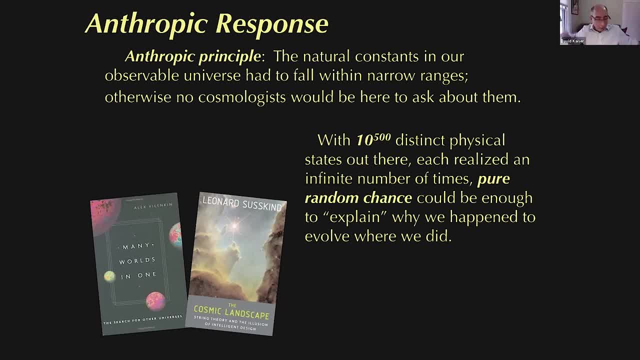 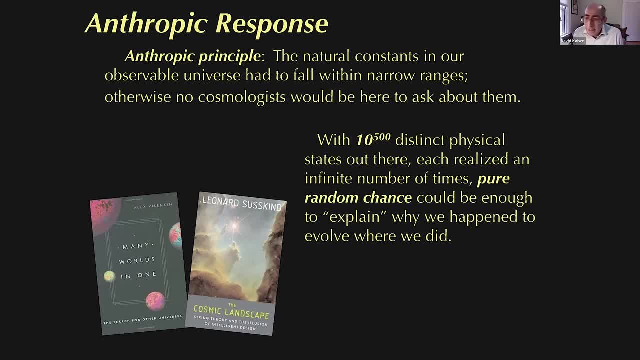 I don't know. I don't know. I think this would be a great idea to run. It's not exactly a great idea, but we might be able to measure the constants, at least as we currently understand it, to have been able to come around to ask those questions. 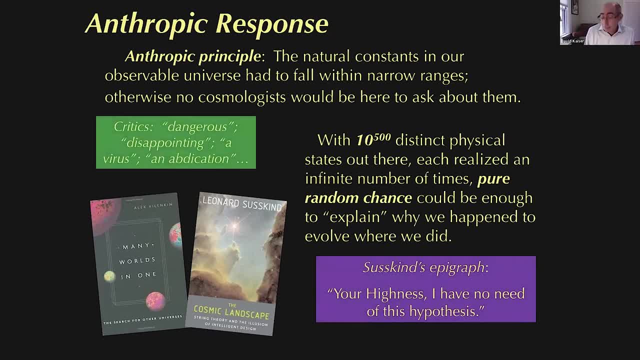 So it's not that you pick out one string state physically, You say we'd only ever be able to measure a certain very small subset. So some critics- and they say critics within physics critics, Nobel laureates within irony theory, for example- 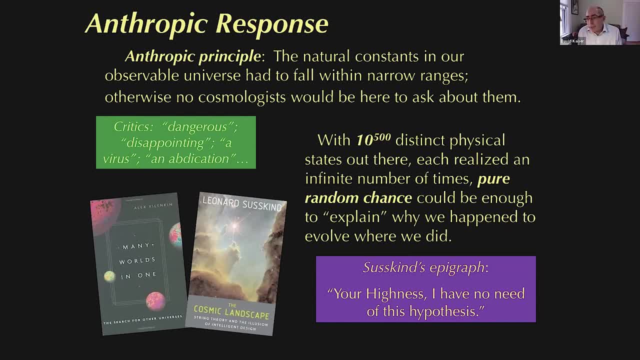 some of them really, really don't like this idea. I personally am still rather ambivalent, to put it mildly. Critics will have called it in print: dangerous, disappointing. a virus really makes me shudder. an abdication of what physicists should be doing. This inspires strong. 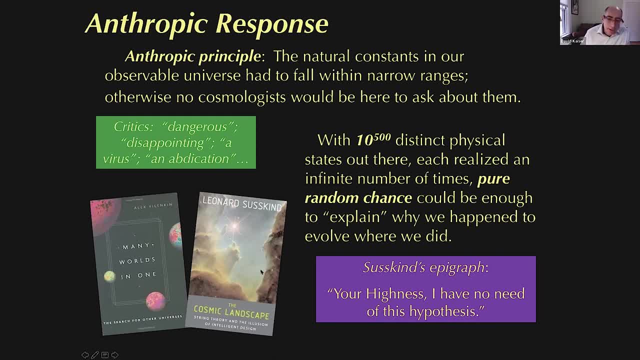 reactions. Lenny Susskind in this book here sort of knows that perfectly well. He's no stranger to making bold statements. So Susskind actually borrowed for the epigraph of his book the famous and probably apocryphal statement from Pierre-Simon de Laplace in answering Napoleon. 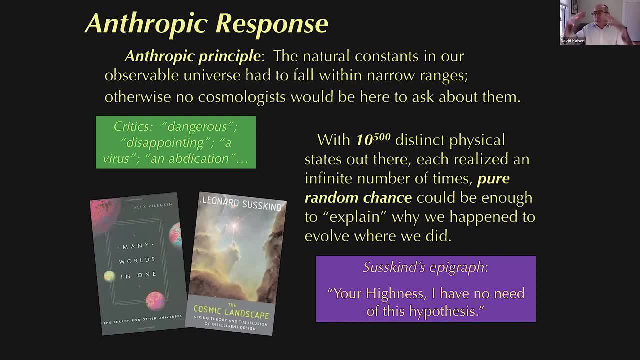 Napoleon was so impressed by Laplace's 18th century kind of Newtonian cosmos. They could account for the motion of planets and comets and everything with such great precision. Napoleon supposedly had asked Laplace: where is the room for God in your theory? And Laplace 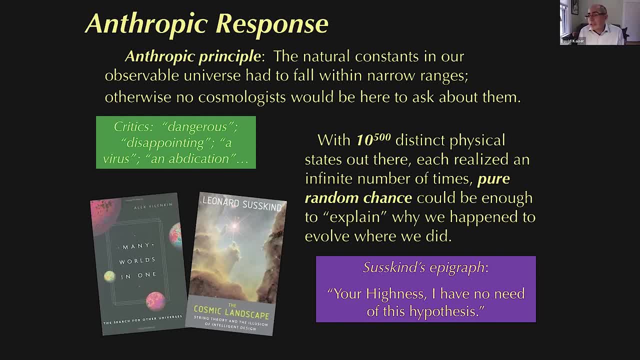 like Susskind says: your highness, I have no need of that hypothesis. He doesn't need, as Newton seemed to need, an appeal to a kind of religious or biblical supernatural force. He says you just have to have 10 to the 500 distinct states and an infinite number of chances. 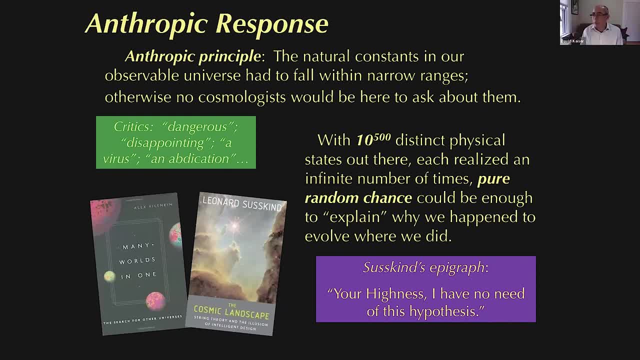 And we would measure around our universe only those that would be consistent with us being there to measure them. Again, I'm not endorsing that view. I find that interesting, although I personally am rather ambivalent. But hopefully you can again see how the kind of chain of reasoning has unfolded. 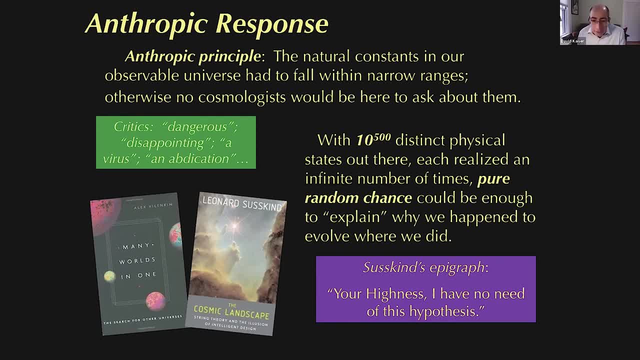 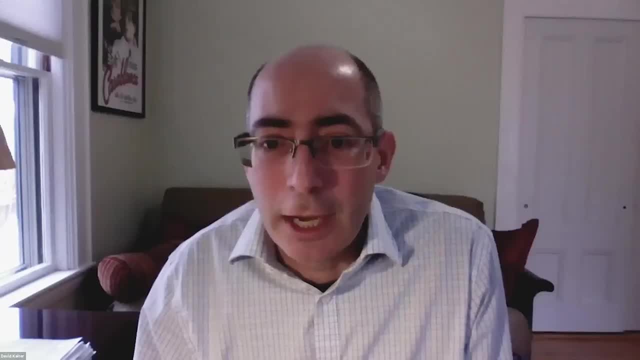 to where this is now talked about with some great attention and inspires great passions among physicists and cosmologists. So let me pause there again. Any questions on the string landscape, on eternal inflation, on anthropic principle, any of these juicy ideas? 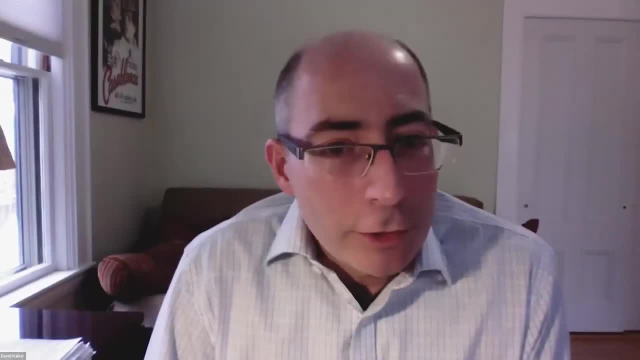 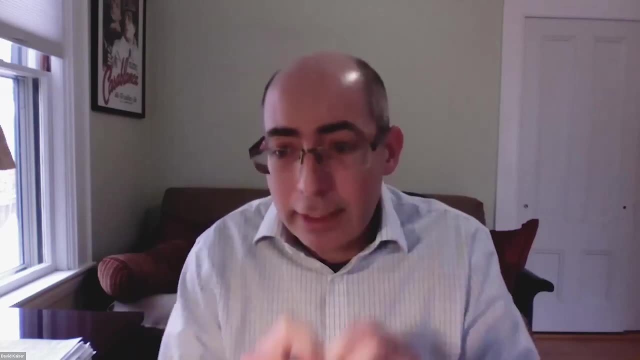 Very good, Stephen. Thank you. Oh, that's a great question. The short answer is, in principle, yes, This could if we had a kind of arbitrarily powerful microscope, if we could zoom in to length scales of order, the Planck length 10 to the minus 35th. 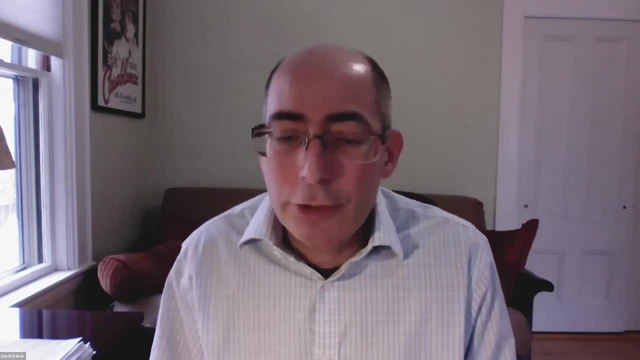 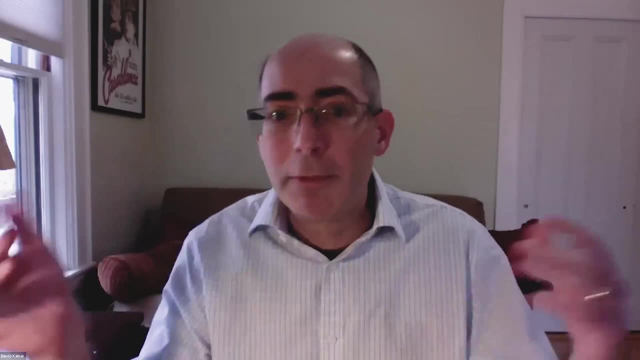 of a meter, which we can, that it could be that each of those was sort of separately realized at each point that we had separately called x equals one, x equals two, x equals three of the mass of the universe. And so in principle, yes, So in principle yes, If we had a kind of 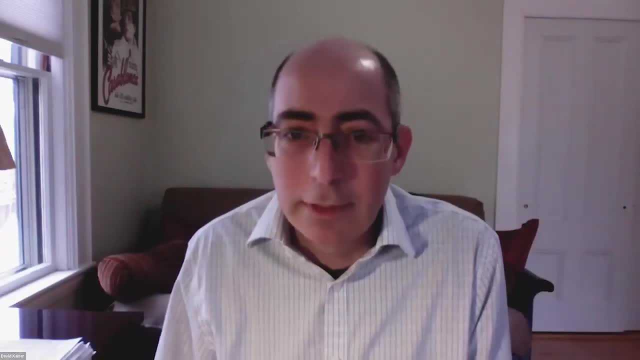 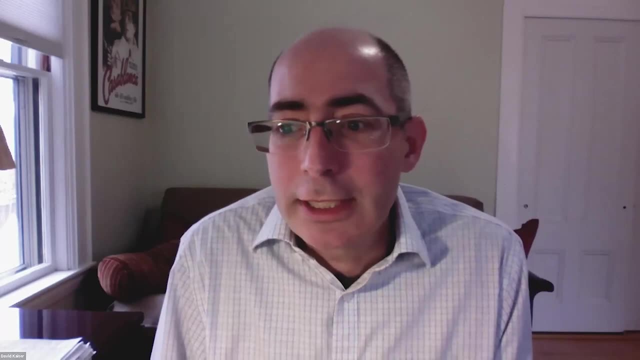 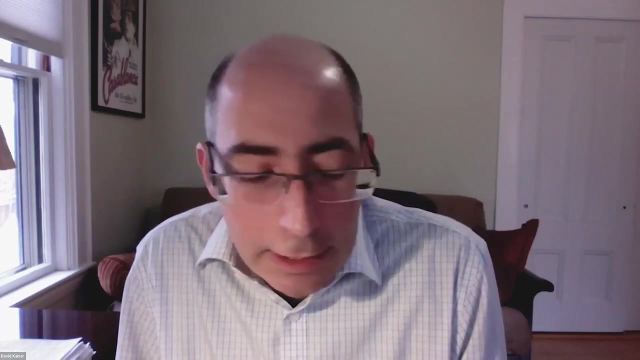 macroscopic space that we otherwise can move around it and measure. So it's not that they must have been, but actually that they could have been, That these are each self-consistent, viable solutions to this complicated set of super string theory equations And, in principle, 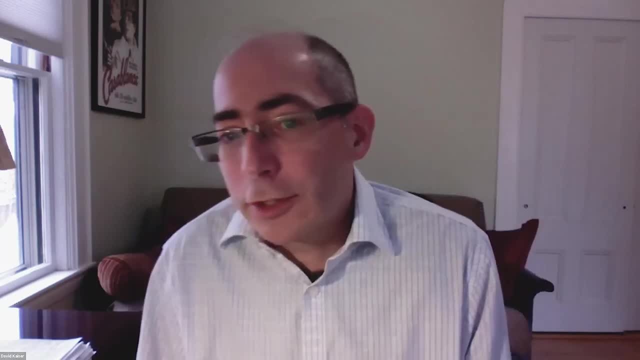 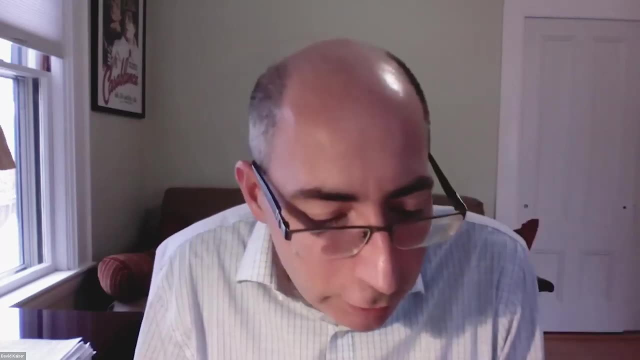 each of them could independently be realized, Or it could be that there's some kind of coherent structure where they all look the same in one region, but then in some macroscopically distant region, some other. So it's not that there's a set of values. might have taken place When the idea gets combined with. the string landscape. it's more the latter, That there are actually microscopic regions where there would have been one of those states versus another, but then something like the Higgs field or an inflation-causing field settles into one of those vacuum states versus another. and then the volume. 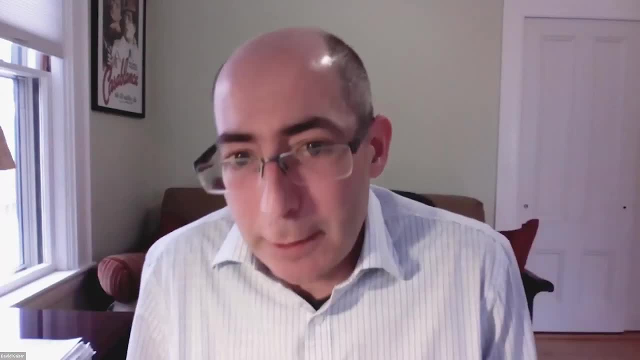 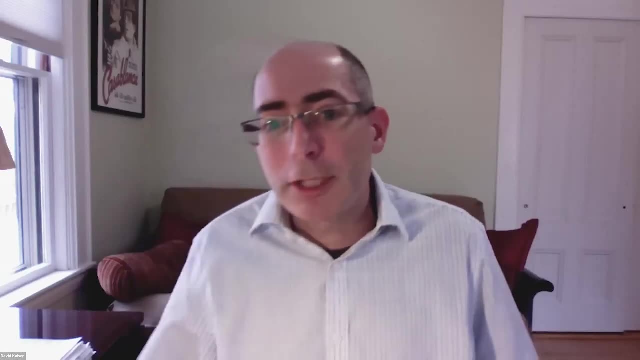 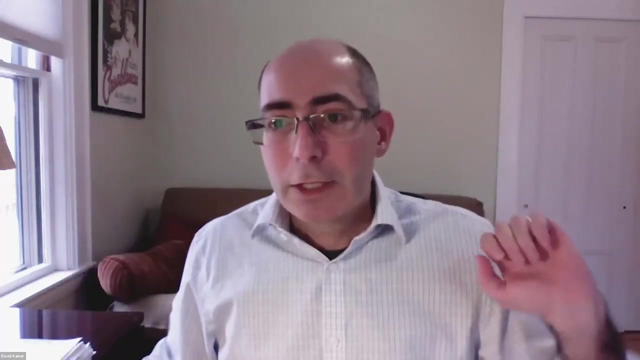 of that space. the three-dimensional volume of that space grows exponentially. So when you start combining the 10 to the 500 with ideas about inflation, you're going to have a set of values that are going to be realized elsewhere. So to the string theorist alone, the idea was each of those could. 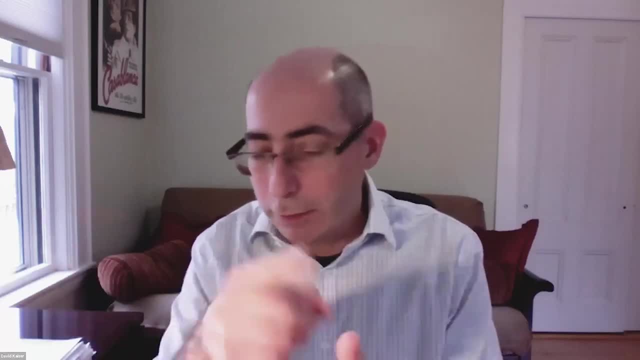 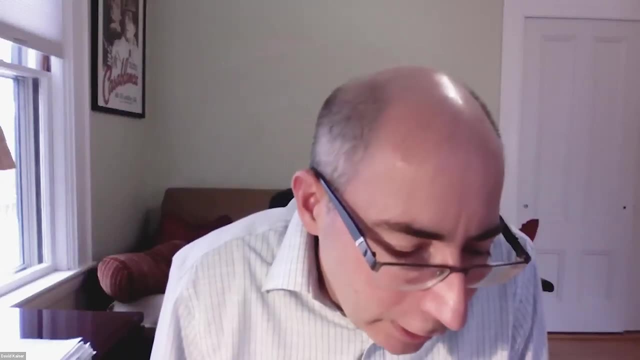 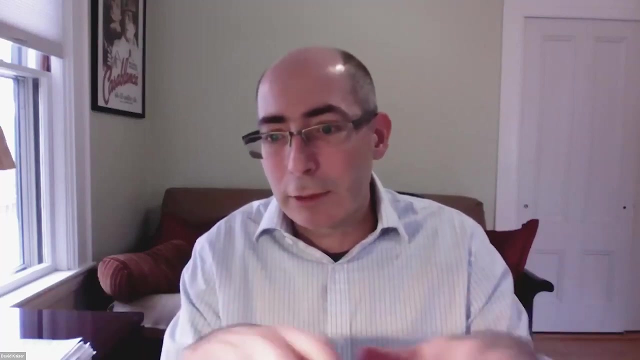 be a self-consistent solution at any arbitrarily small location in the XYZ space we use. But if you start thinking about combining that with inflation, the idea tends to be that all those are near each other, so to speak, at early time, And so if you're going to have a set of values that are 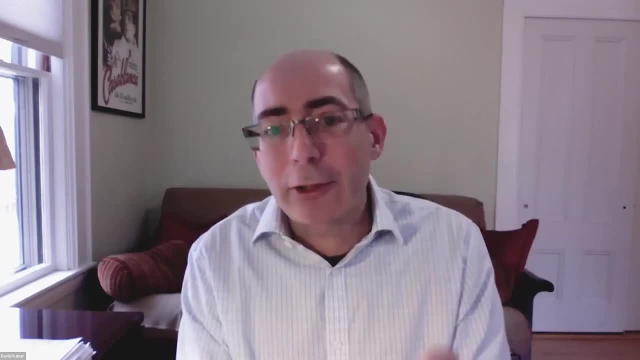 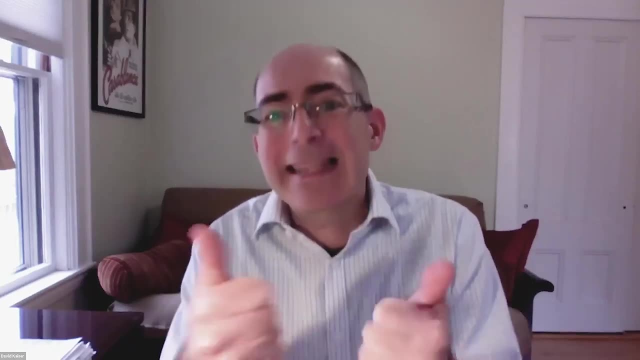 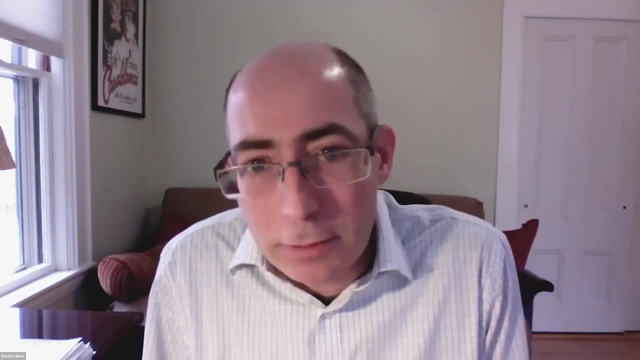 microscopic. you're going to have a set of dimensions, But then whatever's going to start driving a macroscopic inflation, for the dimensions that we live in will actually stretch the space containing that one string state rather than the neighbor. So I guess in an eternal inflation multiverse. 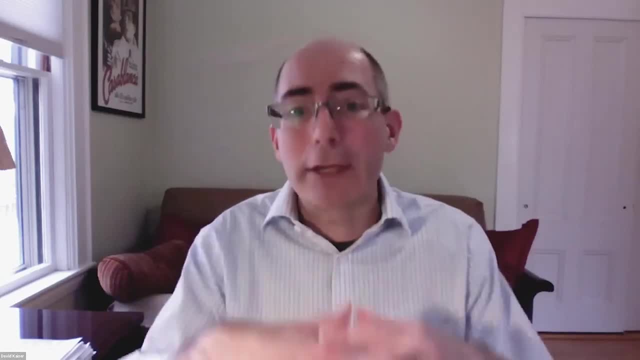 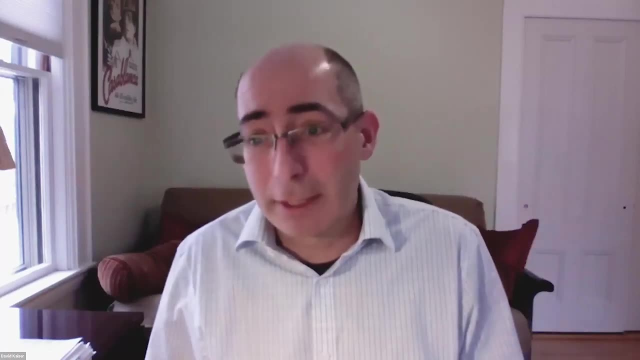 model. I think the idea would more be like we would expect to have a coherence, that if we could zoom in with our microscope we'd measure the same string state within our own kind of macroscopic bubble, even though in principle we would expect to have a coherence. So if we could zoom in with 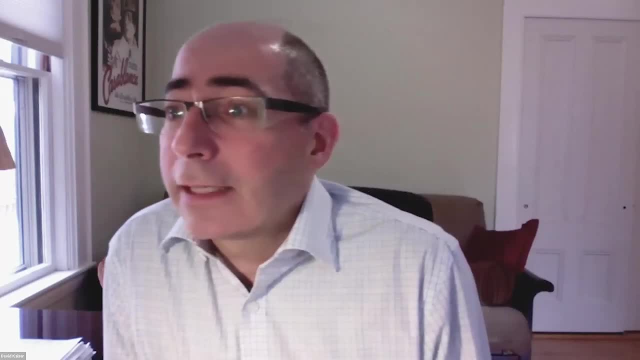 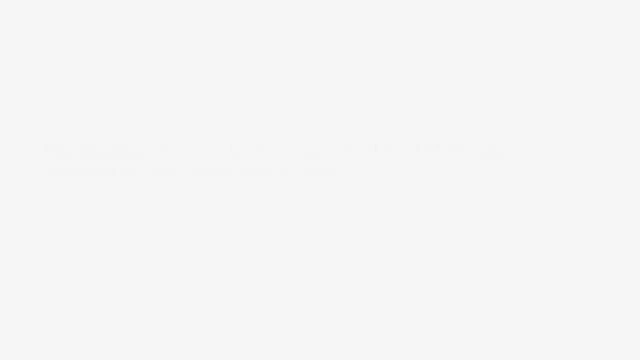 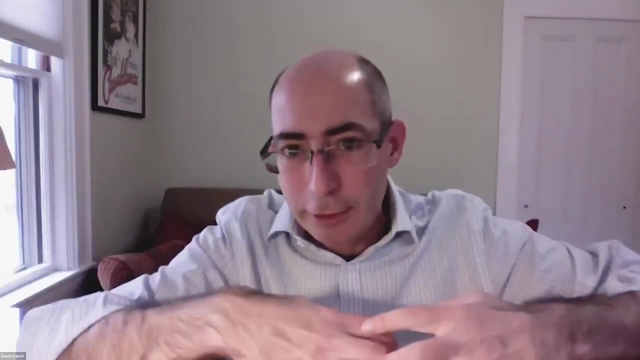 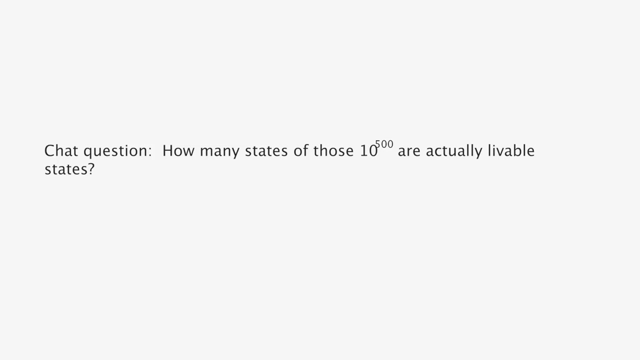 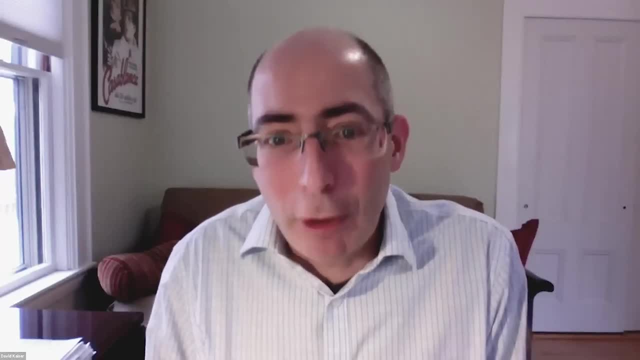 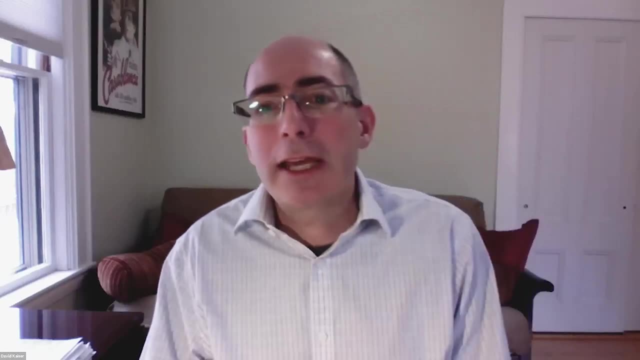 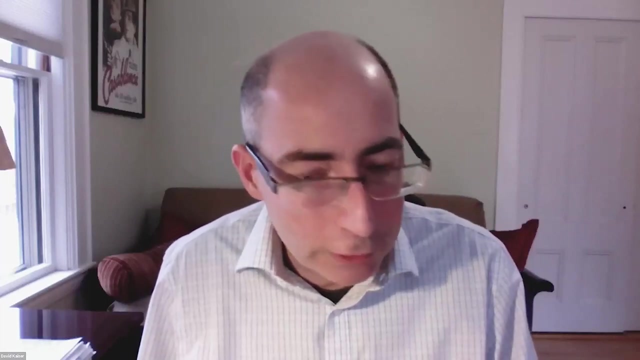 you know, we could sort of we could take what we think we know about the origin of life. what I know about the origin of life is approximately zero, but people look at it more carefully. or even something that's maybe closer to astrophysics, like what would it take for stable galaxies to form and not get ripped apart by a too fast expanding early universe? that's one that people looked at in more quantitative detail. 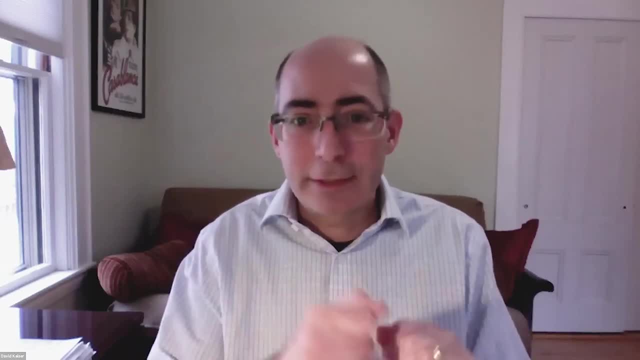 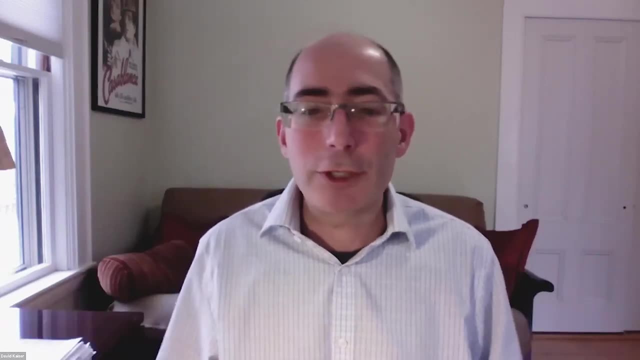 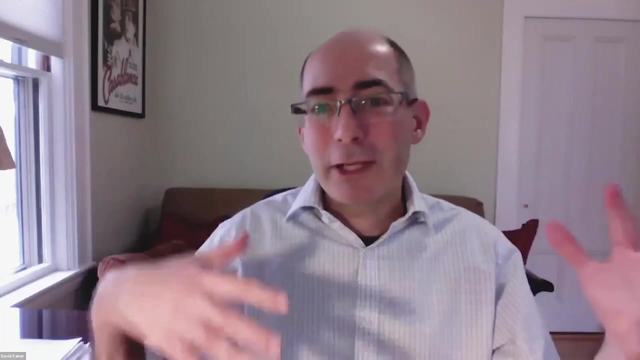 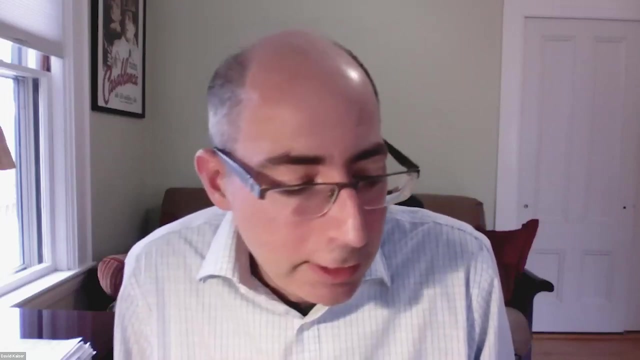 So if you change one parameter, in this case the early expansion rate, you either do or don't get stable galaxies to form. but we have a lot of parameters we could tweak. what if we tweaked the electromagnetic force and the unit strength of gravity and the expansion rate, right? so who's to say, in this multi-dimensional system of constants, even the ones that we know about, then one couldn't find sort of compensating solutions. could we find galaxies formed if we did have the faster early expansion rate? but if we tweaked three-dimensional system of constants, then one couldn't find sort of compensating solutions. could we find galaxies formed if we did have the faster early expansion rate? but if we tweaked three-dimensional system of constants, then one couldn't find sort of compensating solutions. could we find galaxies formed if we did have the faster early expansion rate? but if we tweaked three-dimensional system of constants, then one couldn't find sort of compensating solutions. could we find galaxies formed if we did have the faster early expansion rate? 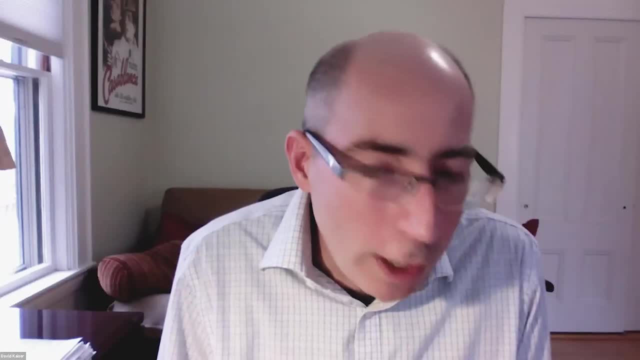 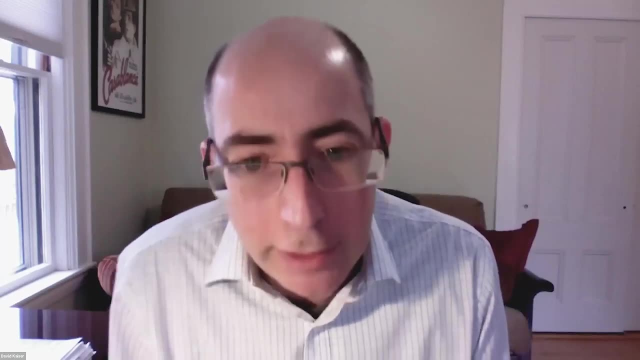 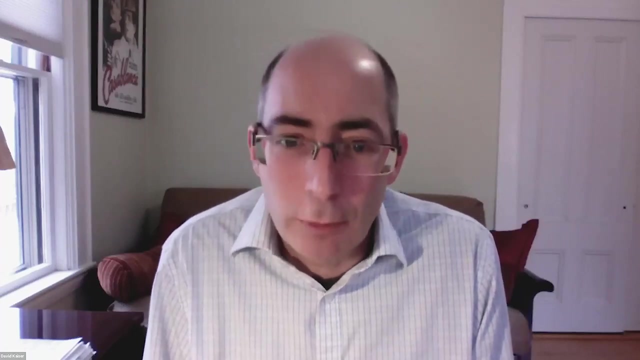 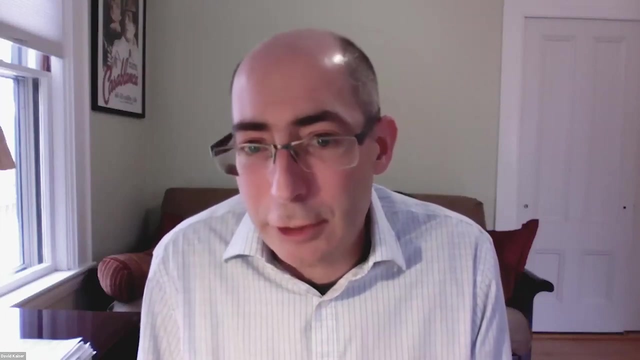 or three other parameters of our choice. And that's, I think, a well posed critique of this. like wiggle one parameter, find things do or don't work And, to be honest, I think a lot of the work so far has still been, understandably, to make it computationally tractable. understandably, it's still mostly been like wiggle one constant: what changes If the force of, if the value of the electric charge was slightly different? could you have stable hydrogen atoms, yes or no? Okay, well, if I tweak that and five other things, maybe I can again. 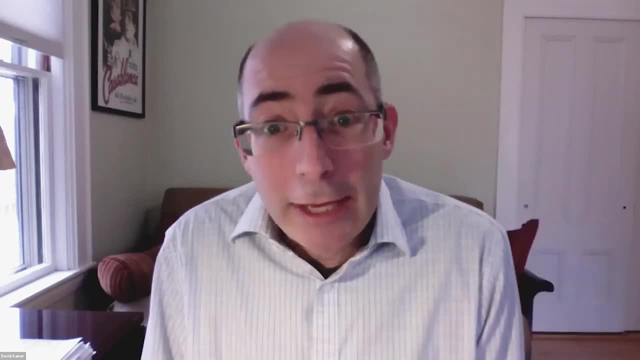 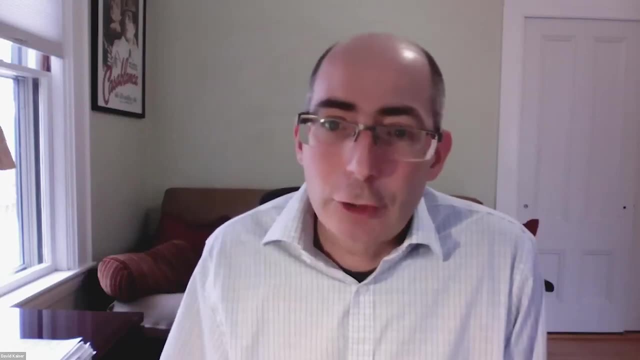 So the short answer, Alex, to your very well posed question is: I don't know- and frankly I don't think anyone knows- The way people have tried to pose that is in this somewhat kind of simplified or, let's say, tractable approach. but I agree, if we're honest about it, I think it's a wide open question. 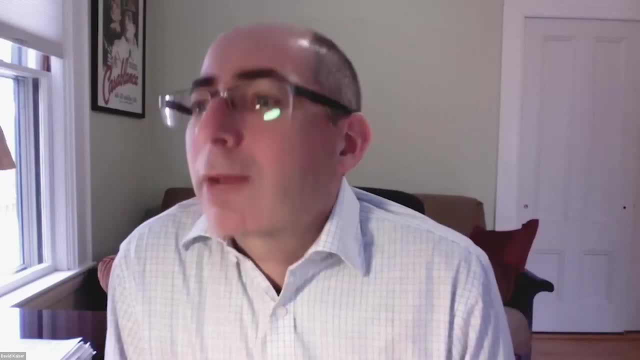 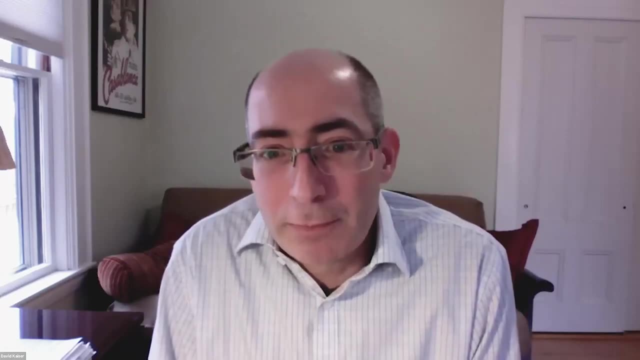 Kay asks: is there any connection between the anthropic principle and the quantum theory idea that quantum values don't exist until we choose to measure them? There could be connections. It's a great question, Kay, One of my co-authors. so now it's getting close to home. I've been tainted by all these crazy people. No, a very dear friend has actually published on a kind of quantum multiverse. What if the many worlds interpretation from quantum theory, which I think is kind of like what you're referring to here, Kay- what if the many worlds interpretation of quantum theory were actually realized in physically distinct but disjointed regions of space, like in the multiverse? 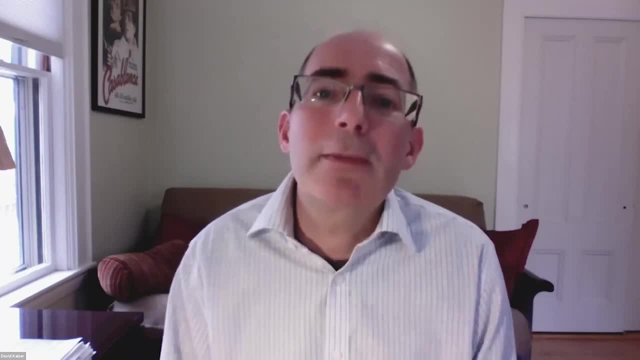 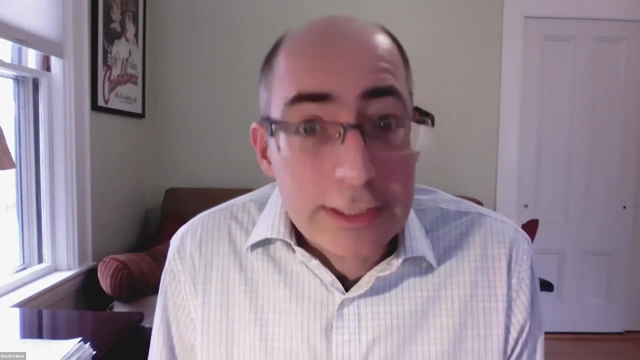 So one can at least try to pursue this question. It's not required, So typically these are actually separate sort of kinds of many worlds that people talk about And so typically they're kept kind of separate. But certainly conceptually one can try to build these self-consistent ideas and maybe even see if that leads to new predictions. 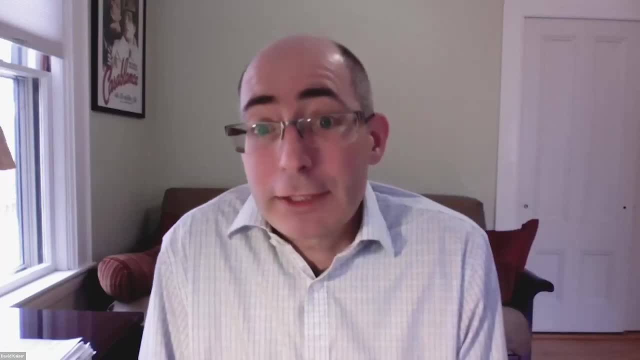 So far I haven't seen any, But one can try to see if these sets of ideas could even fit together in principle, let alone do they help explain one another. So, Kay, that's a great question. Some people do work very squarely on that. 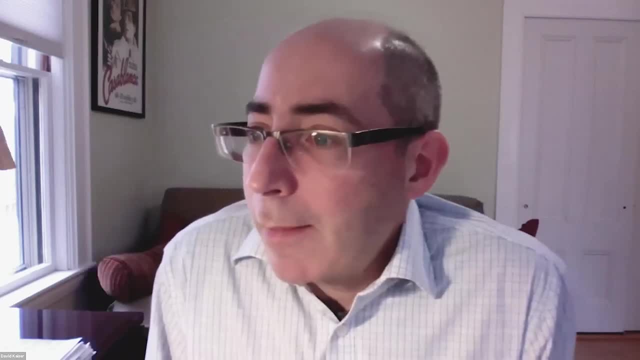 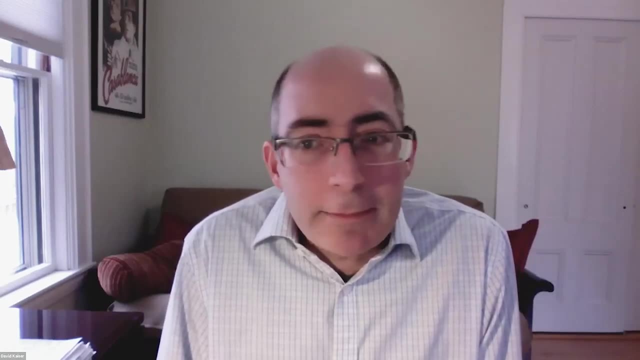 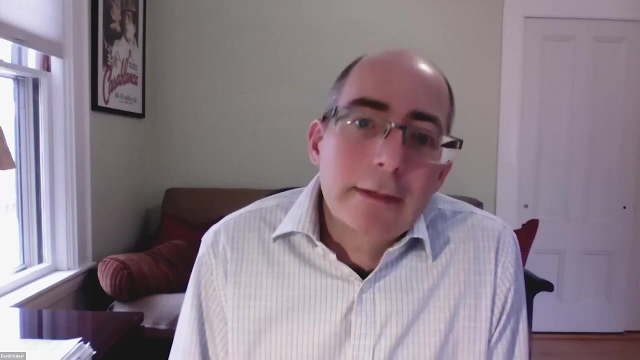 Fisher asks: since these extra dimensions are on the scale of the Planck length, I imagine there's no experiment we can perform to determine if they have any physical meaning. Good, So I should say the limits, empirically, are that these extra dimensions can't be larger than about millimeter scale, And millimeter is a lot bigger than the Planck length. There's no compelling reason why they should be millimeter scale and not larger right. So that would still take some explaining. But the kind of high precision tests of gravity. that's where these limits mostly come from, testing gravity in a kind of classical general altivistic framework. people have done pretty compelling experimental bounds saying there's no measurable departure down from like. 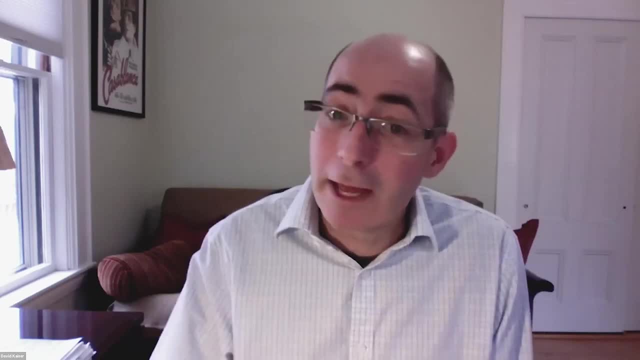 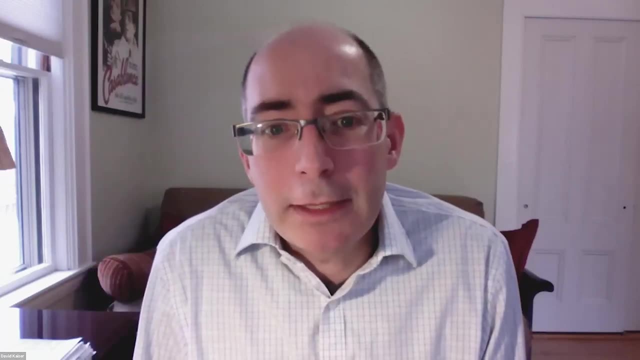 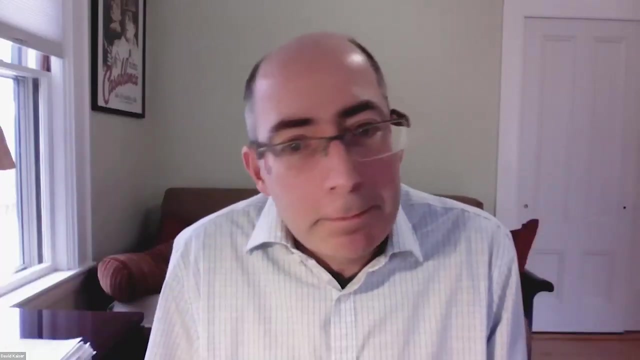 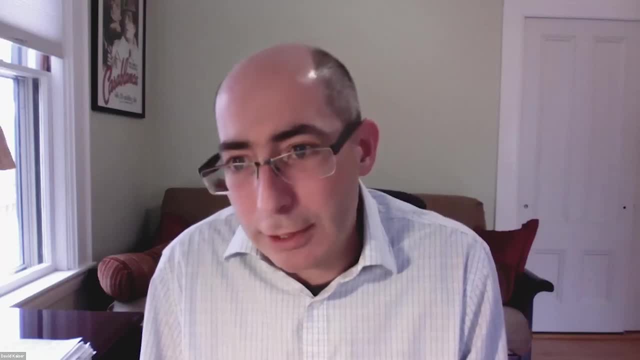 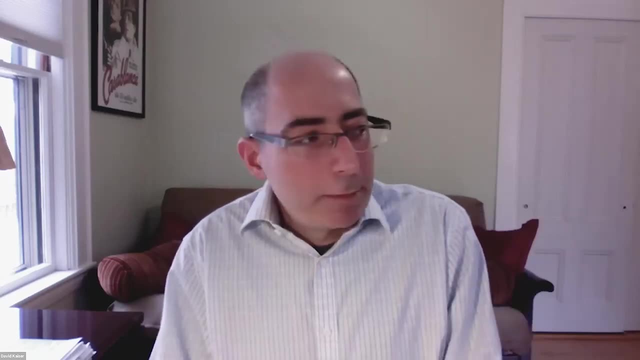 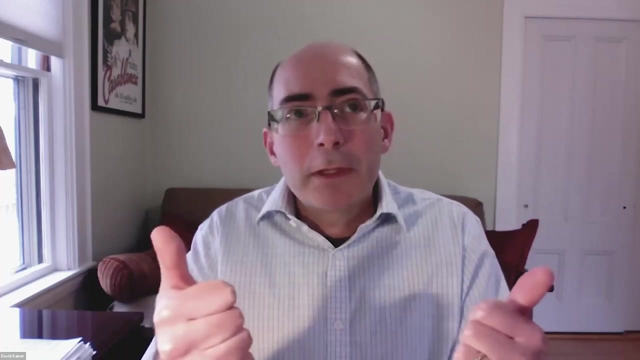 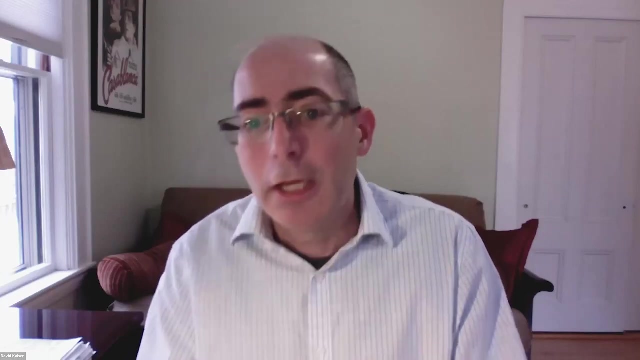 if these extra dimensions were small on human scale, but not so small is with something that's called missing momentum. It's different from the missing mass problem. So at very high energy, particle colliders like the Large Hadron Collider is there, could, are there way. is there basically momentum that goes missing in the otherwise very careful momentum conservation balance when you smash, for example, two protons together and collect all the junk that comes flying out. 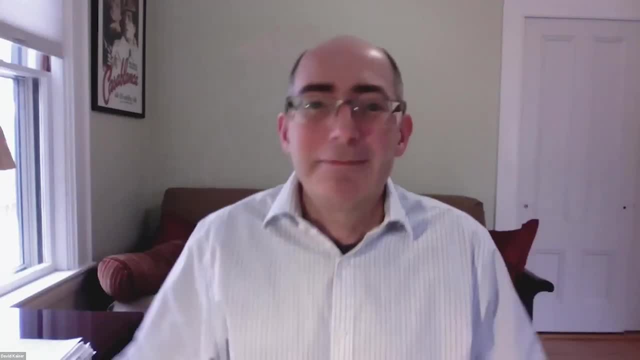 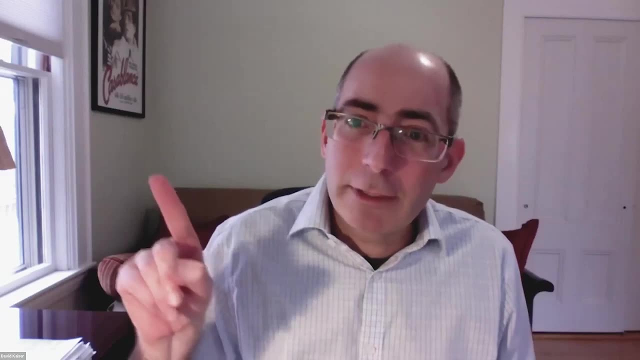 Every time they've done it so far, the momentum balances perfectly, Which is we should think like that's really great. That's great If there had been some of these particles in some sense taking some of their journey, taking a kind of detour. 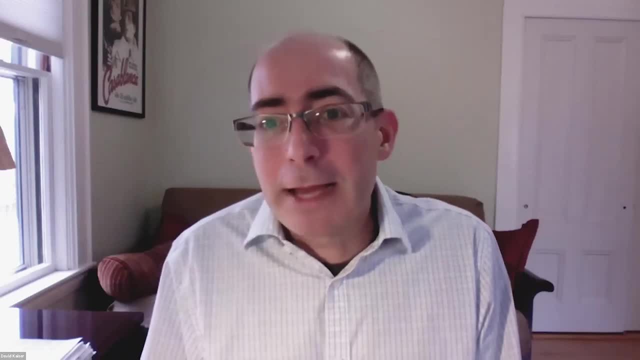 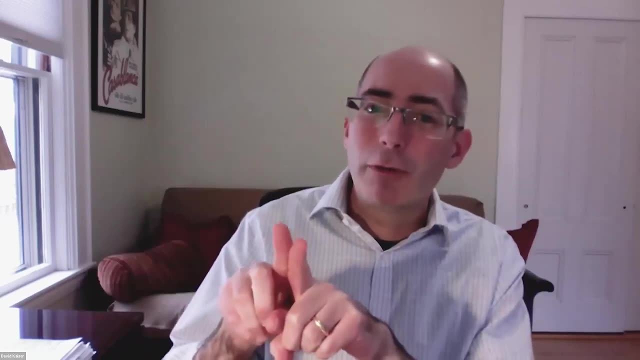 like a shortcut through some of these extra dimensions of space, then the momentum balance that we measure in our three dimensions should, in principle, be off, and maybe by a measurable amount, if, if those shortcuts were over long enough distances, like you know. 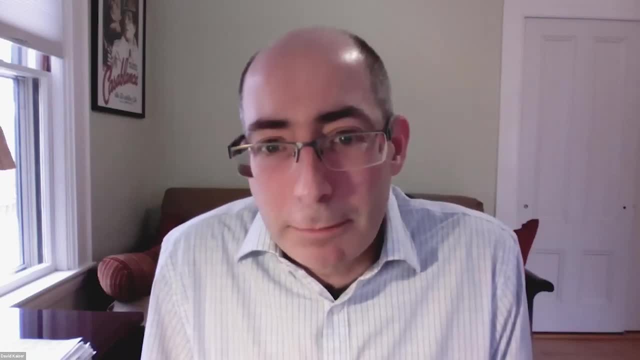 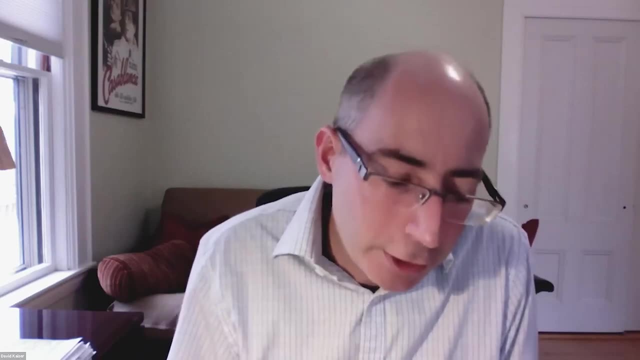 microns, not plot lengths. So there is a program to put to use particle collision data to put limits on on that version of a kind of shrunken down extra dimension. I should say I mentioned Lisa Randall's book Warped Passages. 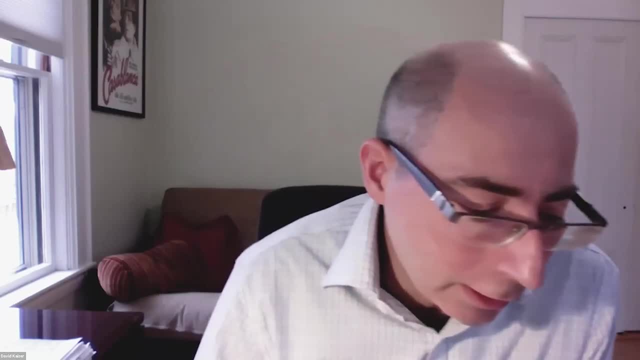 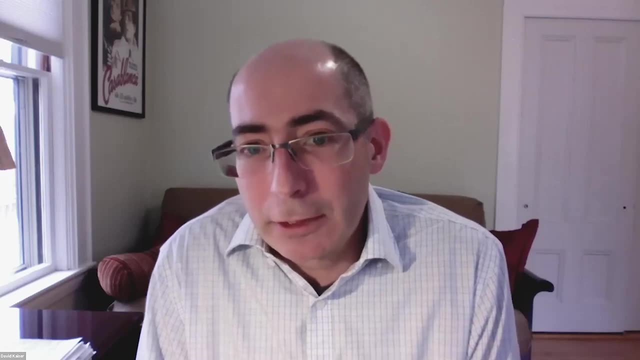 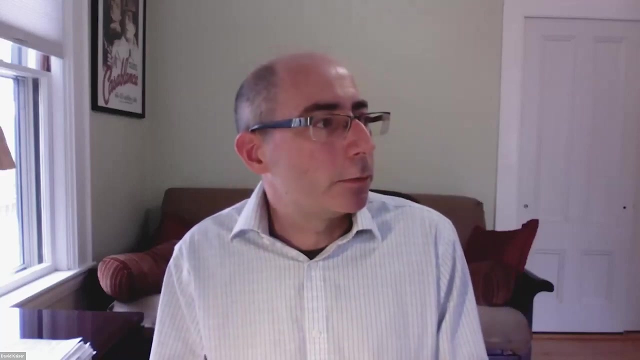 Lisa talks about one of her own very, very, very ingenious interventions was what if these extra dimensions actually never got small? What if they are still macroscopically large? What she found with a, with a colleague back in the late 1990s- and I did some work on these models, but really Lisa was the driving force- 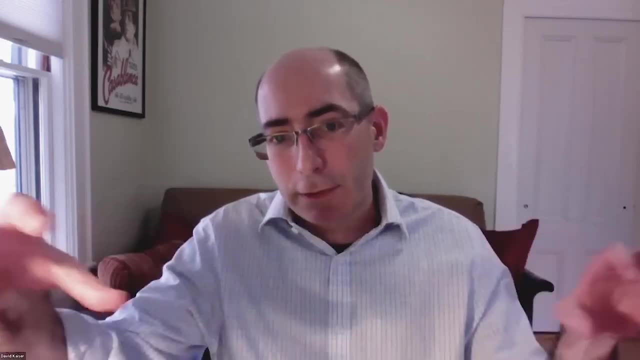 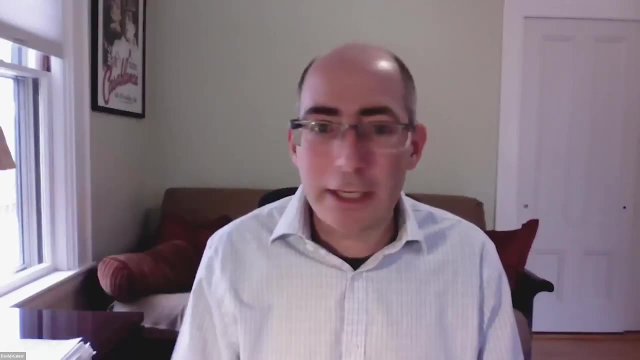 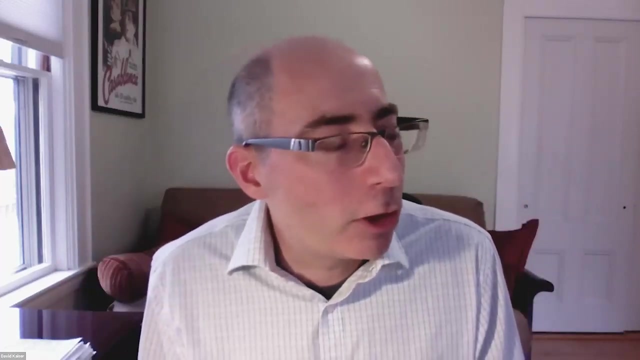 was. you could find self consistent gravitational configurations in which we would live on a three plus one dimensional slice And in fact quarks would stay stuck here. even gravity would appear to be stuck on this kind of sliver, self consistently You could have basically, it's almost like bound states for gravity to be. it's like an analogy to bound states. 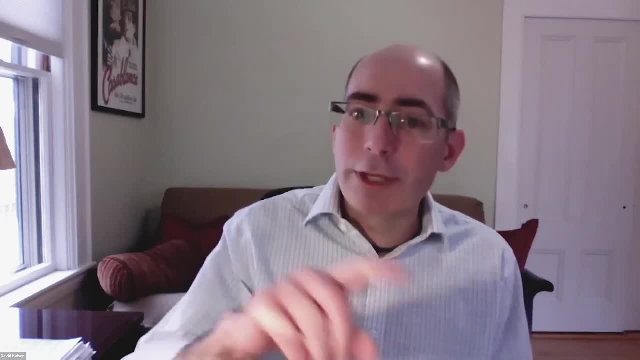 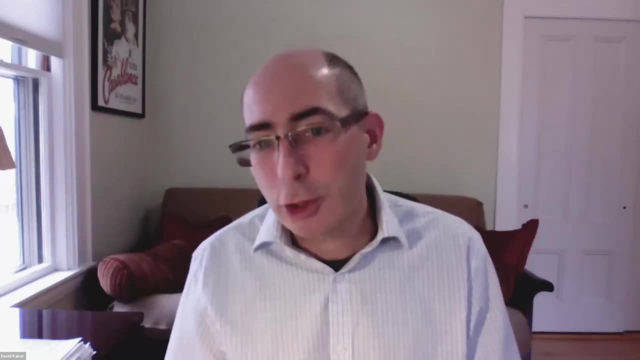 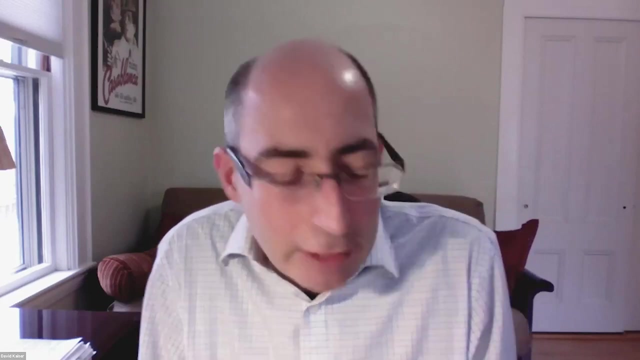 So the graviton might be exchanged, but might be exchanged only within a subspace. of all that are out there And you can, you could find again sort of simplified toy models in which gravity would behave that way, And Lisa Randall was really the pioneer for that back in starting in, I think, 97, 98.. 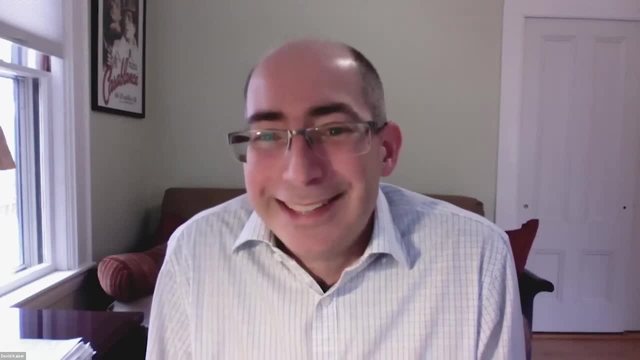 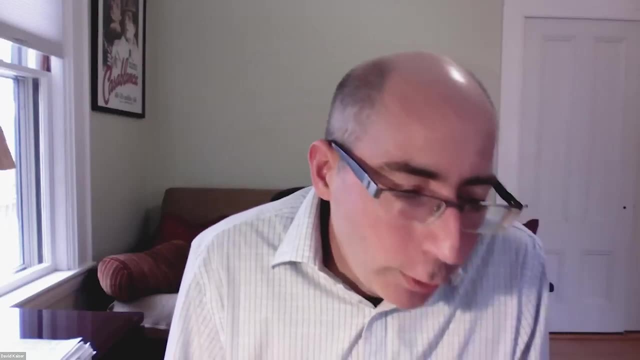 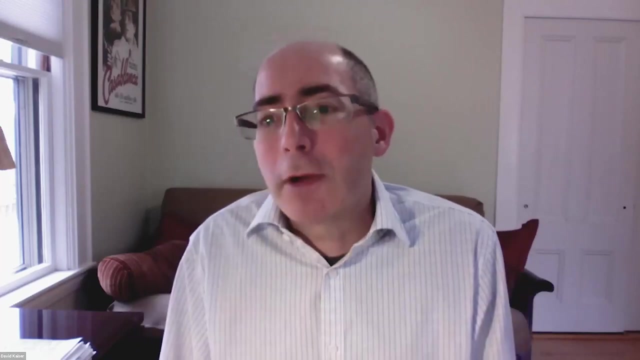 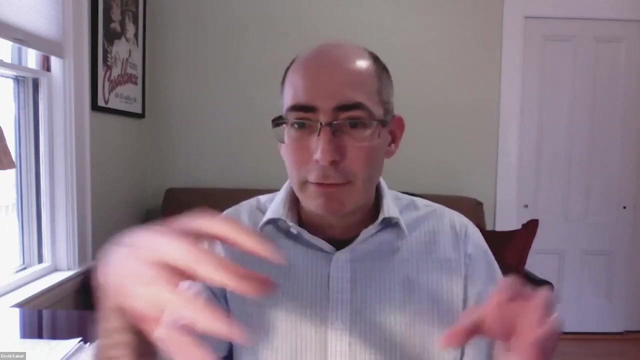 So there are other ideas around to try to live with at least conceptually large extra dimensions without having to curl them up. Now the challenge there was: could one find a model that has the symmetries that we actually observe in our universe, and not more? So those models work really very, very lovely if you have very, very highly symmetric spaces. for the ones that we would live on, that look either exactly like Minkowski space. 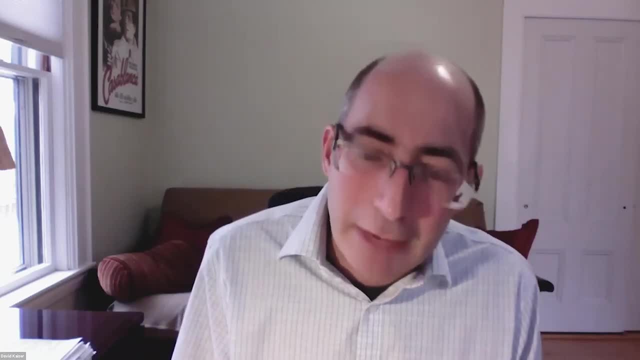 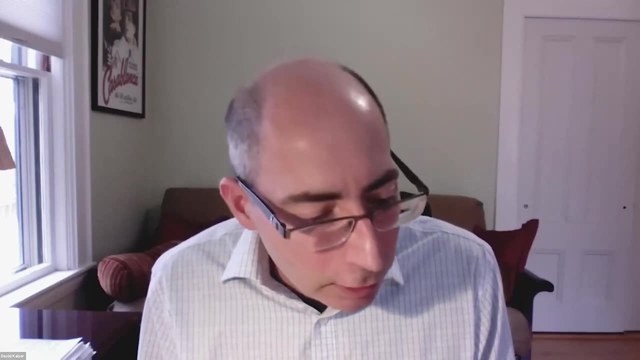 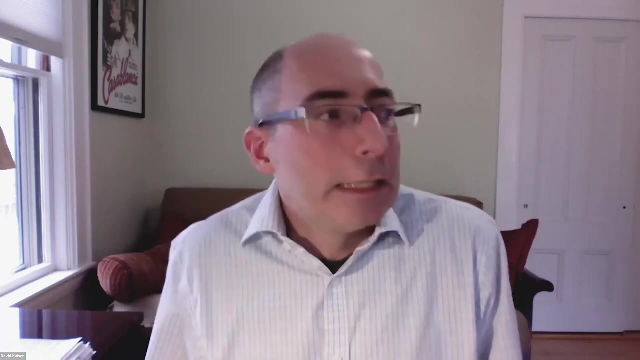 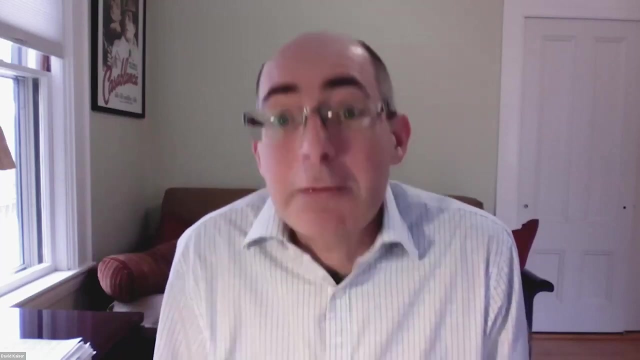 or something very similar. We live in a slightly less symmetric space time than Minkowski space, And it turns out there was at least no mathematically demonstrated way to embed even that simplified toy model with one fewer kind of symmetry group in that structure. that doesn't mean it couldn't be done, So that's an open question. but there are many ways to try to live with, make peace with many extra dimensions, but they all require, you know, a pretty big kind of leap. 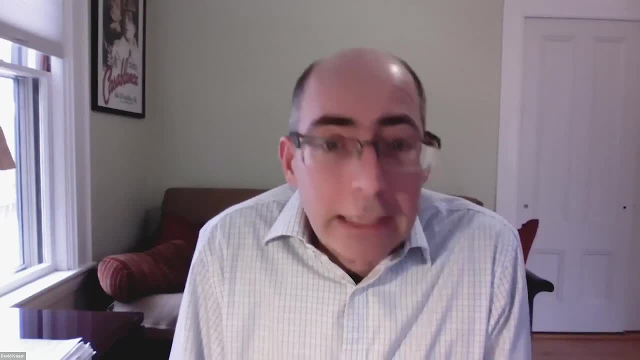 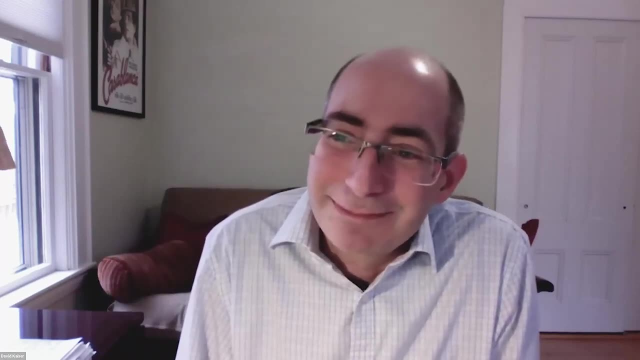 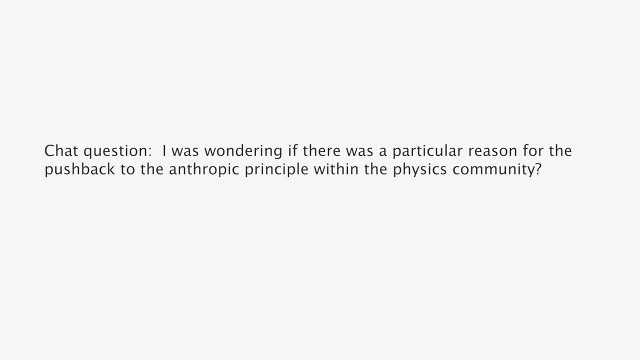 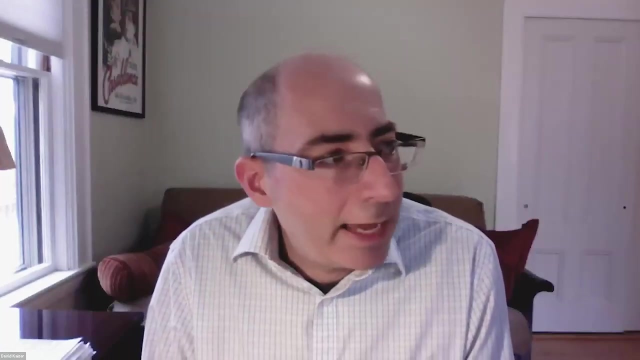 And none of them so far has been compelling, kind of forced on anyone, based on new kind of experimental observations or anything else. So it's still in the realm of the hypothetical. Good Other questions, You know, I think. I think part of it is that that really, at least to its critics- and frankly I'm sympathetic with this critical view- it seems to give up on the, on the aim of trying to explain the universe that we live in based on 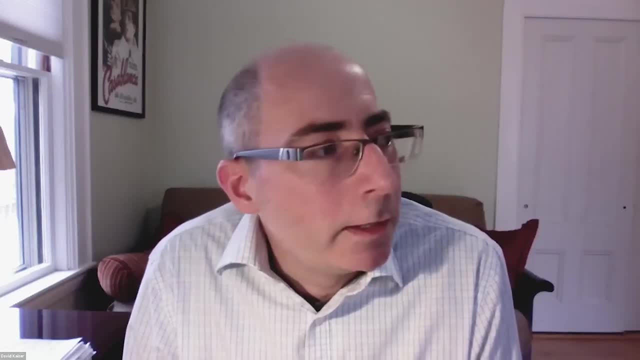 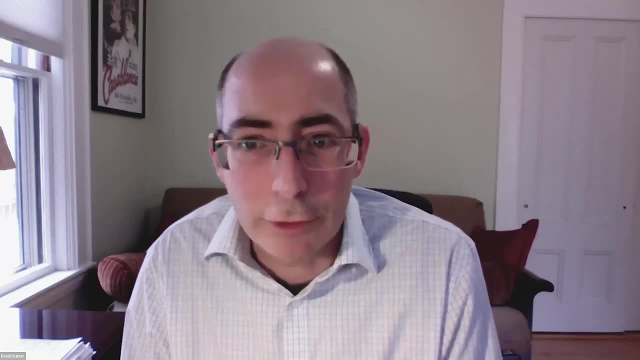 that is such an uns véhiculous way of perceiving the universe that exists, But there are some physical forces or laws that we could explain. It basically says that the universe that we live in is the outcome of basically random chance. It makes it more like the way we account for change in Darwinian natural selection. 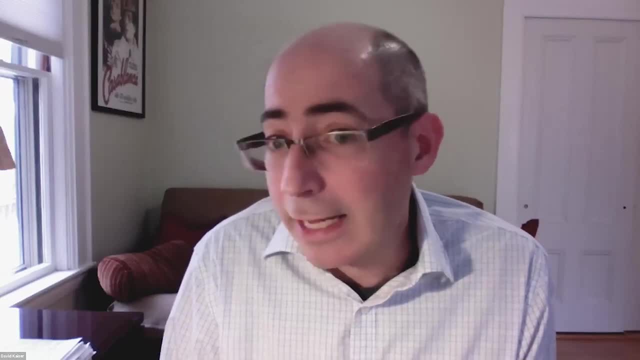 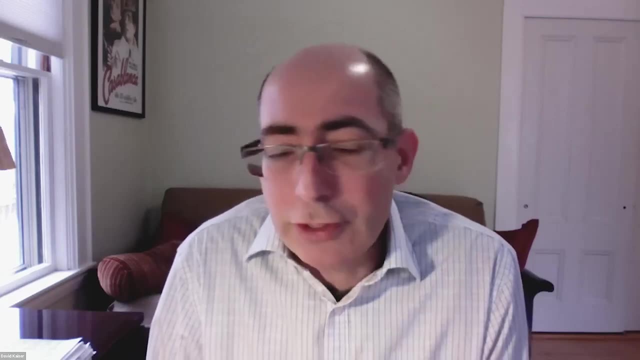 But now, with like infinities instead of just large numbers, It could just be random twists and turns of fate And maybe that's, maybe that is the right answer. But that kind of grates against a kind of aesthetic preference. It's not like it's a logical necessity, but it grates against a kind of form. 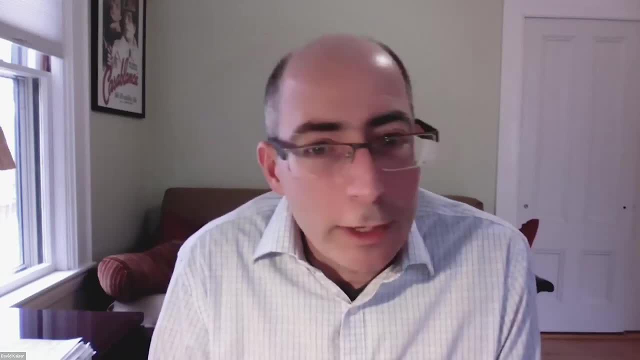 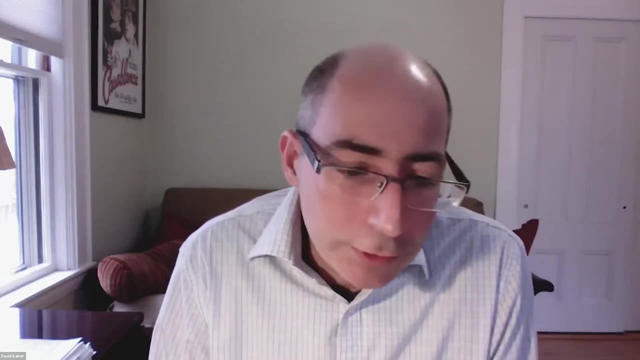 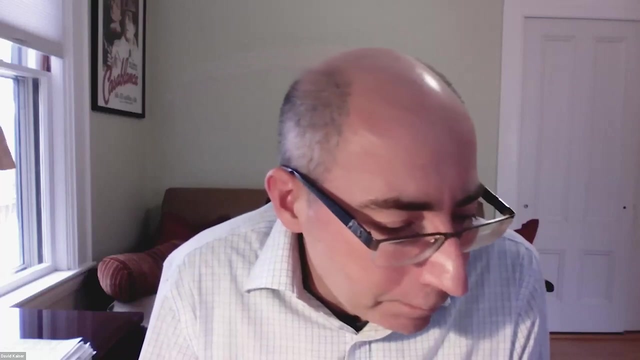 of explanation that has, I think, otherwise been successful as a goal, Let's say aspirational, for things from Newton's day through Lisa, Randall's day for that matter, for efforts to try to account for a specific set of, let's say, fundamental forces acting on a specific set of. 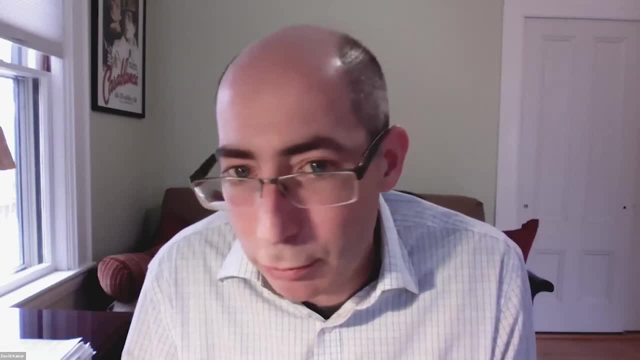 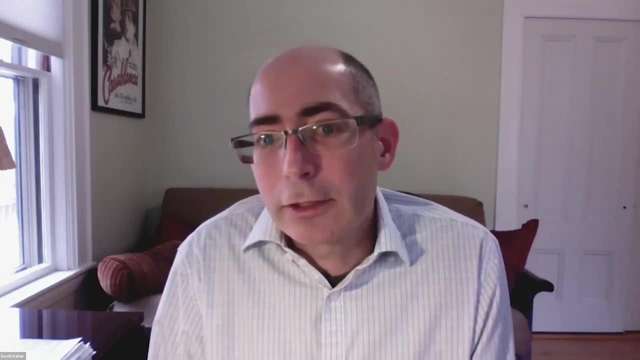 elementary constituents, whether they're quarks and gluons or superstrings or name your favorite, and being able to account for bulk properties that we could compare with observations, And I think, the thing that sticks in the cross, so to speak, for critics of the anthropic principle. 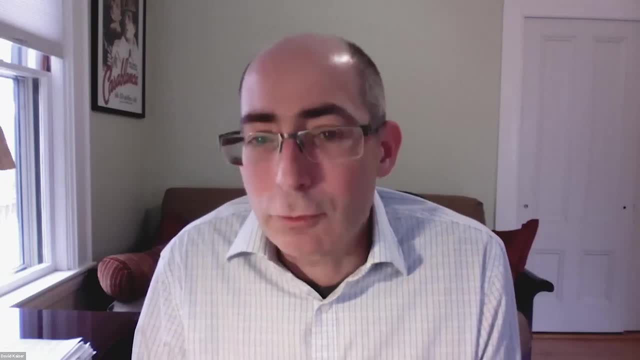 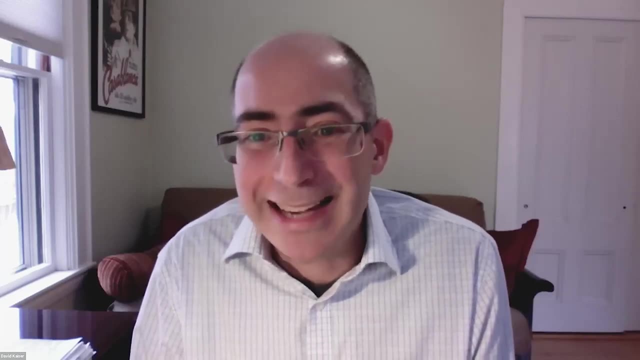 is that at the end of the day, people have to say: just random chance, and there's no kind of deeper explanation for why we measure the things we do And they not only could be different, they actually might be different and maybe even are different, infinitely different ways. 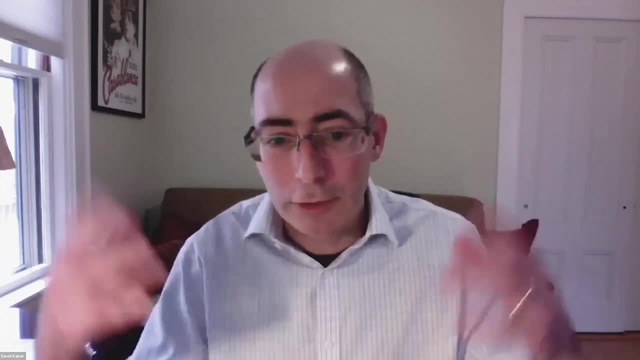 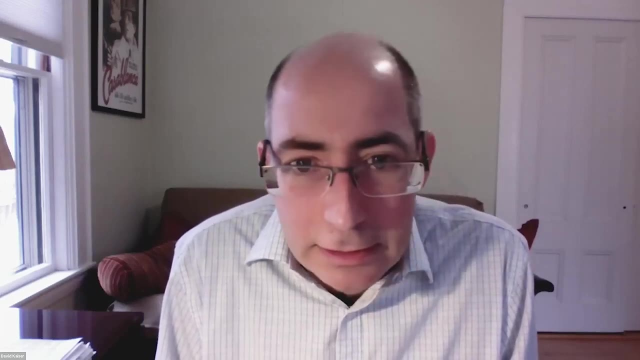 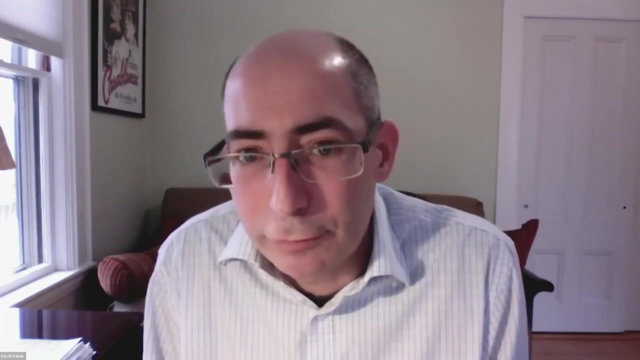 out. So it's changing, so to speak, the explanatory goals. That doesn't mean it's not that it's logically internally inconsistent. It's a different kind of aspiration or aesthetic choice or philosophical aim for what one thinks the nature of explanation should be in an area of. 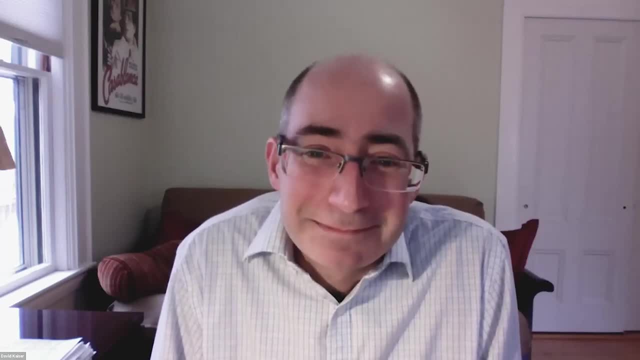 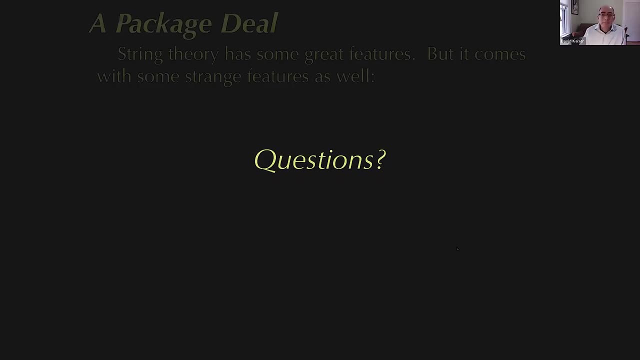 science like physics, And they might be right. Let me press on for this last part Much quicker. So I mentioned that string theory has some great features, at least features that got people excited. We could make sense of those bursts of enthusiasm on the publication pattern. But 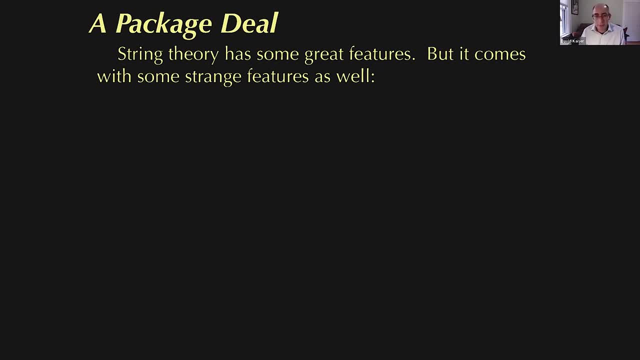 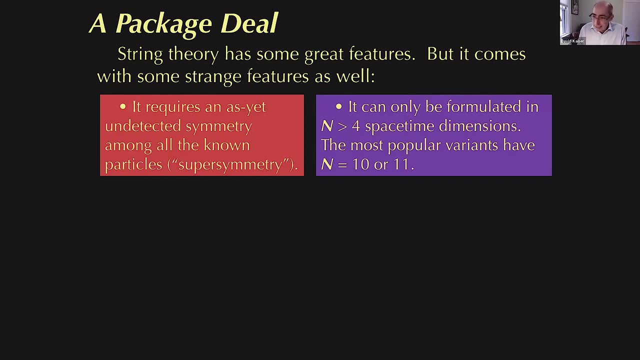 actually I borrow the term package deal from Lee Smolin, one of his books I mentioned earlier. It's like when you want to go buy a used car off the lot, you don't get to choose exactly which features you want. And so again, Lee Smolin uses this analogy. 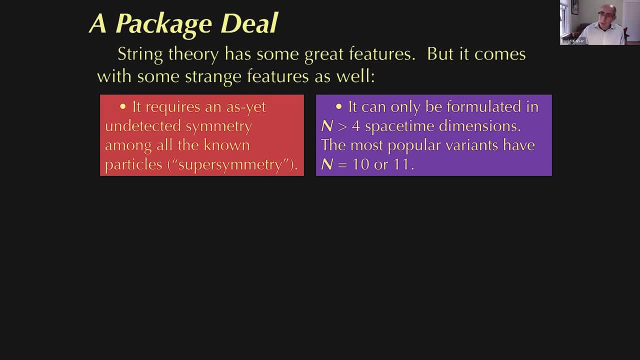 It's like what if the car you really love, this one on the used car lot, has just the right kind of transmission you're looking for, but not the stereo system you want, or vice versa You have to. it's like a package deal. 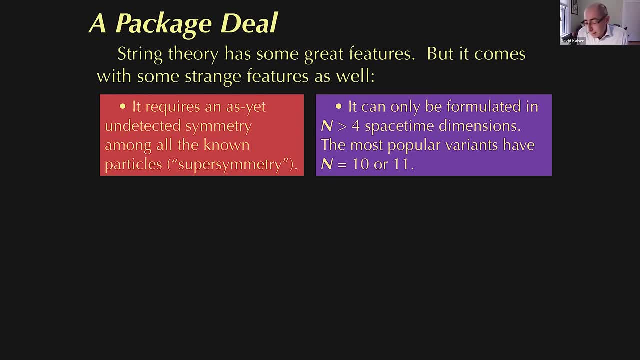 And so string theory has many features like it includes massless spin to graviton. it seems like it could avoid some of these infinities from quantum electronomics, and yet it can only be formulated self consistently with these as yet undetected symmetries. 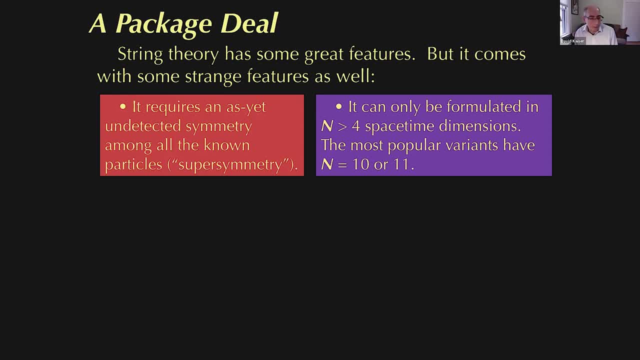 So these super symmetry doubling every known particle in the universe and also many extra dimensions, And so people, critics like Lee Smolin, have said, you know, are the things we don't want starting to outweigh the things that we do want? Is this a good deal in this package deal? 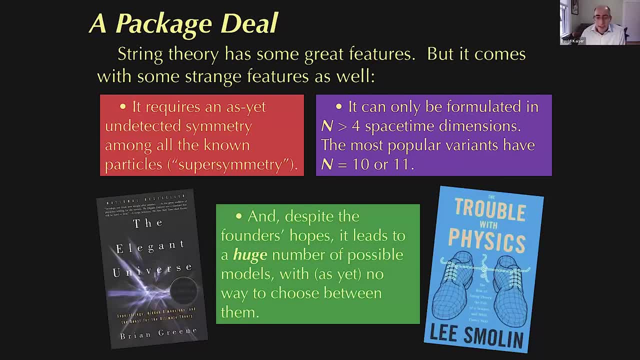 And so again for your reading list. these are now kind of classic books. Brian Green's book came out first in 1999.. Brian has been for a long time one of the most, I'd say, eloquent proponents of the string theory. 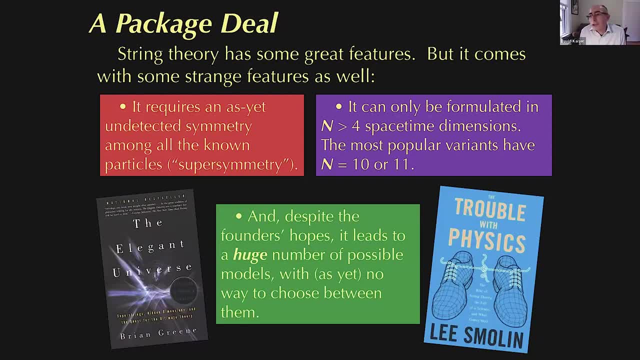 And I know it's hard to see People think that he was talking about something that was like a counterbalance to the theory that he was talking about. And so again for your reading list, these are now kind of classic books. Brian Green's book came out first in 1999.. Brian has been for a long time one of the most, I'd say, eloquent proponents of the string theory. 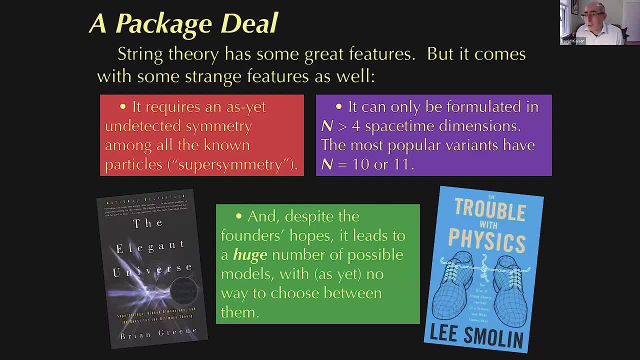 theory, super string theory approach, And this book was a finalist for the Pulitzer Prize. It's a beautifully written book, very accessible And then again a very clear book by one of these now outsmoking critics, Lee Smolin. This one came out in around 2005 or 2006, called The Trouble. 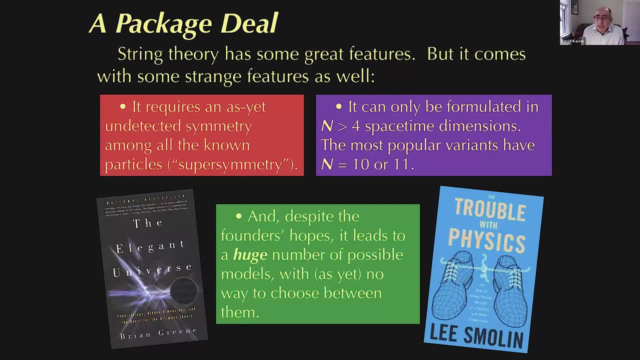 with Physics And I think these two together give you a pretty nice range of again what the stakes are in these so-called string wars. What are the hopes that got people like Brian and so many people excited And what's the kind of cold water? What are the cautions that some critics like Lee Smolin 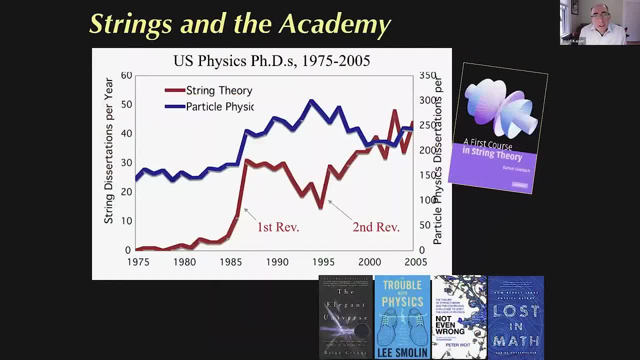 put on the table as well. Those are two you might enjoy. Let's go back to counting things. As I tried to indicate- and we've seen many times in our course together- these kind of rivalries or debates are not happening in a vacuum. They're not happening in a string vacuum, not even happening. 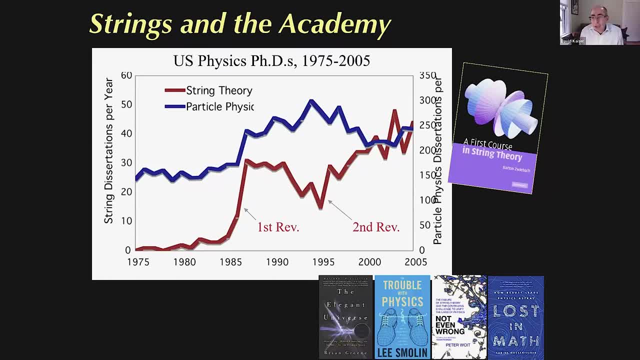 in a macroscopic vacuum. So let's go back and ask about what else has been going on that might help nudge or push and pull the state of discussion among, let's say, high-energy physics, especially, but not only, in the United States in recent decades. So here is. 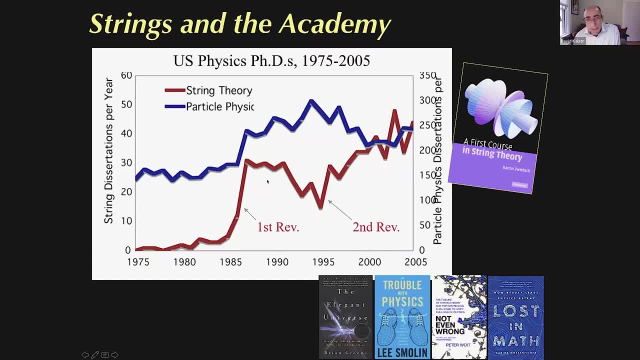 another thing I like to count. The blue is all with this axis. here are all the PhDs per year in the US on any area of high-energy theory, high-energy physics, including experiment, all high-energy physics, particle physics, And the red is once again dissertations, now on string. 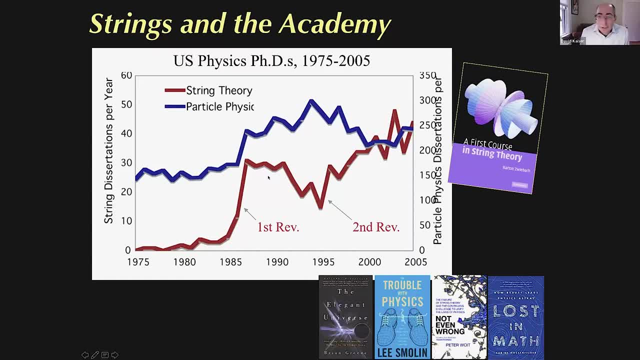 theory It looks a lot like the curve of publications, not surprisingly So. again, you see a very different set of patterns of when you have a kind of growing number of people in particle physics broadly and then going into a decline, a pretty clear trend line there. 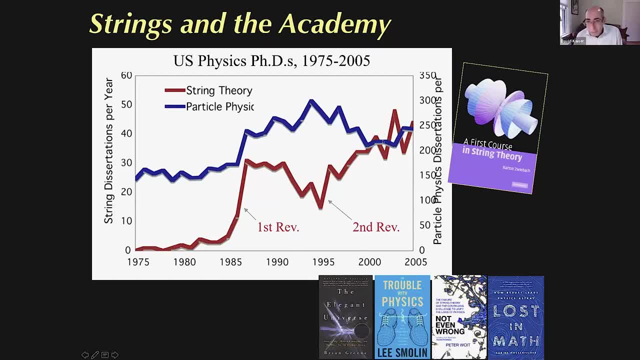 starting in the early to mid-1990s. Meanwhile a very steep climb, a kind of almost runaway growth on the attention to string theory and they're kind of out of phase. Overall particle physics starts to decline while string theory starts another one of these large periods of rise. 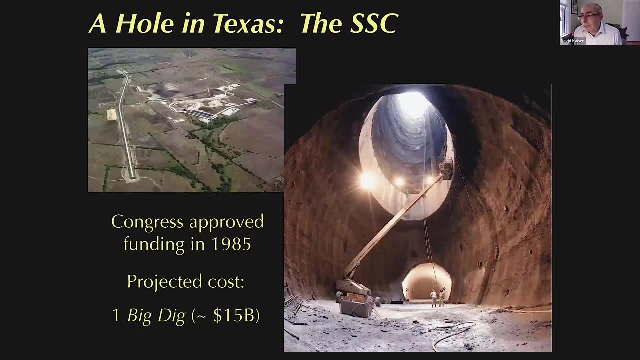 Well, that's not happening alone. One of the things that happens right around that pivot point is something that I never stop talking about. It was the cancellation of an enormous project called the Superconducting Supercollider, or SSC. This was a project approved in the US in 1985.. It was under construction outside of Dallas. 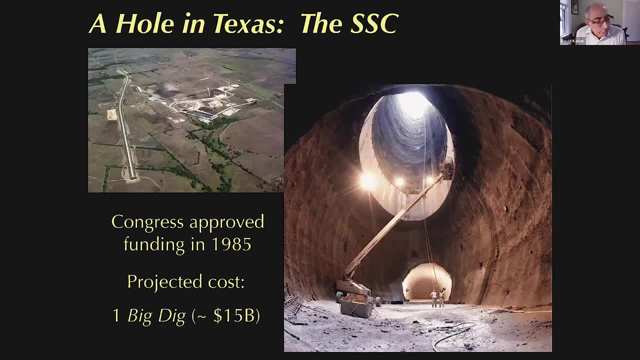 Texas, in a tiny town called Waxahachie, Texas, not too far from Dallas. It was actually going to be three times larger than the Large Hadron Collider, which at that point had not yet been built. So it would have been- let's see- a 52-mile circumference or 50-mile circumference. 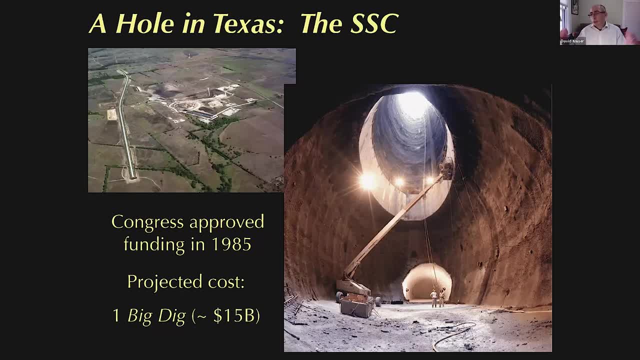 24-mile circumference ring to accelerate protons and smash them together with correspondingly three times larger interaction energies. The argument was that people could have hopefully found things like the Higgs boson, maybe evidence of supersymmetry, in the 80s and 90s. 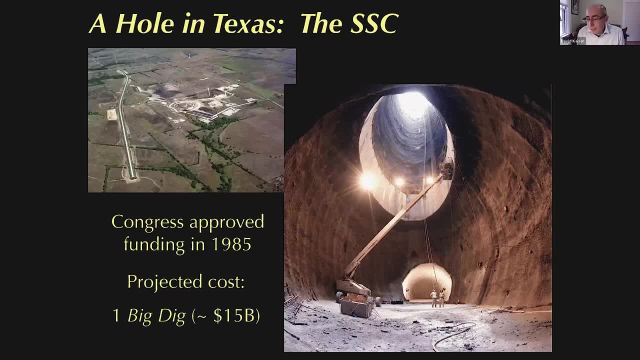 The problem was this was, as you might expect, unbelievably expensive. They actually wound up excavating almost the entire tunnel, many, many, many hundreds of feet underground. They had not finished installing the superconducting magnets and all the rest. 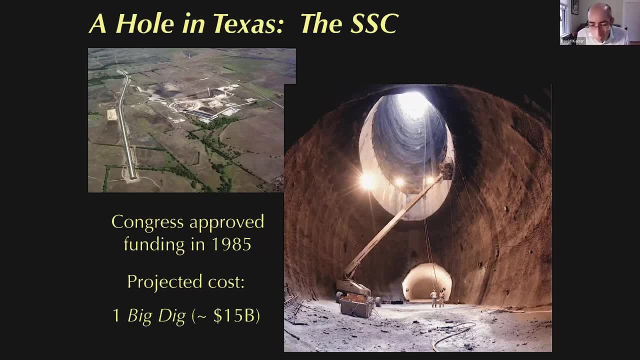 The cost was growing very quickly. It was approved with a budget of a couple billion dollars. By the time the project was canceled, the budget had ballooned to $15 billion. That's now on a US appropriations budget. that's a lot of money. That kind of budget now conflicts with. 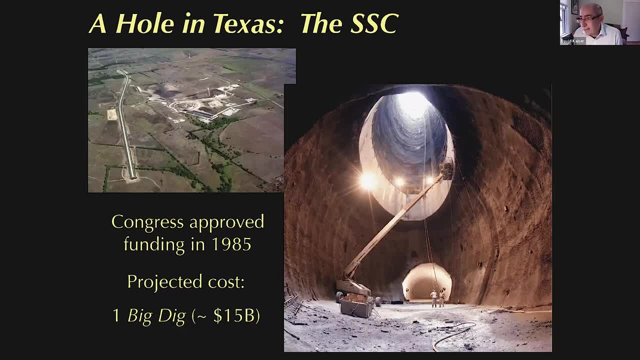 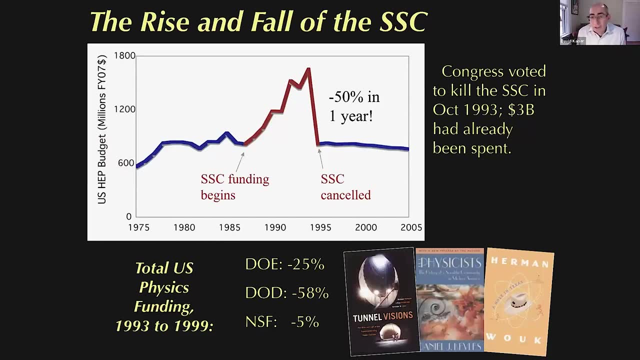 things like military expenditures, not basic science expenditures. So this project was heading for a collision And in fact, after many fits and starts, the Congress canceled the SSC with one fateful vote in October of 1993.. I remember the date very well because I 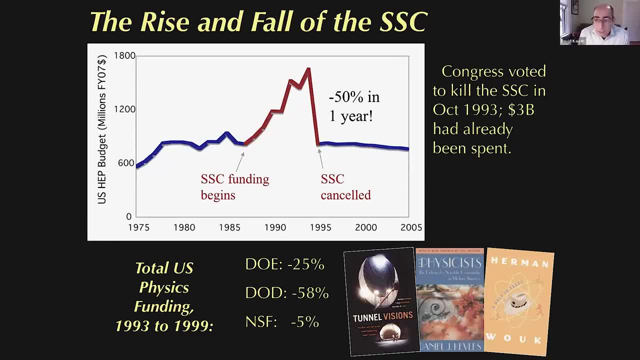 entered graduate school in September of 1993.. So I don't take it personally, but the US Congress killed off one of the reasons I went to grad school one month after I entered graduate school. I don't think they had me in mind. So you can see here. look at US funding for energy physics in. 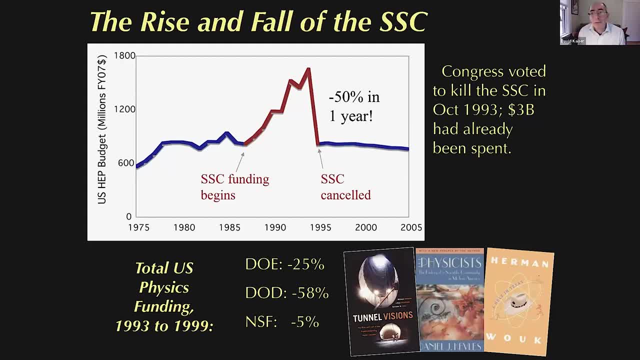 inflation-adjusted or constant dollars. Funding for the entire field, not just for that one experiment, for the entire field of energy physics fell in half in one year. That was an even sharper fall than the otherwise sharp falls we looked at many times in this class. 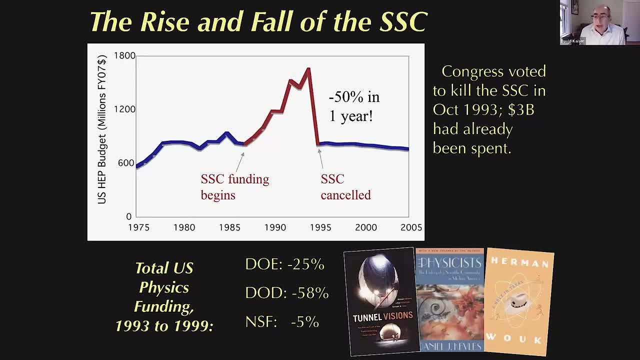 in the early 1970s. In the early 70s, the funding for energy physics fell in half over the span of four years. This time, Congress was even more efficient and canceled or reduced the budget for energy physics in half in literally one year And over the rest of the 90s after that. 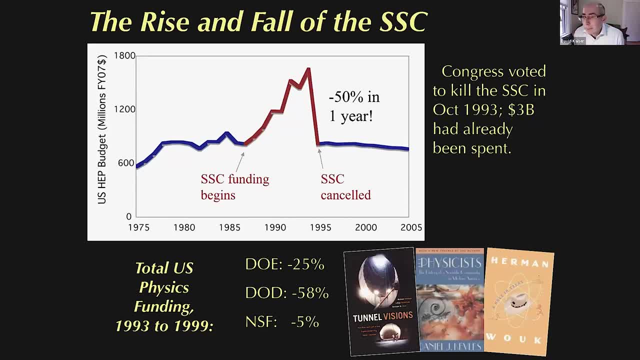 funding for physics across the board continued to lose ground, both because of budget cuts and because of inflation. Many, many books that have looked at the troubled history of the SSC in particular. there was even a novel about this by the novelist Herman Woke. He's the same novelist. 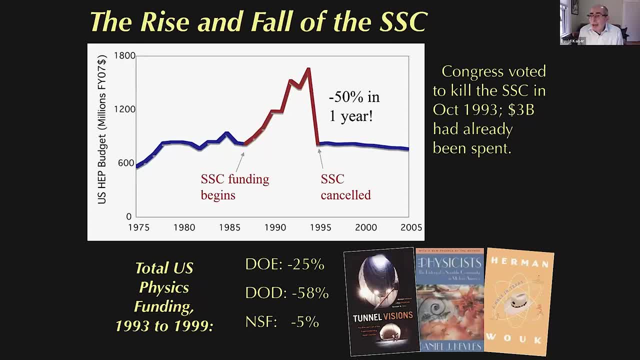 who wrote the Kane Mutiny. a very accomplished novelist wrote a novel about physicists in Texas watching the SSC get canceled. I took it to heart. Why did Congress cancel funding? In short, the Cold War had ended. There's many moving parts, but the overwhelming cause seems to have been 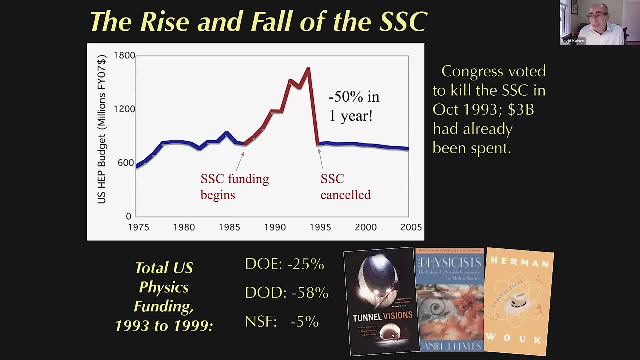 as many of these scholars have agreed, that the kind of reason to keep funding very large amounts of money on so-called basic research in areas like energy physics had always been a competition with the Soviets and the idea that if outright warfare broke out, you'd have all these well-trained people with good equipment. And after the Soviet Union dissolved, 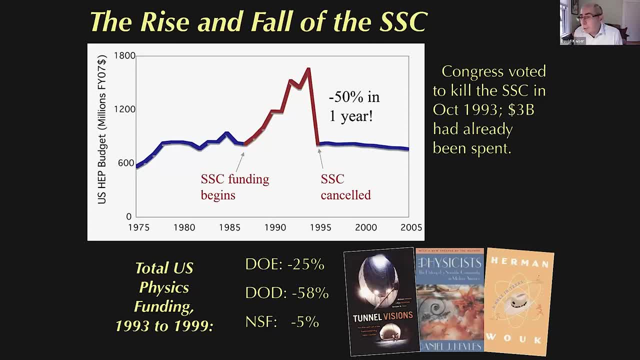 in summer of 1991, those arguments no longer held the same kind of sway that they had for generations before, And one of the most visible symbols of the end of the Cold War for science funding in the US was this idea that the Soviet Union was going to have to pay for the energy. 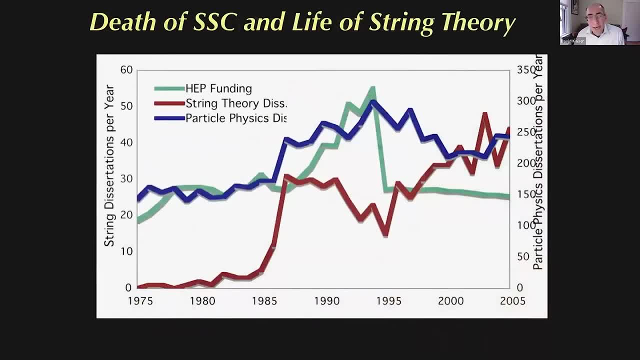 consumption of the world, And that was the cancellation of the huge accelerator. Let's go back to that plot of remember. this is now all PhDs in particle physics, PhDs in the US, strictly on string theory, And here because green means money. 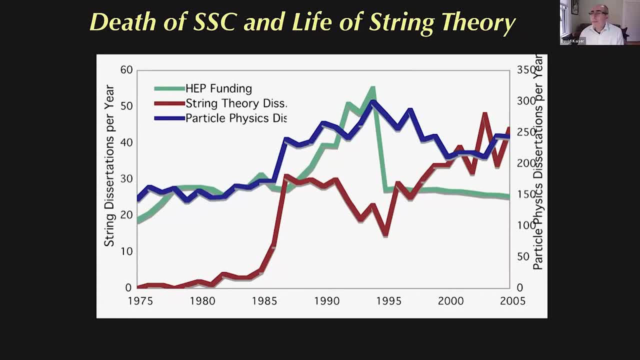 green is now that budget curve I just showed in the last plot- Look at the amazing correlations here- that you stop getting more people entering particle physics when funding falls in half Meanwhile, meaning you don't replenish the people who graduate, So people graduate here. 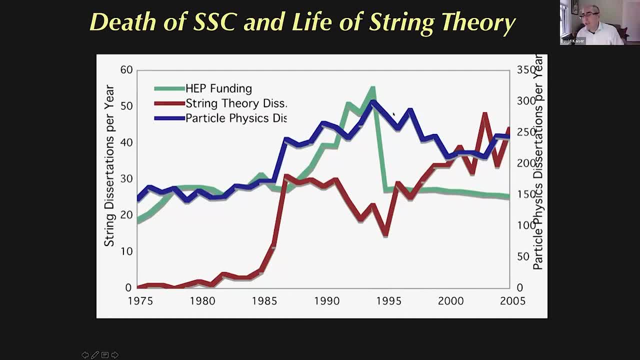 but not as many people enter afterwards, You start seeing the kind of characteristic five-year timescale fall-off that we can at least correlate with this very dramatic change in funding for the larger field. Meanwhile, string theory costs approximately pencils and espresso, well, and health insurance, all of which are important, none of which cost $15 billion for. 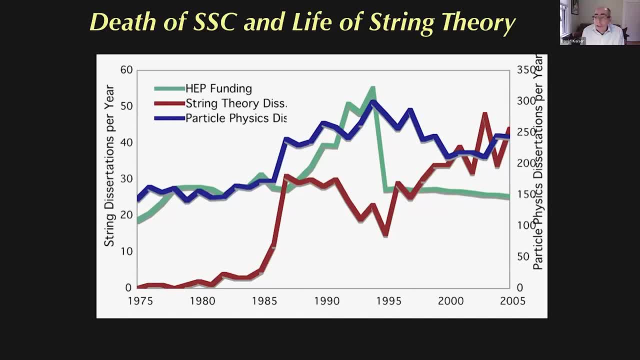 atom smasher. So dissertations on string theory start growing exponentially just at the moment when other trends within the subfield are looking less and less fiscally viable. It's not only the US. This is a complicated plot. It's a complicated plot. It's a complicated plot. It's a complicated. 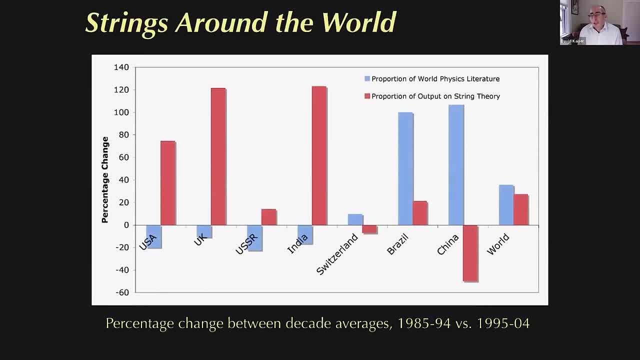 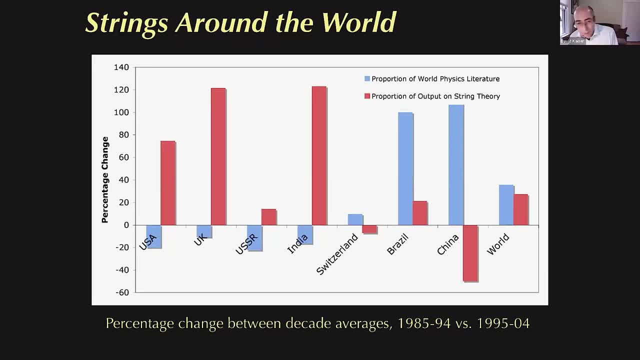 world, where the blue curve shows the change between the decade of the mid-80s to mid-90s, the change of that decade compared to the next decade, 90s to mid-2000s, the change in proportion of the world. physics literature. 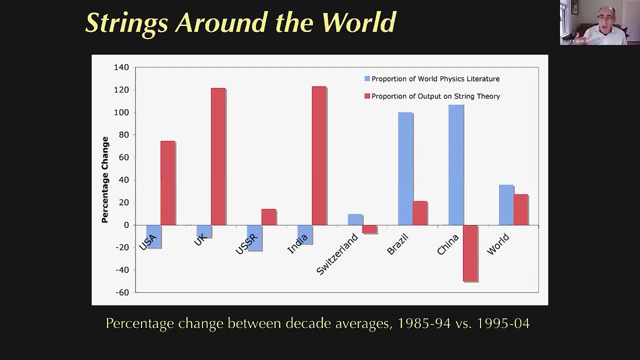 That's a very close proxy for budgets. Other people looked at this more carefully So you can really think of this as kind of budget trends. You can see the budget for physics research across the board fell in the United States after the end of the Cold War. That's consistent with what I 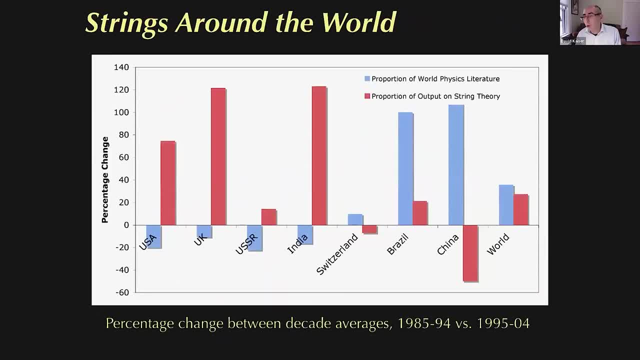 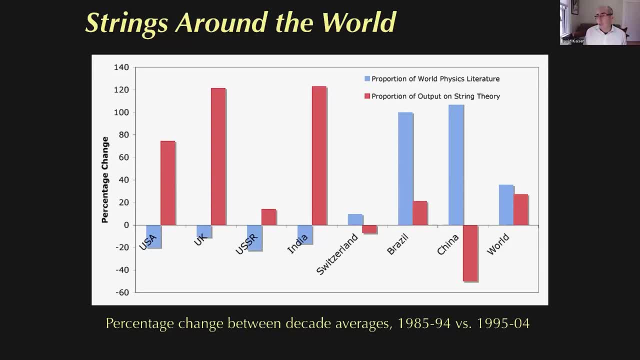 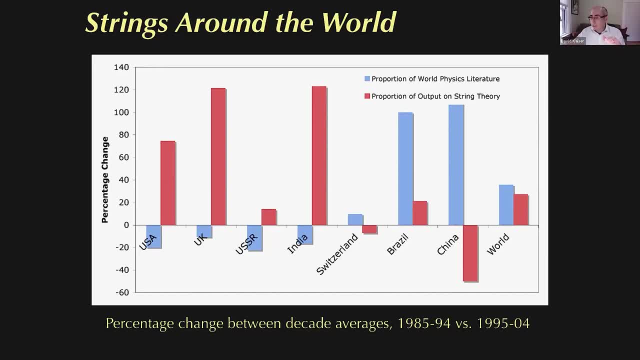 in physics overall and the proportion of physicists there who began working on string theory, versus the inverse countries that were investing across the board, more and more aggressively, across the full range of physics, And you see either a slower growing proportion or a falter proportion of the world physics literature. So it's a very close proxy for budgets. 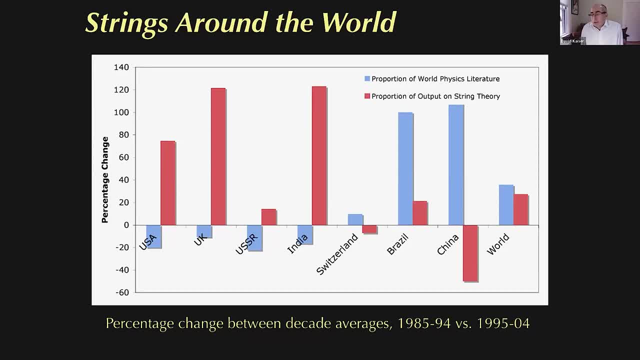 a falling proportion of physicists working on string theory. That doesn't mean there's no reason to work on string theory intellectually. It does remind us that these decisions are not happening in a vacuum, that what are the resources available with which to even ask certain questions? 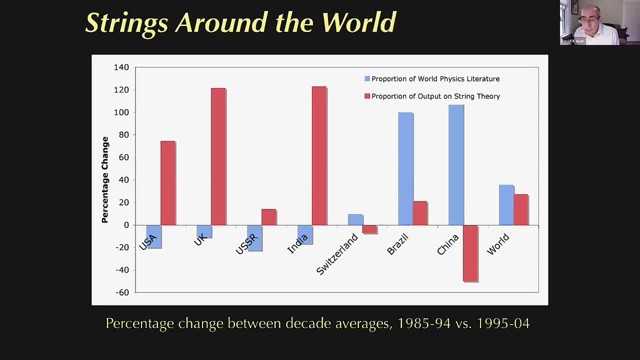 Those change not only based on arguments about string compactifications or eternal inflation. Physics, then, is now still embedded in a pretty messy world, a world that, in this case, went through a pretty dramatic change with the end of the Cold War. So let me wrap up Early in our own. 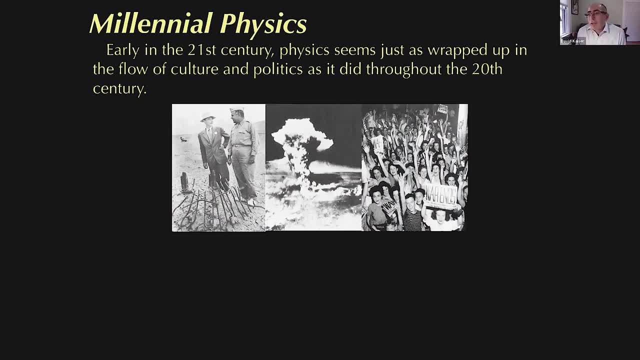 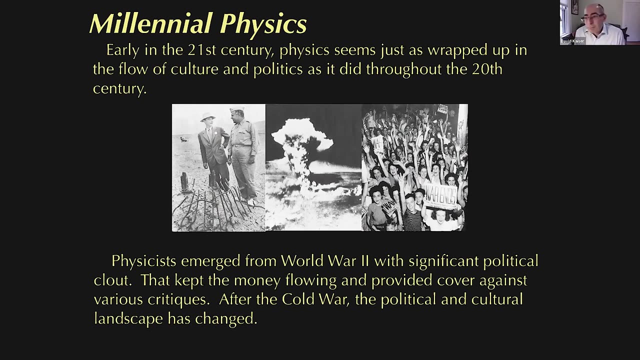 millennium physics seems to be just as much in the flow embedded in the world of people, culture, politics, geopolitics and budgets and all the rest, as it has been throughout the whole period we've looked at this semester. We saw for a good chunk of the term. there was a moment in 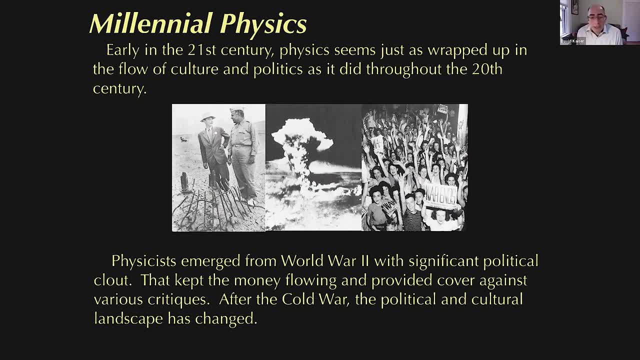 the middle decades of the 20th century, largely coming out of the wartime projects, when physics, especially in the US, seemed to have a kind of unlimited range of resources and a command of respect and so on, as well as heightened scrutiny with McCarthyism and all the rest. It was center. 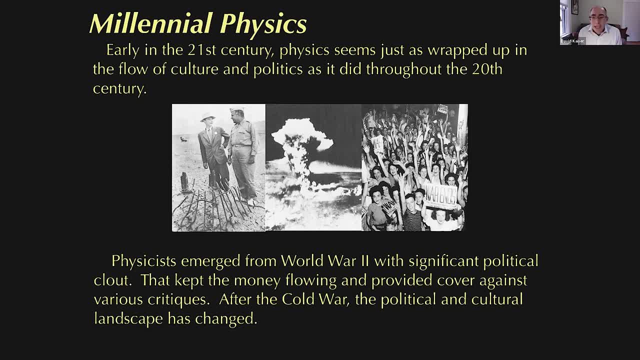 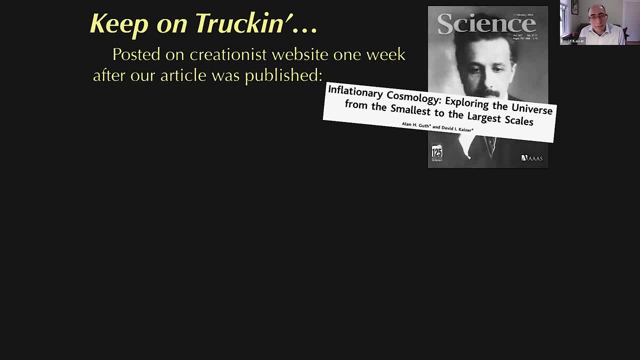 course, a couple of years ago- this was about 15 years ago- Alan and I had written a very brief review article on inflation. In fact it was one of the readings for the previous class. It was published in Science. One week later there was a point-by-point rebuttal posted on a creationist.